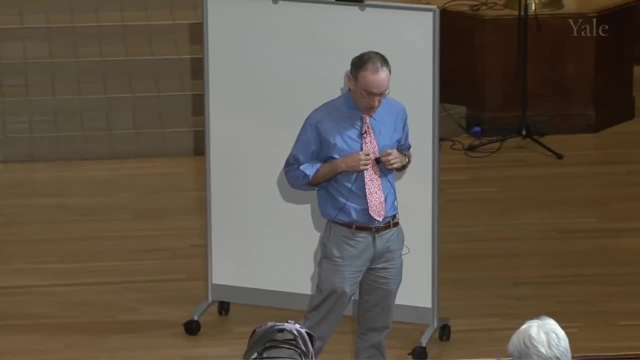 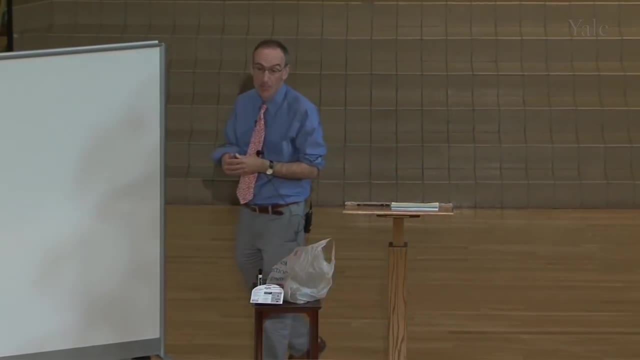 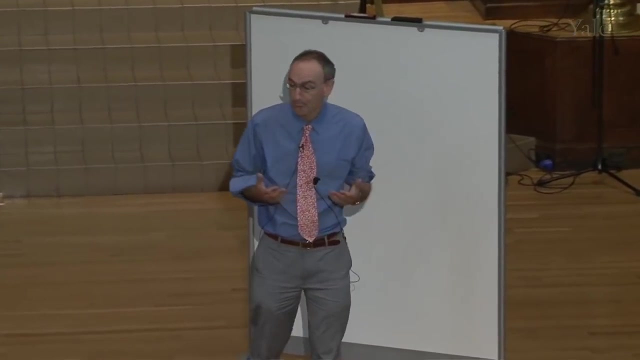 strategic situations. So what are strategic situations? Strategic situations are any setting where the things that you care about, the outcomes that you care about, the things that you care about, depend not just on your own actions, but on the actions of someone else. 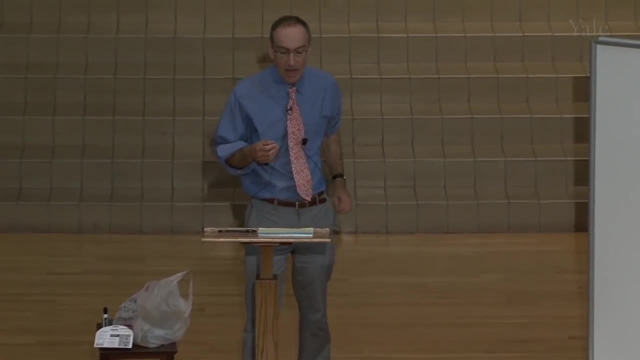 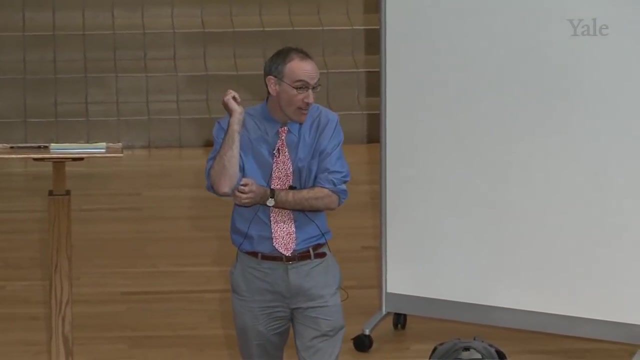 So let's think of some examples, but we won't stay long with examples. In economics, an obvious example would be two firms who are competing in the same marketplace. So think of Apple and Google, or Apple and Samsung. They're both competing in the market to make. 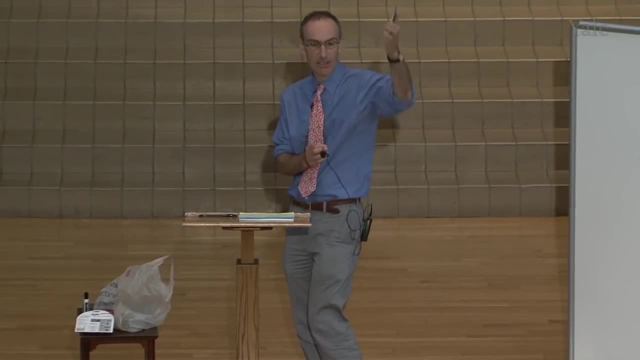 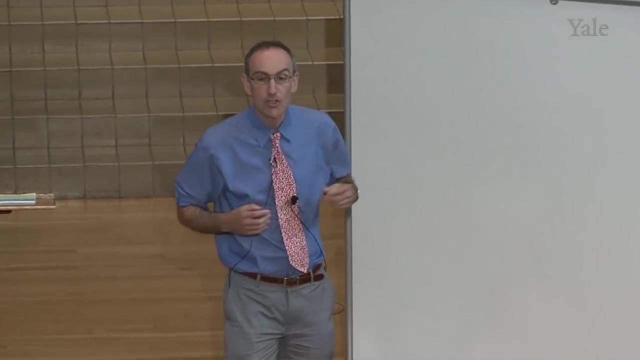 telephones to make these things. Whoops, just knocked off the mic. Make these things, And they have very There are strategies available to each other: Pricing quantity, innovation, suing each other, bribing juries, whatever else they do. 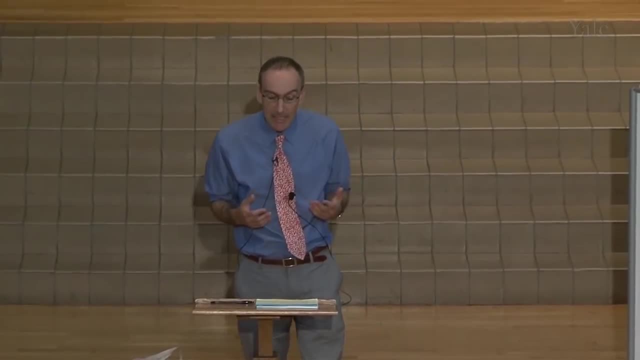 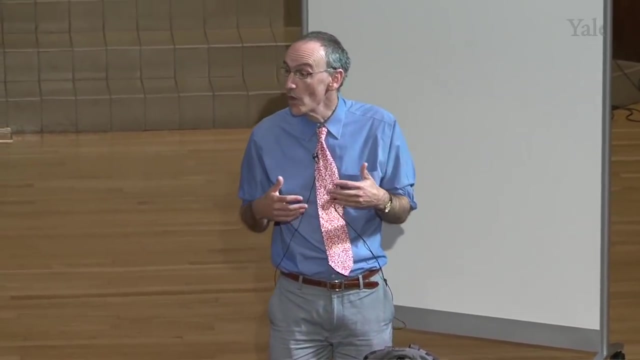 So that's a game involving players where they're competing, but it isn't only competition that we can model. We can also model settings of cooperation. So think about teams working on the same firm or, looking around the room, groups of deans and vice presidents of Yale. 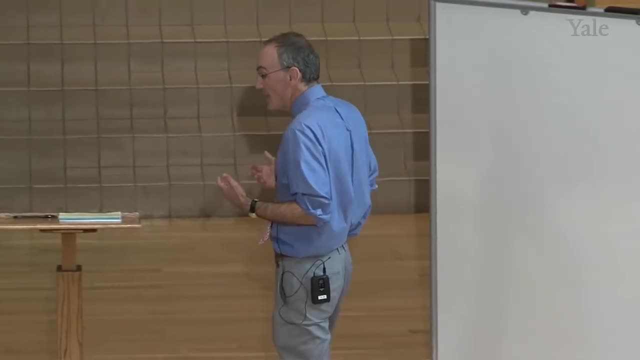 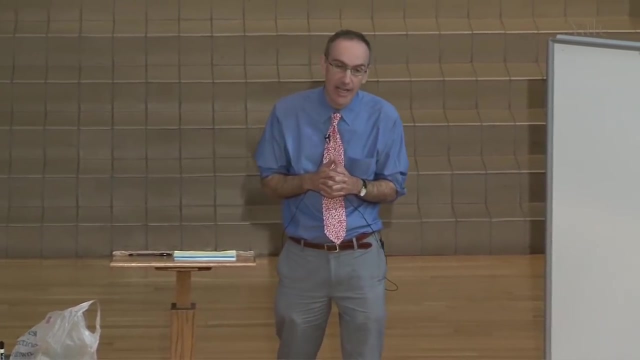 who are working together to try and get things done. So game theory is. Game theory is also the way you analyze how to herd cats, roughly speaking. So when we teach Game Theory at Yale, what we do is we try to play games in class and 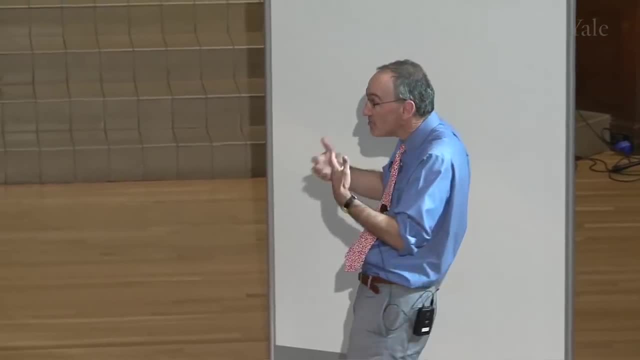 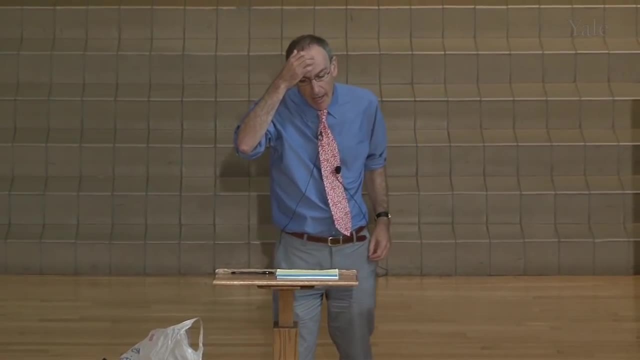 we analyze them as a way of teaching the technique, but also learning about the game. That's a technique of teaching that's now spread pretty much worldwide, and it's what we're going to do today. So today I'm going to play a game. We're going to analyze that game. We're going to 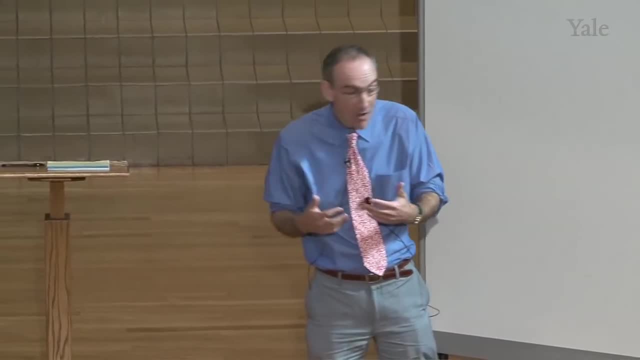 play the game. We're going to analyze that game And we heard the game. We're going to play it. We're going to play that game And we hope. I hope we're going to learn something as we're going along. 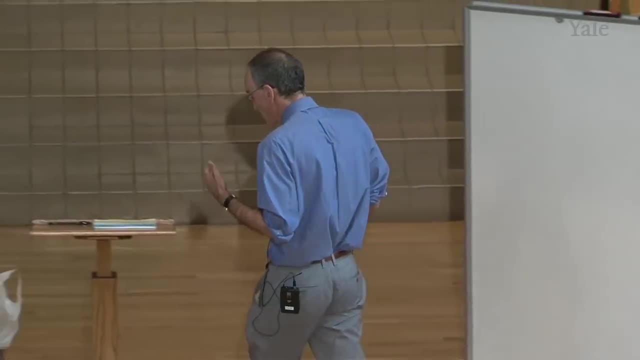 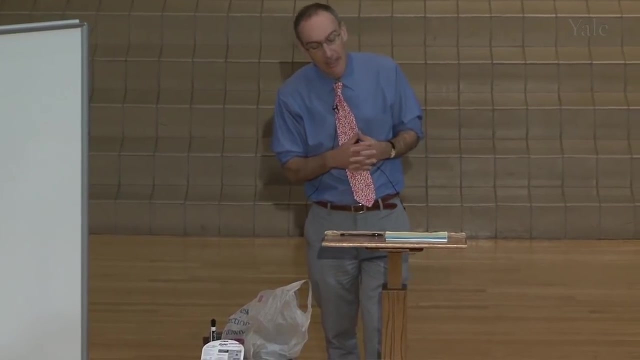 Okay, So that's what we're going to do. If some of you would have seen this game being played online- if you've seen my online courses and if you haven't, you'd be able to plug in for looking at the Yale online courses- Not just mine, but everyone else's as well. 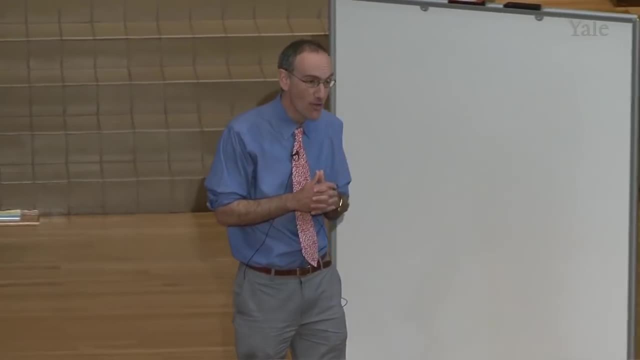 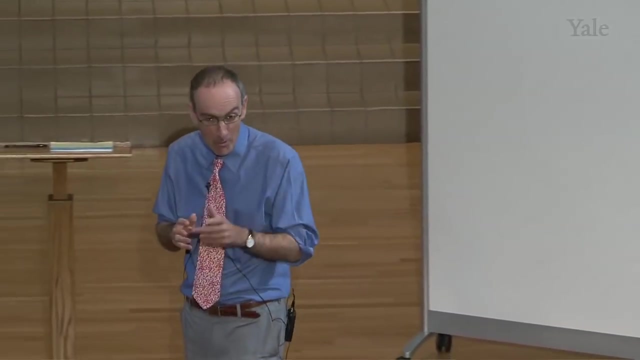 So I need two volunteers for this and, rather than embarrass people, I'm just going to pick people out. So I'm going to pick two deans who happen to be here, who didn't know this was going to happen. Pick Robert Post, who's here, and I'm going to pick James Bundy, who's there. 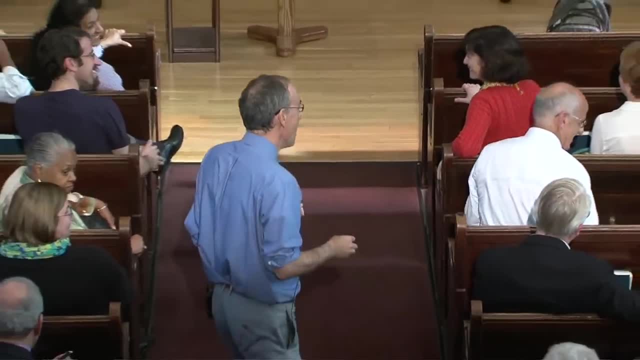 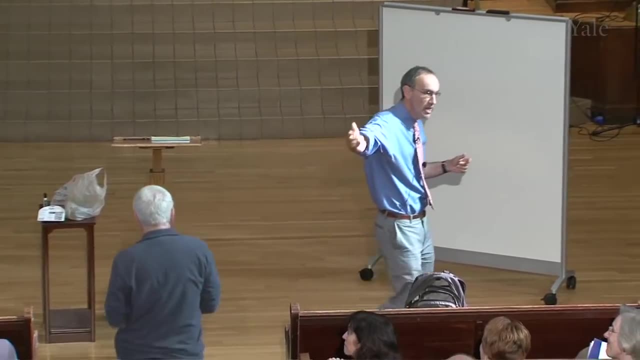 and I'm going to drag them out the front. One reason for picking on these two deans is this is a day to celebrate Yale. Robert Post is the Dean of the Law School, which is quite simply the best law school in the world. 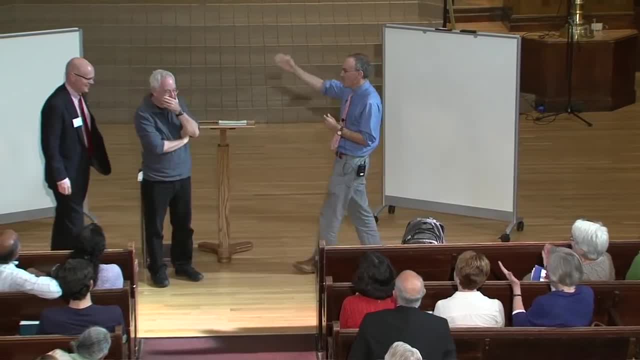 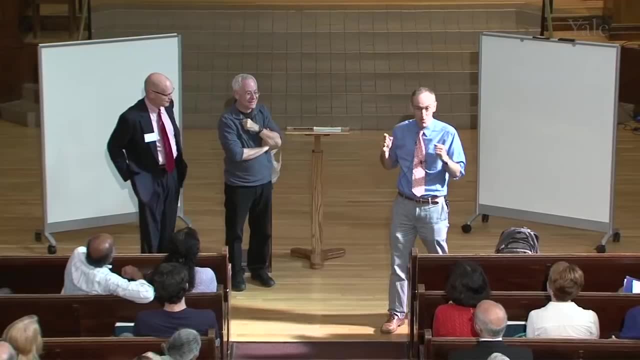 and he is quite simply the best Dean of the best law school in the world. James Bundy is the Dean of the Drama School, which is the best drama school in the world, and he is quite simply the best Dean of the best drama school in the world. 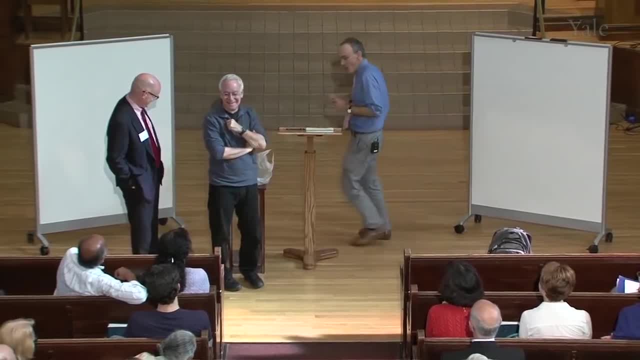 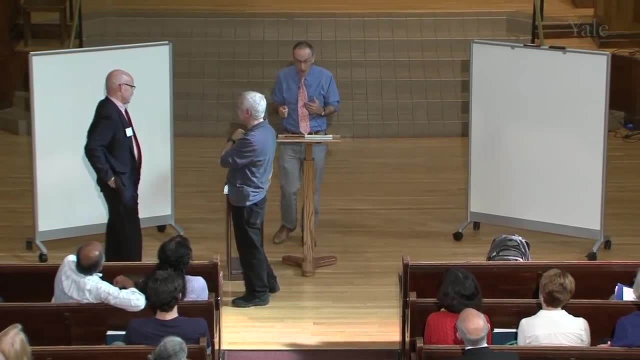 Why don't we have a little plug for our wonderful schools while we're here? OK, so the audience provides the volunteers. I'm going to provide the props, which on this occasion is two wet sponges. We're going to have a sponge fight. 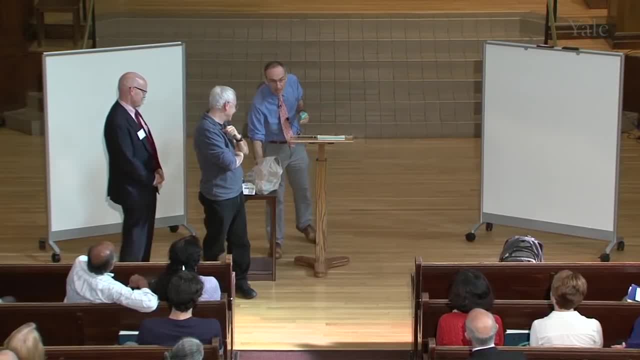 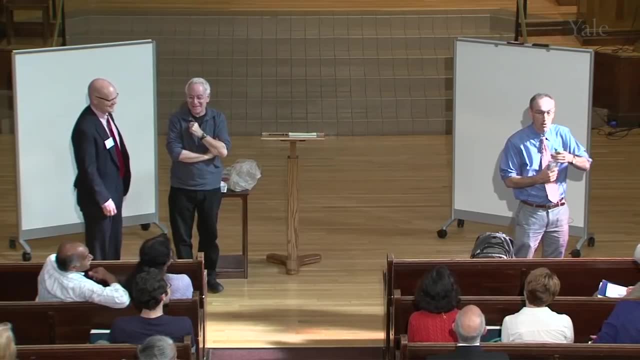 So these are the sponges and I'm going to wet them And, this being Yale, I will use nothing but the best. I'm going to use Yale University spring water. Did you know that Yale University had a spring? I don't know. 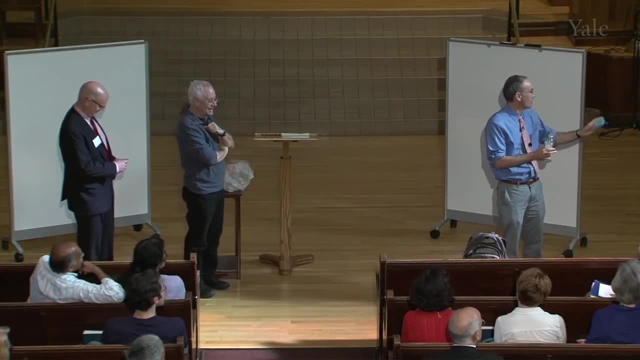 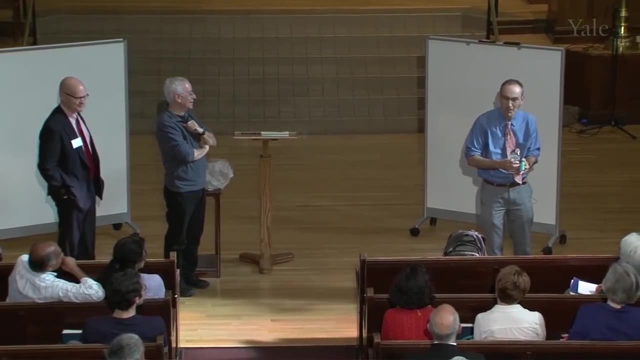 And we're going to wet these And the people who are custodians of this building. you're going to look away for a second because I'm going to dribble water on the floor And Bruce is back there and he's thinking the facilities bill is going to cripple us. 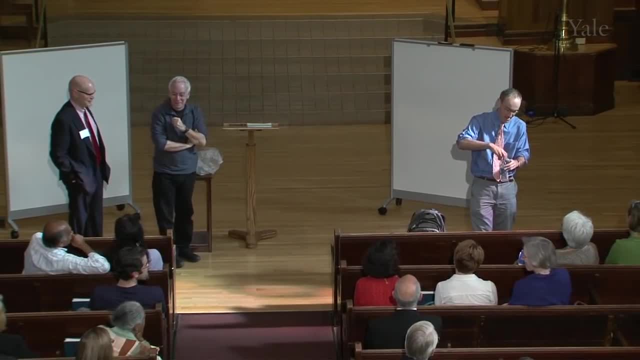 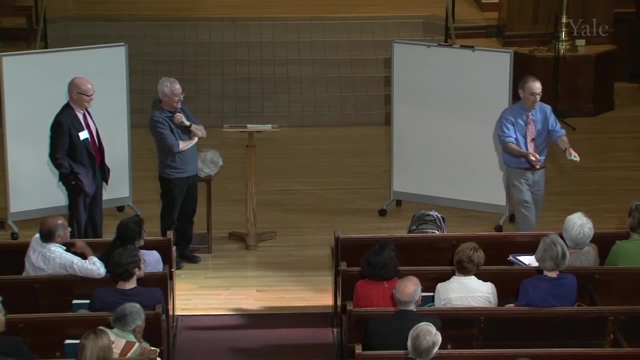 So don't look for a second Bruce. All right, and I'm going to squeeze these out and try and make sure they're roughly equal weight, All right. so, Joan, are they roughly equal weight? Yes, OK, so we have a blue sponge and a green sponge. 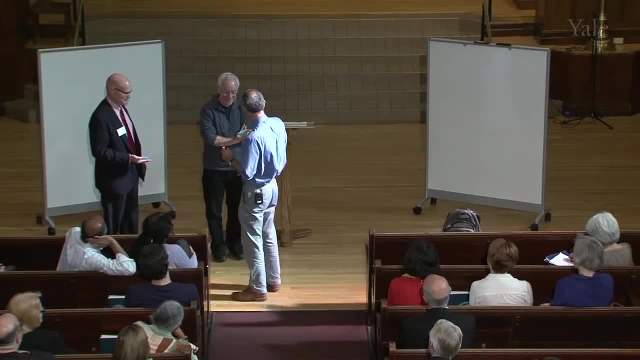 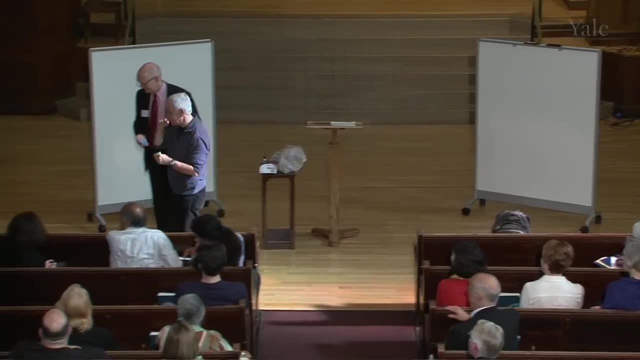 I'm going to give the blue sponge to James Bundy and I'm going to give the green sponge to Rob Post, And the minute I'm going to position them at either side, I'm going to put Robert here and I'm going to put James here. 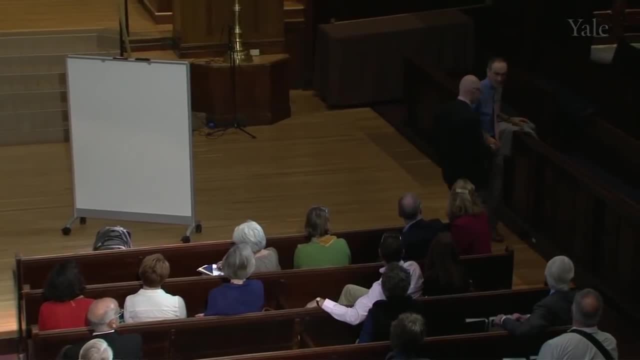 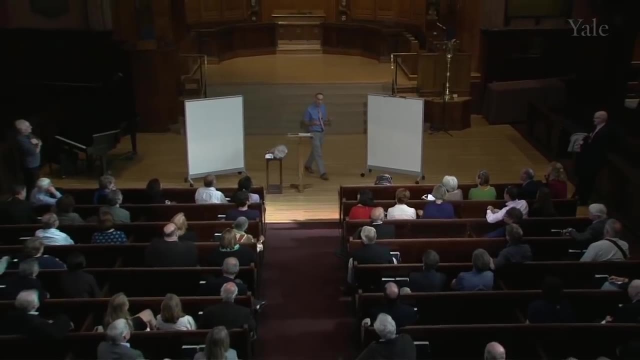 OK, I'm going to move my coat out of the way. All right, here we go. So we're going to have a sponge fight or, if you like, a duel, And the rules of the game are this: We're going to have alternating moves. 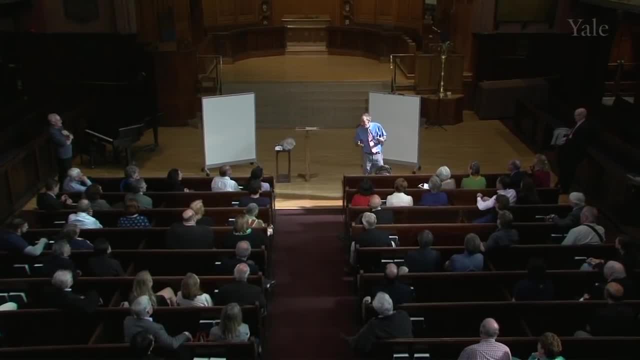 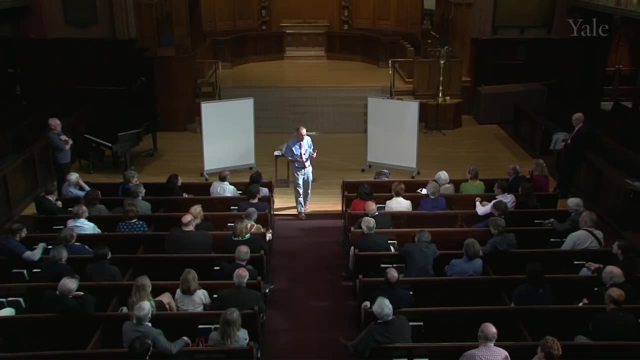 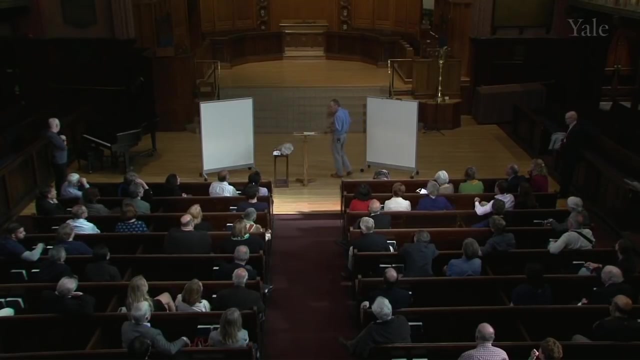 All right. When it's your turn to move, you are going to have to make a choice, And the choice is going to be whether to throw your sponge at your opponent or whether to take a step forward. If you throw the sponge and hit your opponent, you win. 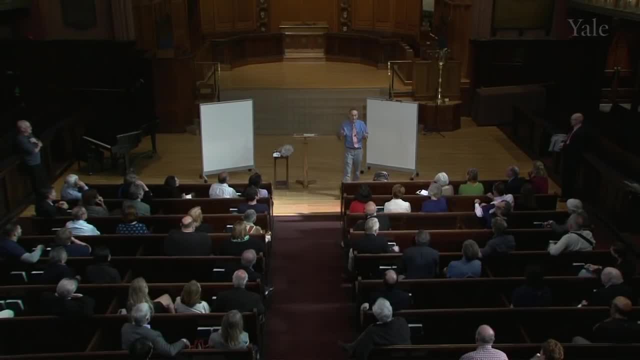 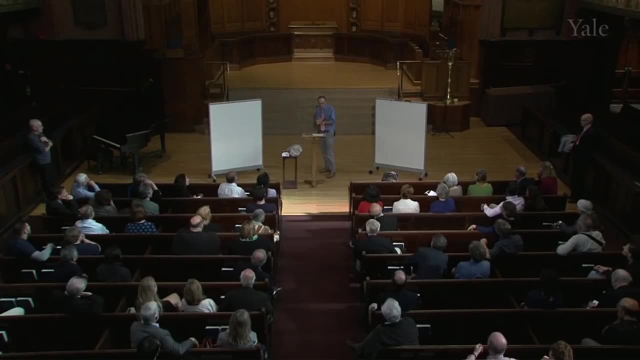 If your opponent throws his sponge and hits you, you lose. Simple rules. We'll need a few specifications, ones that are important, but the most important specification is this: Each player only has one sponge, And once they've thrown their sponge, if they miss. 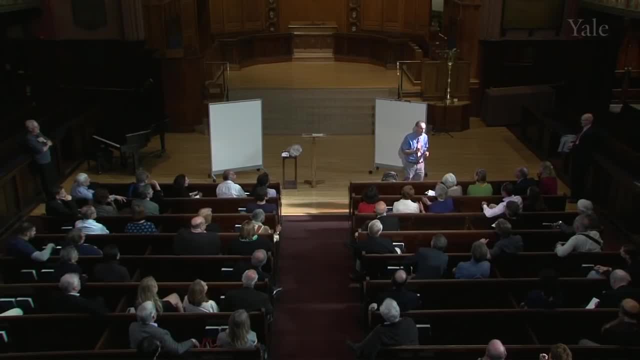 the game continues. Oh, All right, So we could work out the strategies in great detail, but let's not. Let's just realize what's going to happen. So if you throw your sponge and you miss, since you have to keep on stepping forward, 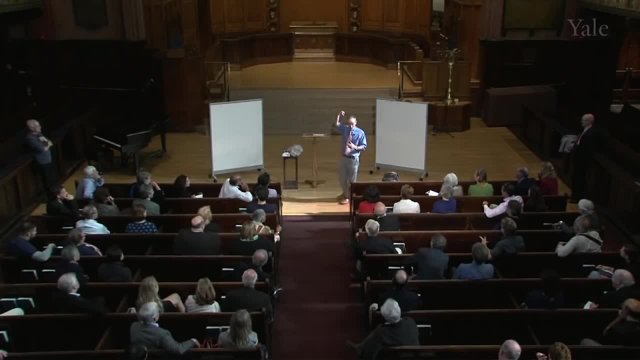 eventually, the other player is going to be right on top of you and it's going to basically plonk. It's going to plonk his sponge on your head. So if you throw your sponge and miss, you're going to lose. 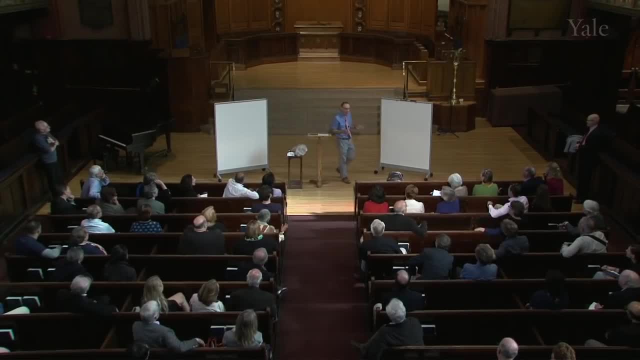 But we will play that through and see what happens. Two other rules, minor rules. Each step has to be about a yard to keep things fair, And this is a rule that I don't know will work in America, but let's see. 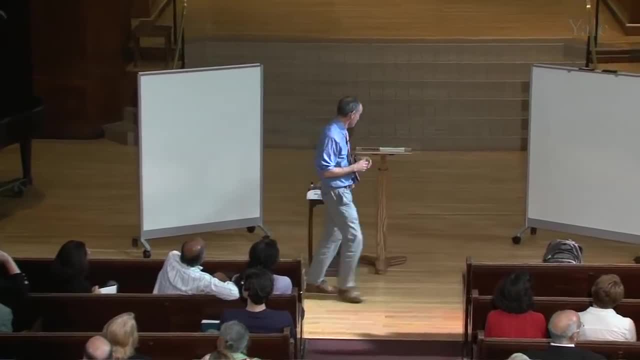 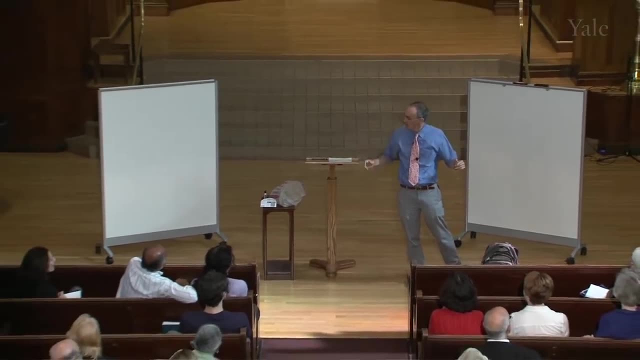 Gentlemen, never duck, OK, All right, All right, OK, All right, So we'll see. if that's OK, Does everyone understand the rules? All right, so we'll make James player one and Robert player two. I'm exploiting you rather. 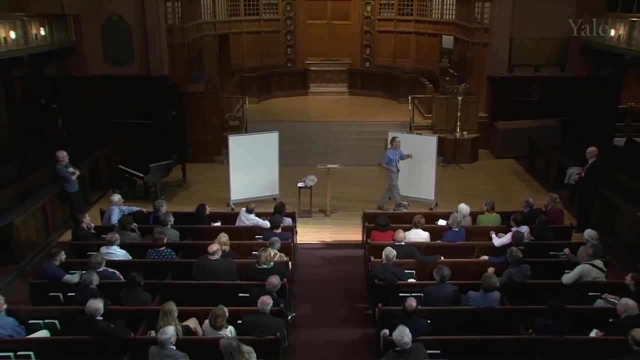 I apologize, but deans are meant to be exploited by provosts. It kind of fits, It hits on the roll. So, James, do you want to throw your sponge or step? I'll take a step, Take a step. OK, so a step. 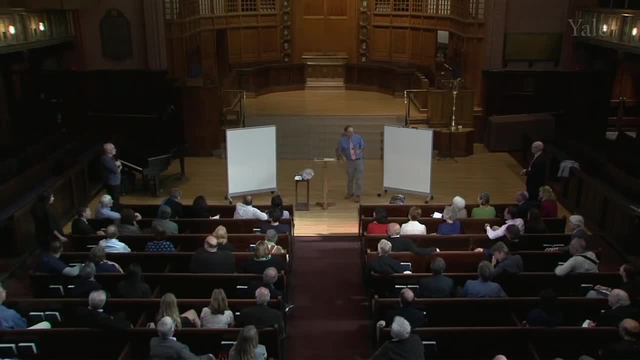 And now it's Robert's turn, and he's also going to step. And now it's James' turn. He's also going to step. All right, now it's Robert's turn. He's going to step. Now, at this point, let's just pause a second. 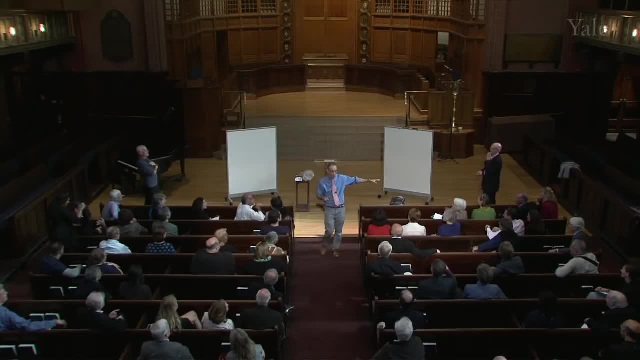 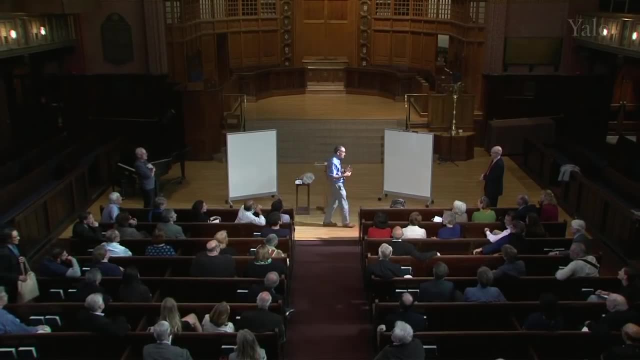 and let's ask people what they think people should do. So it's James' turn. You can all see the situation. One of the things we think about in game theory is how to put yourself in the shoes of other people. So imagine you're in James' shoes right now. 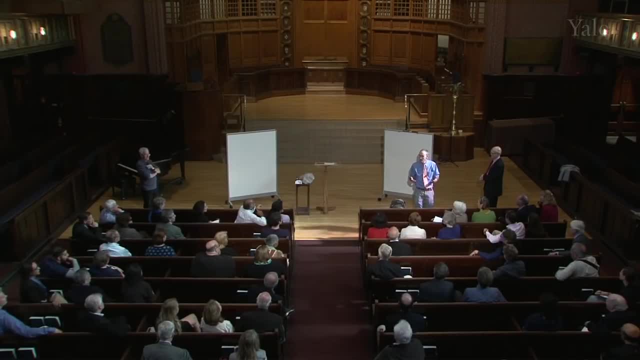 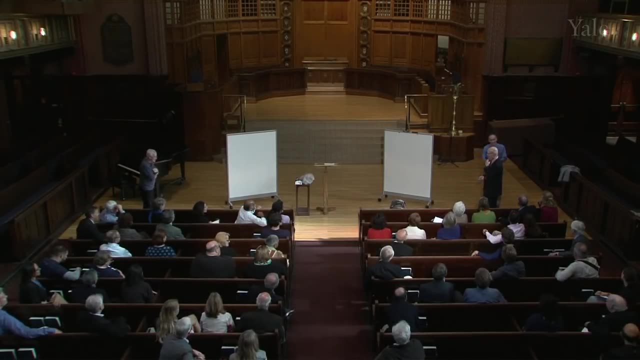 Would you throw Or would you step, Step, Step, Step. Everyone thinks they'd step. OK, They're all saying step. They don't trust their arm. I don't know how you are at baseball, All right. so that's the same question now for Robert. 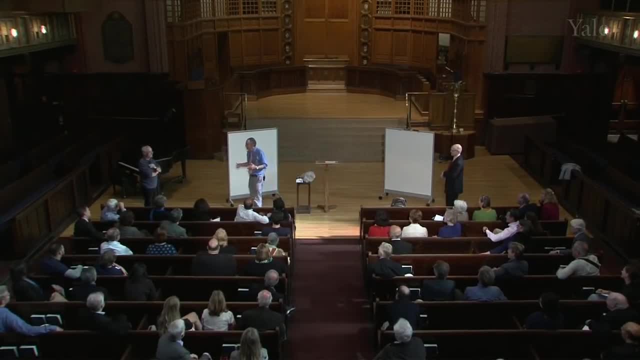 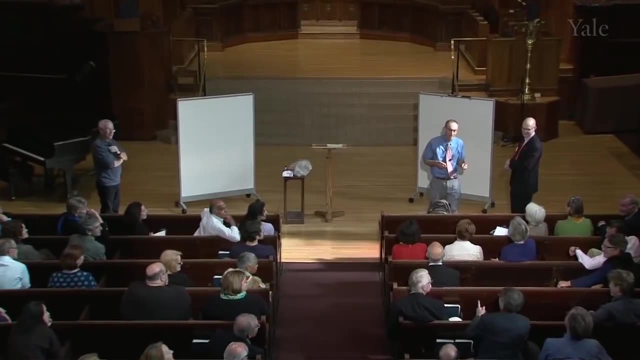 Who thinks he should throw, Who thinks he should step, Step, Step. They don't really trust the arms of the deans. OK, All right, All right, and now? yes, Can I ask another question? Are they allowed to try to dodge? 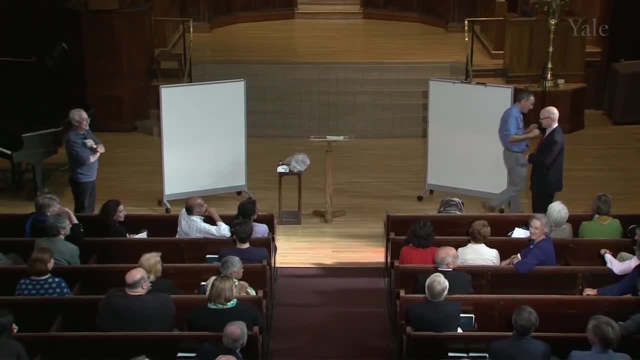 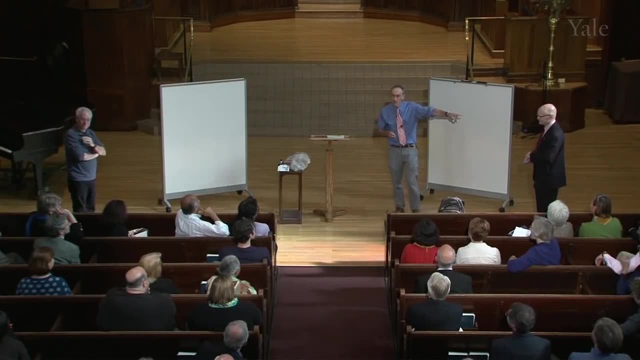 No dodging, No dodging. Not allowed Again. gentlemen, never do things like that. This is a strictly gentlemanly game. All right, so James' turn Who thinks throw Is James' turn Who thinks, throw Who thinks. 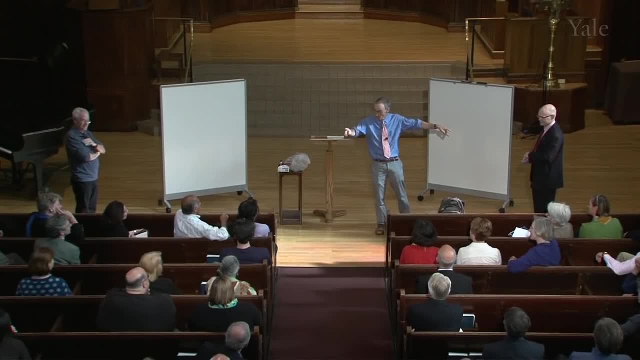 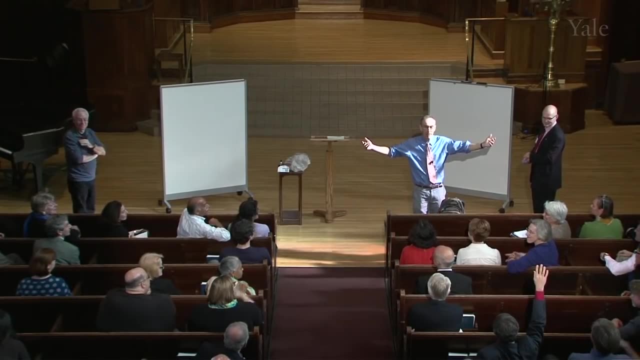 Who thinks You can throw it. You think throw. Shankar says throw, Raise your hand. if you think throw, Raise your hand. if you think, step, Well, it's up to you. I don't know how happy this one is. 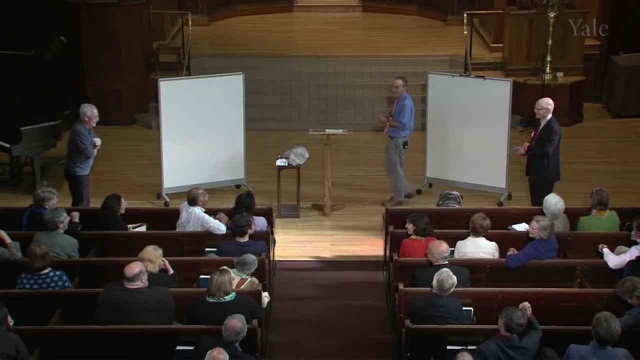 We don't know if it is baseball. We don't know that. We don't know that, We don't know. And it's a pretty light sponge, It's a big one. We've got to think. basically, step ahead, because whatever you do, 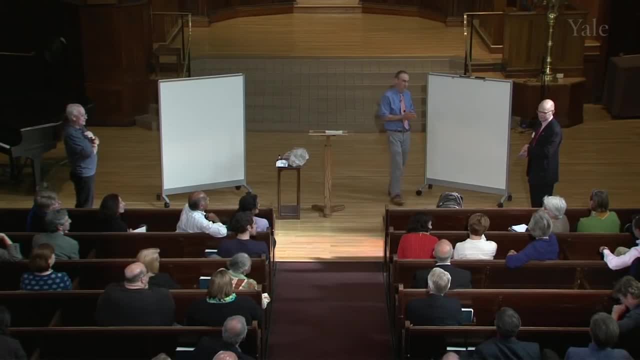 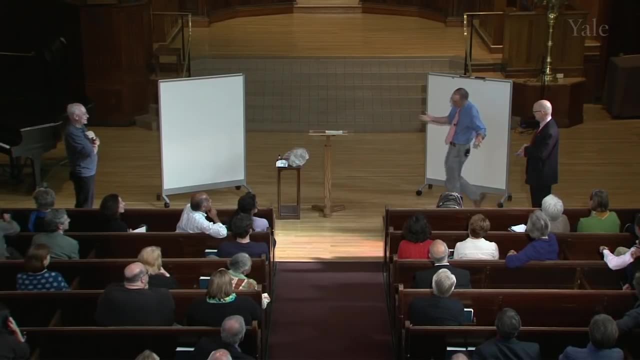 then you know that you'll come up against it. We'll get there. We'll get there. Hold that thought, but we will get exactly that idea, All right. so throw or step. Now I don't know what people think, Throw or step. 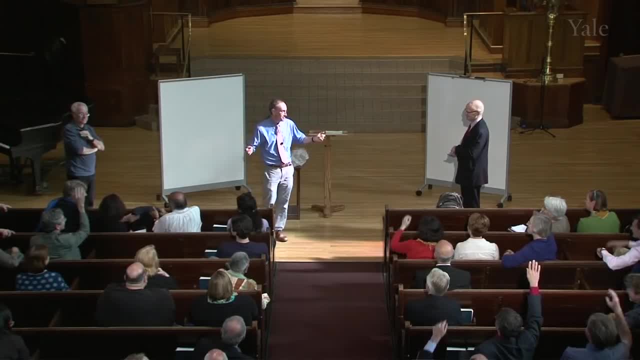 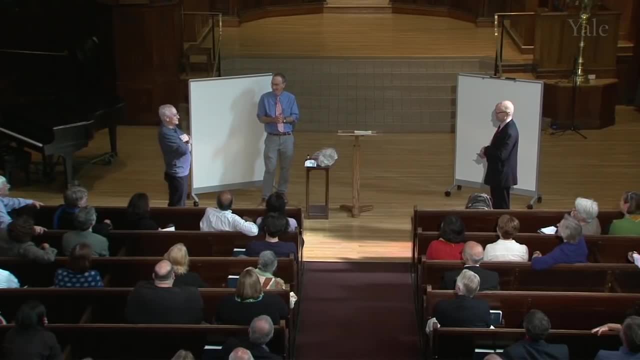 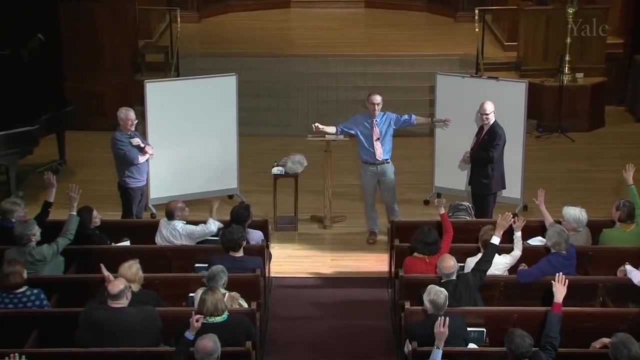 Who thinks throw now? Who thinks step now? Well, up to you Getting more, even More, even. Okay, Jane, throw or step Now. let's have a poll again: Who thinks throw, Who thinks step? Interesting, The people at the front are saying throw. 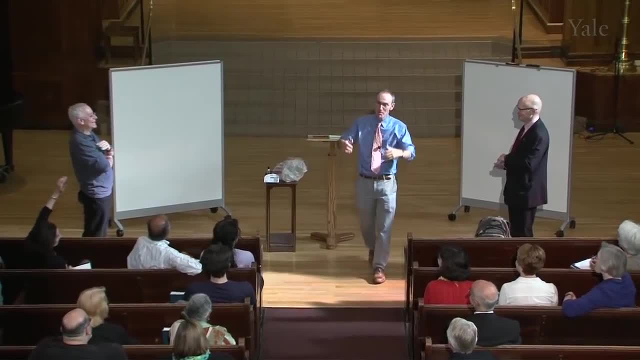 It's got to be a coincidence, but David Swenson is saying anywhere on the body, Anywhere on the body. David is saying throw, and he is the best judge of uncertainty in the room. How is he on air? I've been in the air for about 20 minutes. 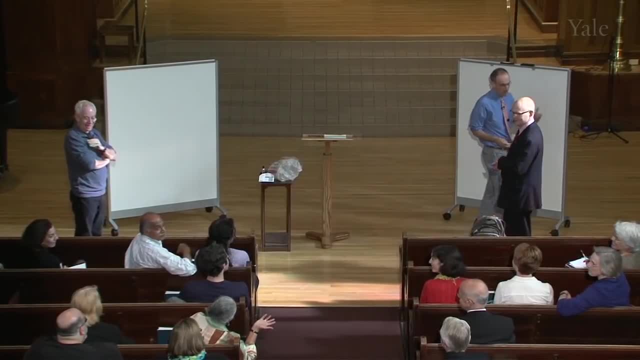 He's not on air. He's on air for about 20 minutes. Oh, he's on air, He's on air. He's on air, So that's not a real question. He's on air, So that's not a real question. 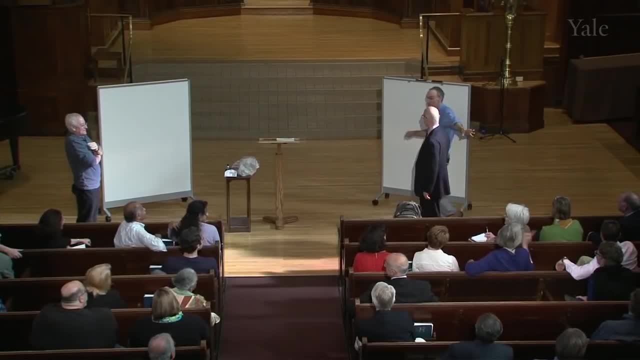 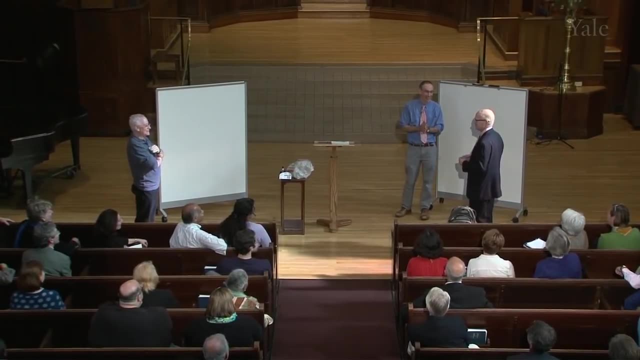 So that's not a real question. He's on air. He's on air. He's the best judge of uncertainty in the room. How is he on aerodynamics? I don't know about his aerodynamics. We'll have to find out. 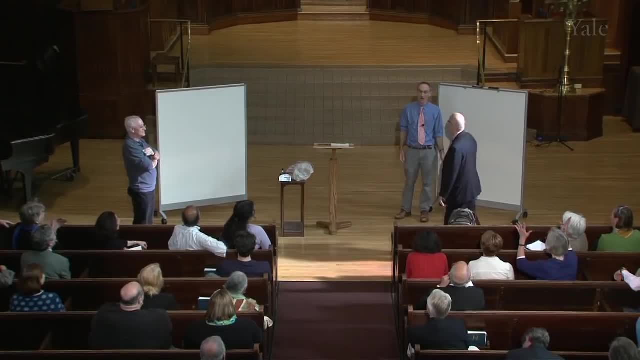 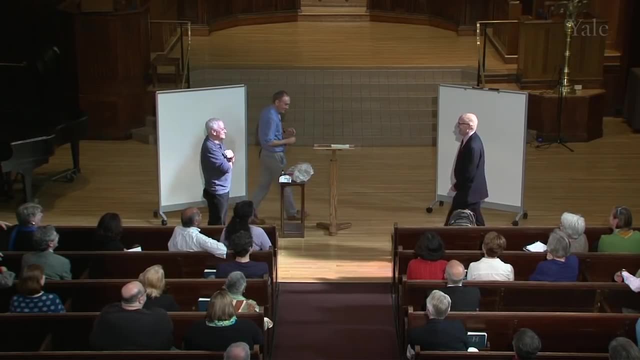 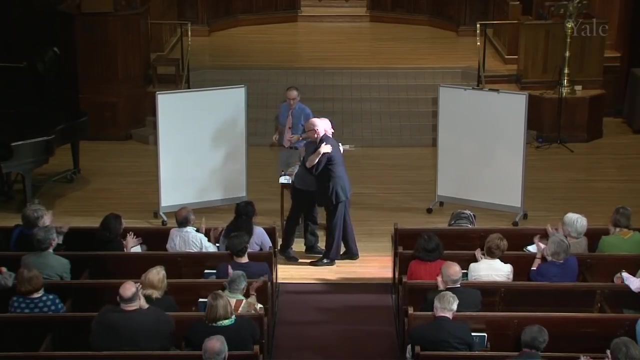 All right, ready. Oh, game continues. So I assume you're going to step and step and step and step, All right. So why don't I get you guys to sit here for a minute? because I'm going to use you in a second. 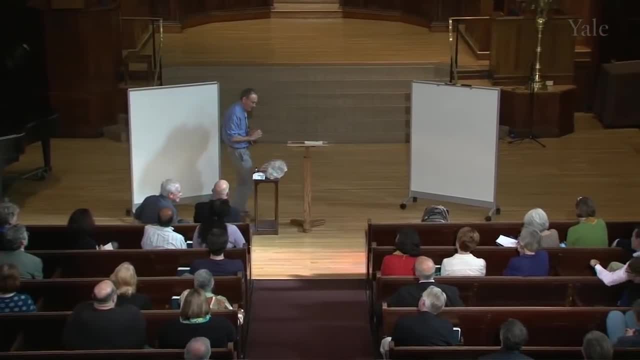 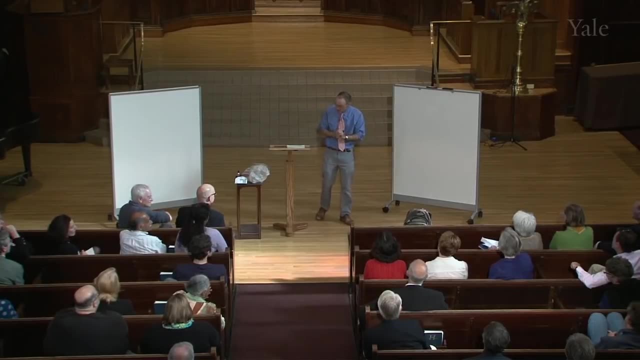 All right, so I'm going to victimize our volunteers a little bit more. later Let's talk about this game a little bit and see if we can learn something from it, And we're already beginning to draw out some lessons there, and we'll draw out more as we go along. 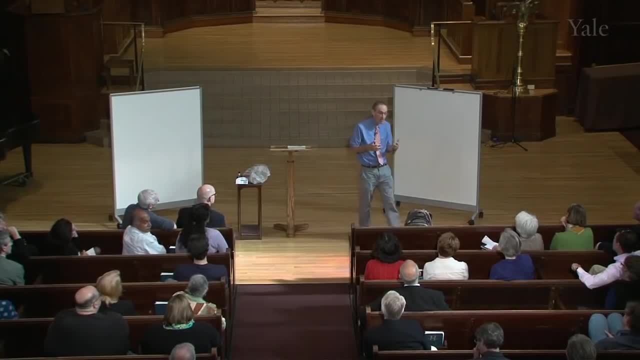 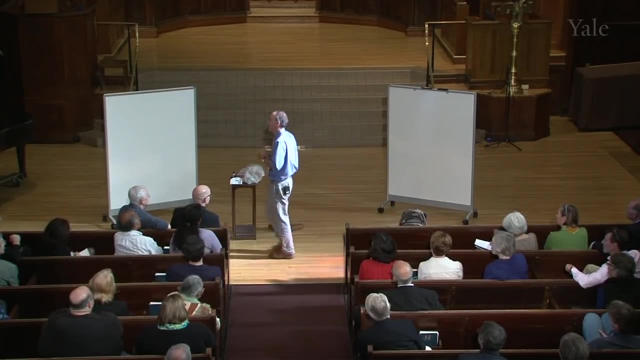 So, first, why is this game interesting? So one reason this game is interesting is it corresponds to a duel. a duel with muskets, I guess, a bit more serious than sponges, And for the people in the room who are Russian literature, 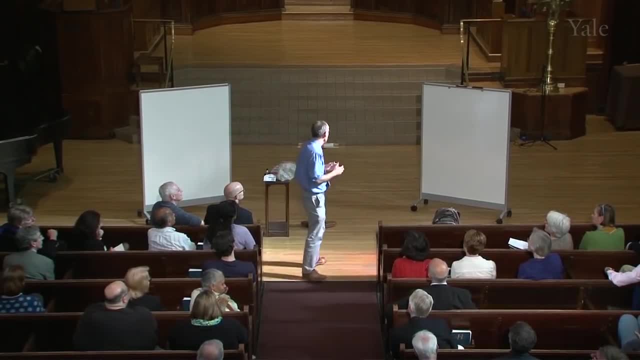 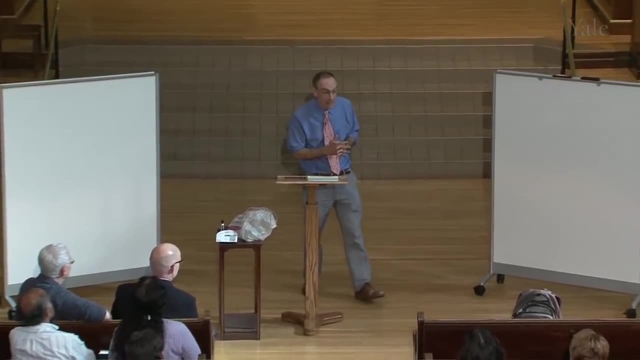 specialists, you'll know that there are plenty of duels in 19th century Russian literature, a little bit in French literature. Probably the most famous, I'm guessing, are the one in War and Peace all right, and the one in Onegin, the Pushkin one. 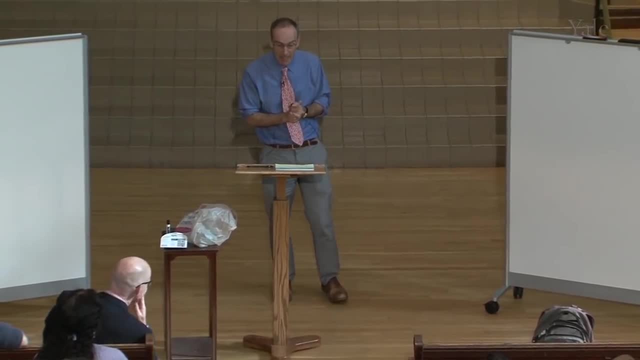 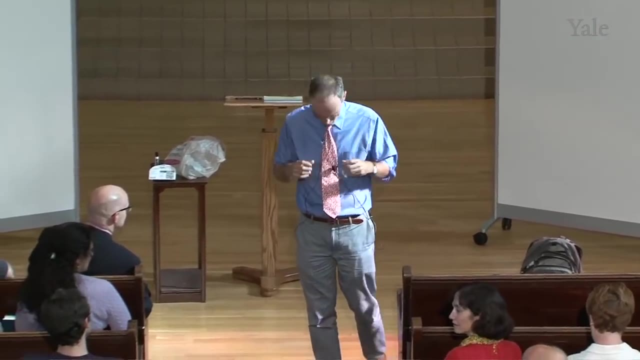 or Tchaikovsky, if you prefer that version. There are many, many others In the War and Peace version. there are other examples, better examples, Oh, yes, up, Better, Better, More up, Okay, Higher, higher. 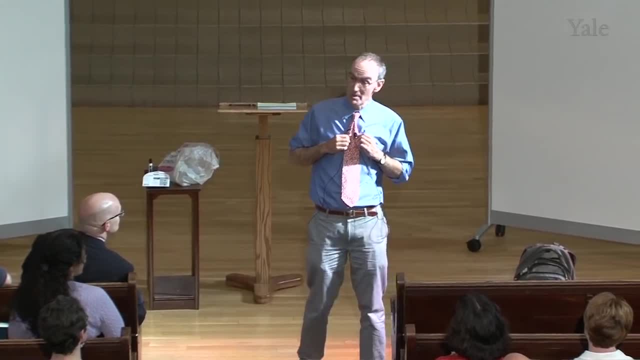 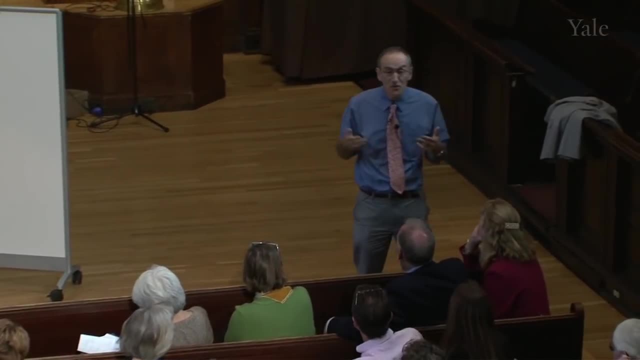 Better. It's a big room. Is that better, Good? Okay, so in the Tolstoy, in the War and Peace version, I think we are led to believe that the hero Pierre shoots his musket too early and he kind of gets lucky. 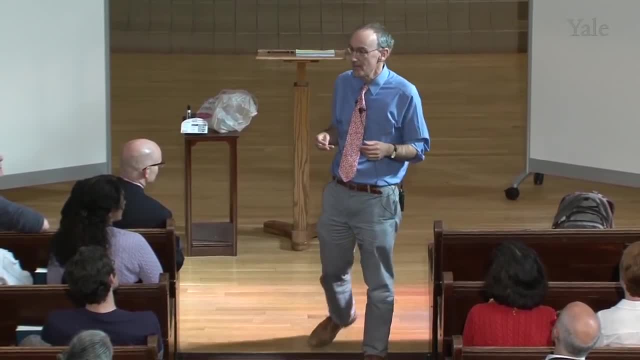 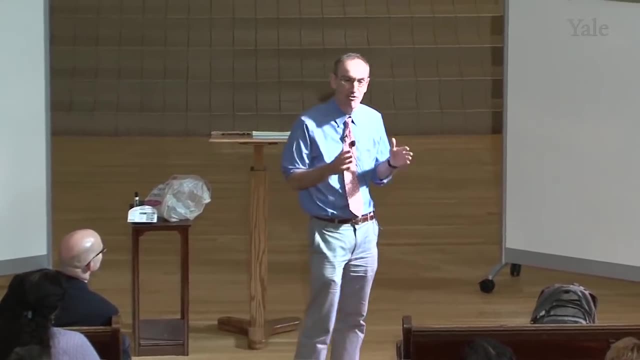 and kind of wings the dollar off. I know that's a spoiler alert, but that actually happened about page. that's about page 300 in the novel, which means it's in the first half of the book, right? So there's plenty more after that. 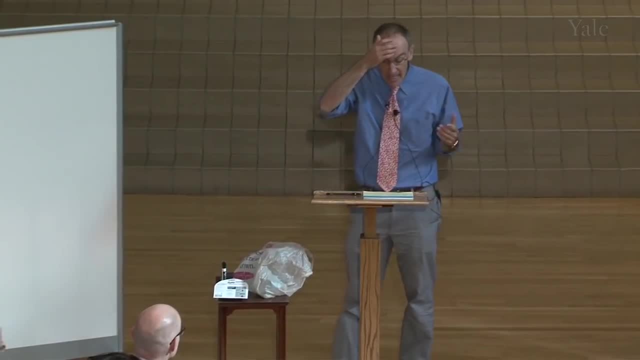 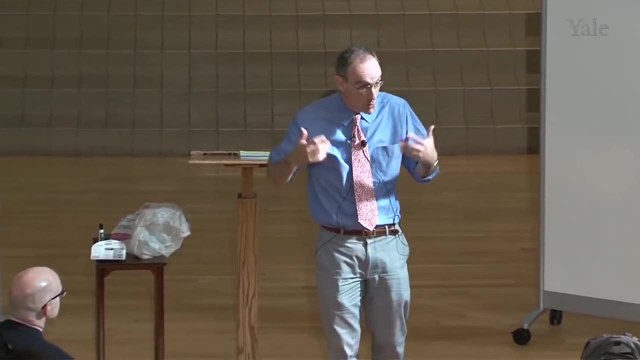 In the Pushkin version in Onegin, Onegin kills Lemski. It's really the critical event of the poem And I think the main lesson we should get from this for dueling is don't duel right, Rather than how to duel. just don't duel. 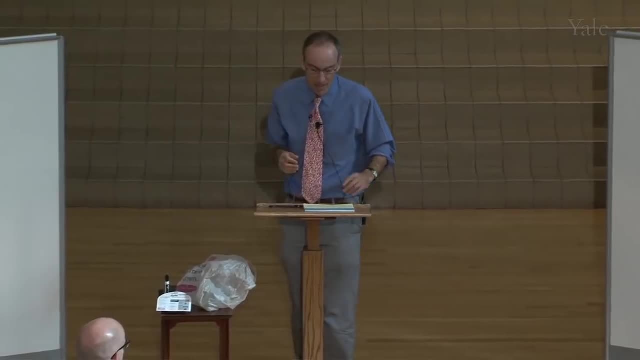 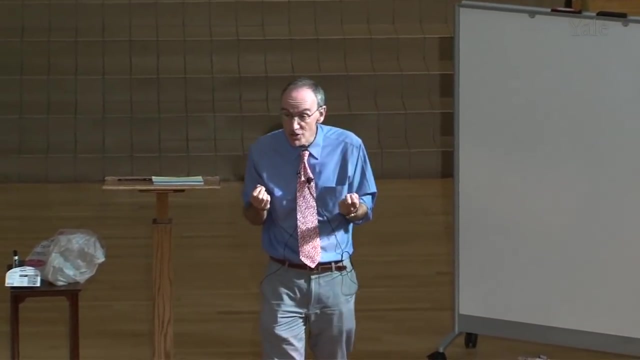 But if you did find yourself in a time machine in 19th century Russia, this might help. But there's more to this idea than just duels. There are games elsewhere where the critical decision is when to do something. There are games when what matters is what you would do. 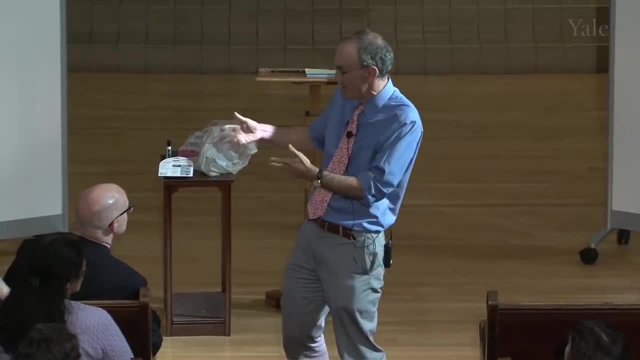 and there are games where what matters is when you would do it. So in this game, there's no question about what you're going to do- You're going to throw the sponge- But the critical question is when you would do it. So let me give you an example. 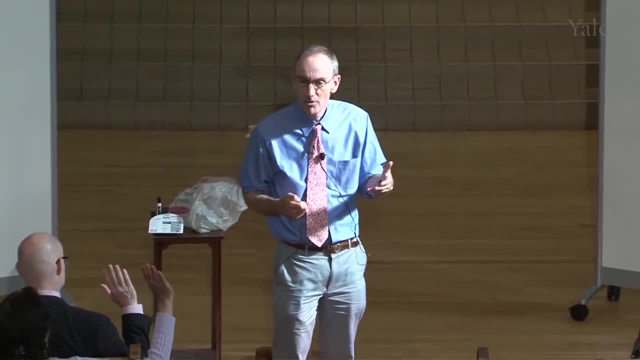 How many of you have watched the Tour de France on TV? A fair number of you, Actually, surprisingly few. And the Tour de France is a bike race, right In the Tour de France, in each stage of the Tour de France. 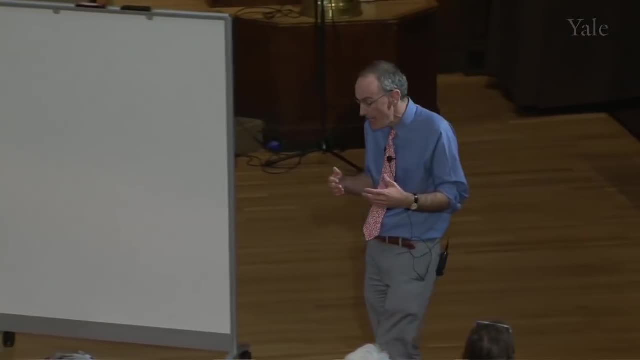 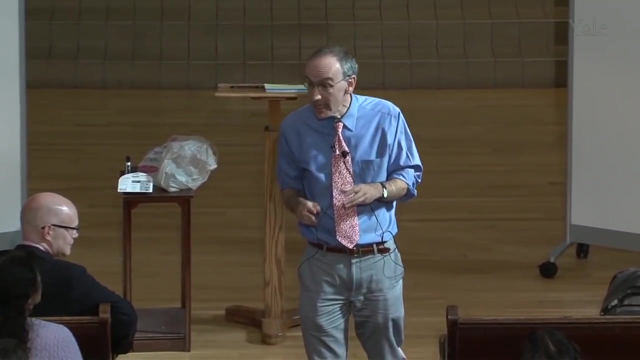 one of the critical decisions that each rider has to make is they have to decide when to try to break away from the peloton, from the pack. And if you break away too early in these long stages, for sure you're going to be reeled in. Because over very long distances the peloton will go faster than you can go, And if you break away too late, then either someone else will break away or just one of the sprinters will win. So the key decision then is when to go. 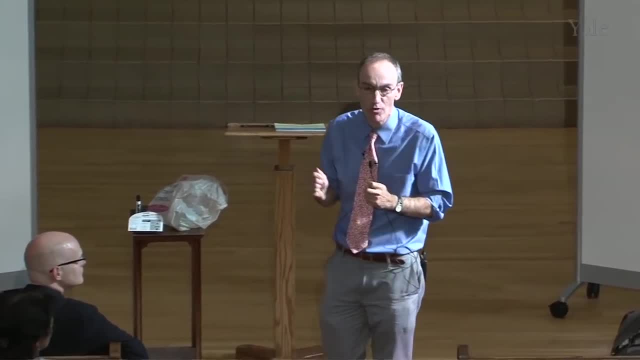 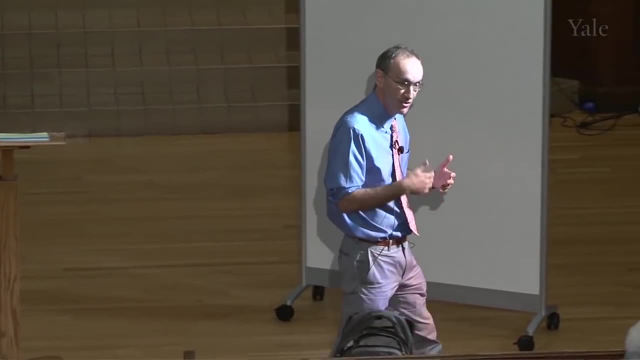 Not when to throw the sponge, but when should I break away? There's even an American movie called Breaking Away. So this is one of the main games within a game in bike racing. It isn't the main game within the game in bike racing. 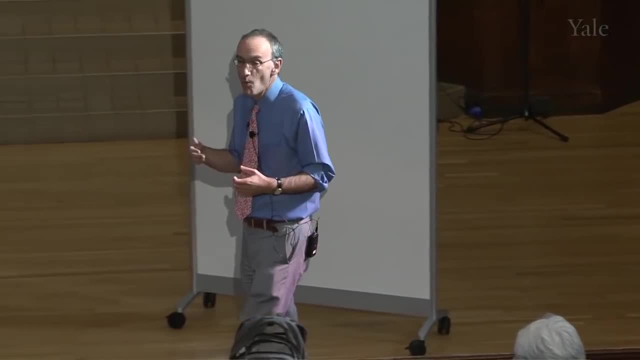 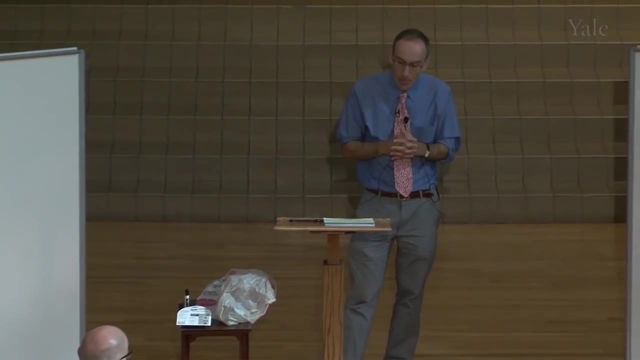 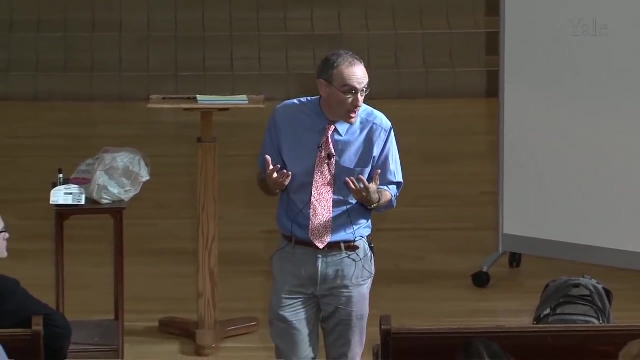 The main game within the game in bike racing is trying to figure out where to hide your steroids. But this is important. Let me give you an economic example or a business example. In business, you can imagine two firms who are both developing a new technology. 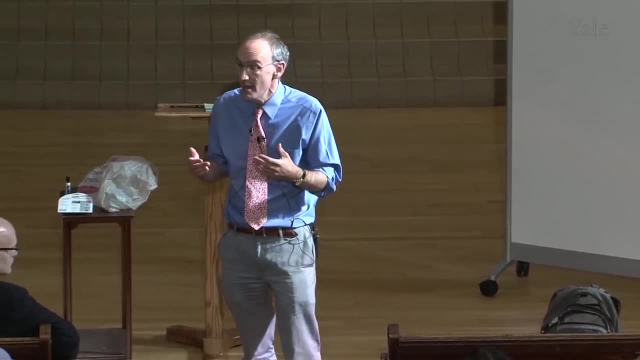 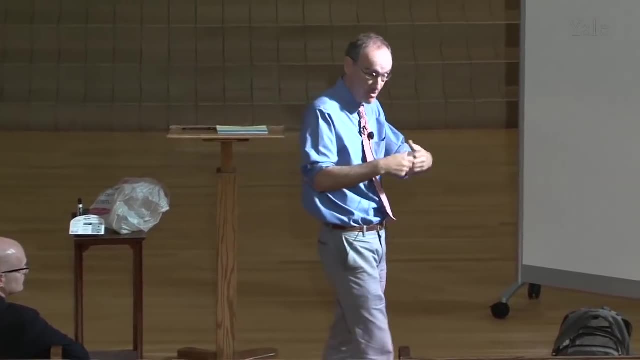 And that technology could be a new way to, for example, book air tickets online, A better way of doing that than the existing one. So both companies are busy doing R&D and trying to perfect this new software or hardware, whatever it happens to be. 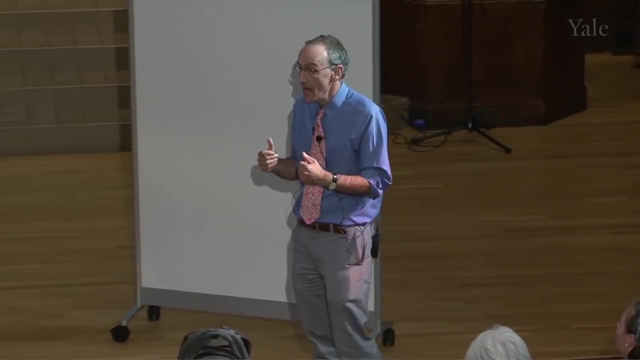 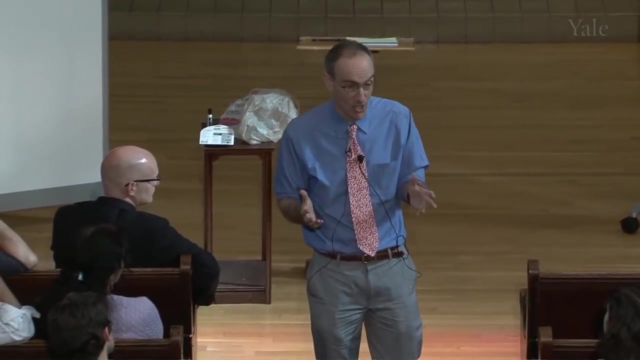 And they have to decide when to launch their software. And the problem here is, if you launch too early, when the thing hasn't been perfected yet, it might not work correctly and you're not going to get a second chance. Basically, if it doesn't work, no one's going to trust you. 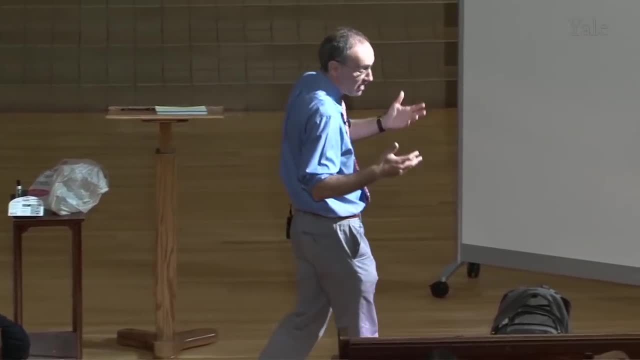 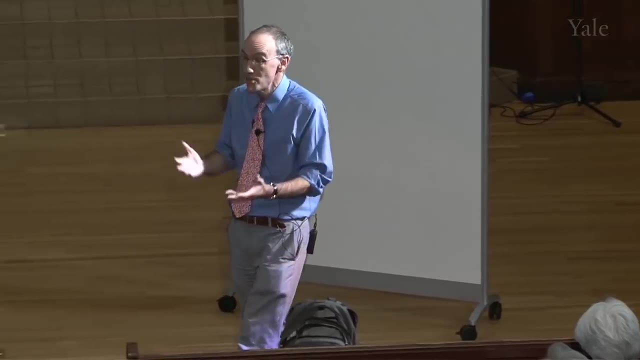 And if you launch too late in this particular market, the market I'm talking about- then the other guy will have launched already, The other firm will have launched already, His or her firm will have established a foothold and probably is going to end up becoming the standard. 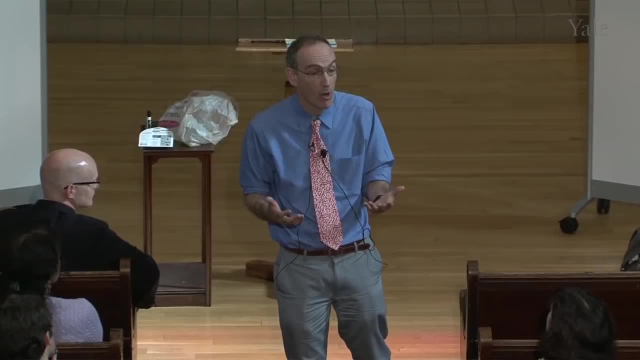 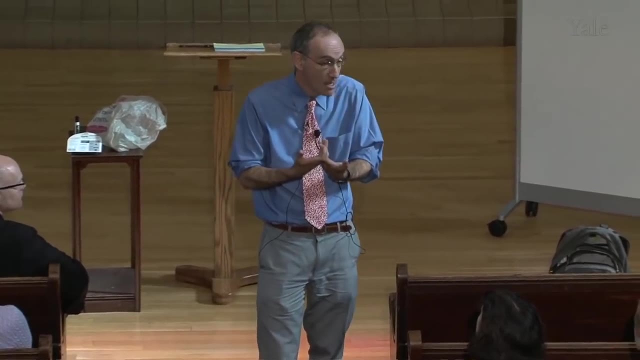 and being the whole market. So this is an example of a market where probably, at the end of the day, there's only going to be one player. So getting the critical foothold matters, But if you go too early, you launch too early. 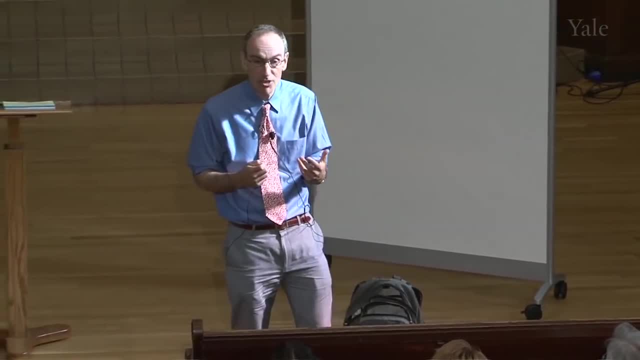 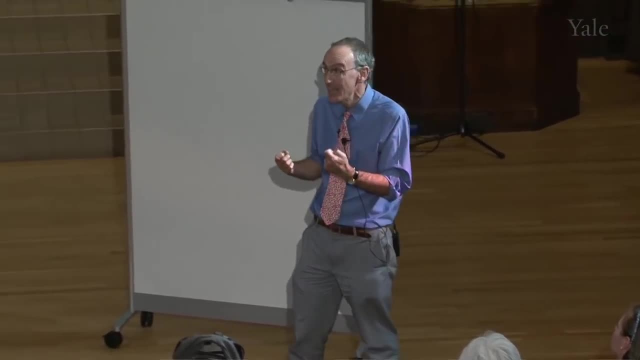 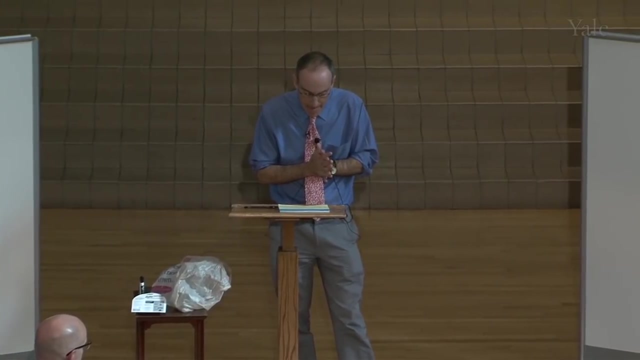 you're going to not be trusted by customers If you launch too late. someone else will have established the standard. So that's about launching a product, not launching a sponge, but basically the math of it is the same. All right, So we're going to analyze this game. 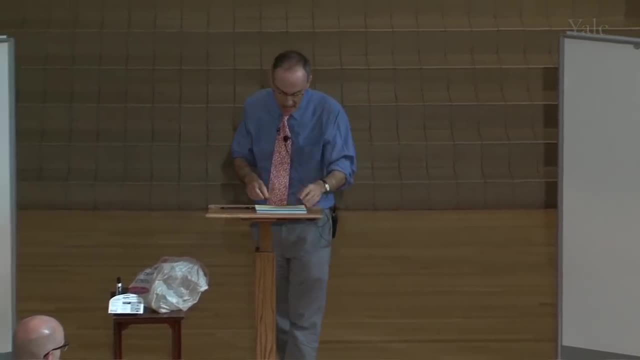 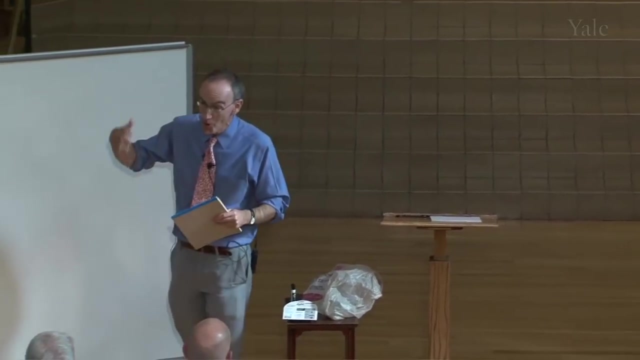 We're going to use these to analyze the game And I'm going to do a little bit of work on the board, but I want everyone to realize that when I say we, I mean we, So I'm going to help you along. 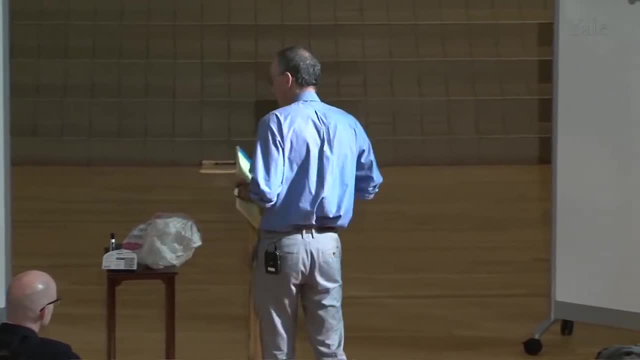 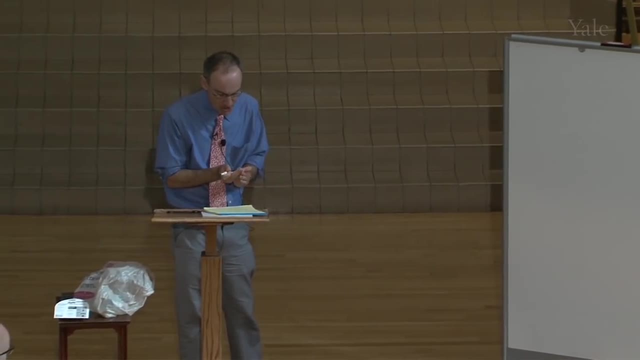 but you're going to solve this with me, So this is not going to be me lecturing. That's not what we do at Yale. We get people to participate. We just did So. to sum things up, before we do that, let me just establish a tiny bit of notation. 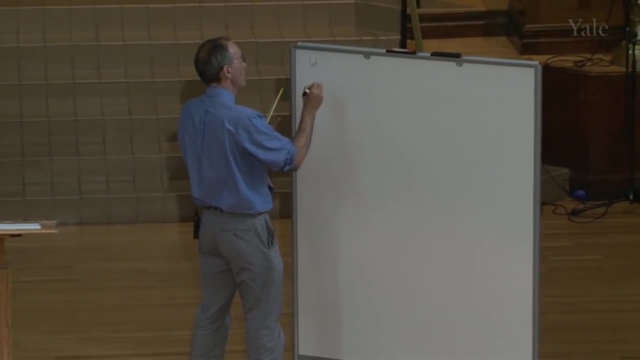 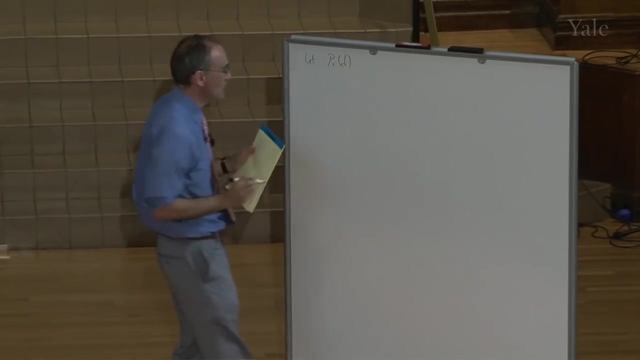 and draw a picture. So just a very simple bit of notation. I'm writing kind of small. I'm hoping it's going to be visible. Let P1 of D. this is the only notation I'm going to use. This is the only kind of mathy thing. 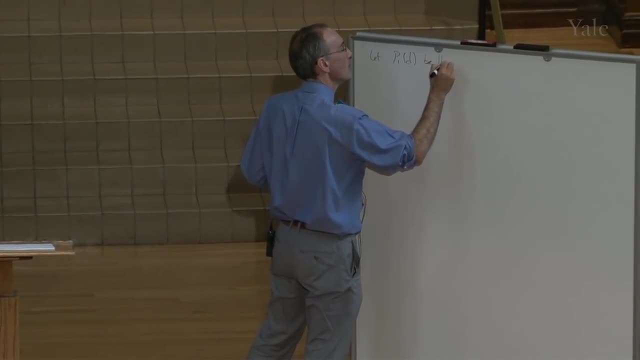 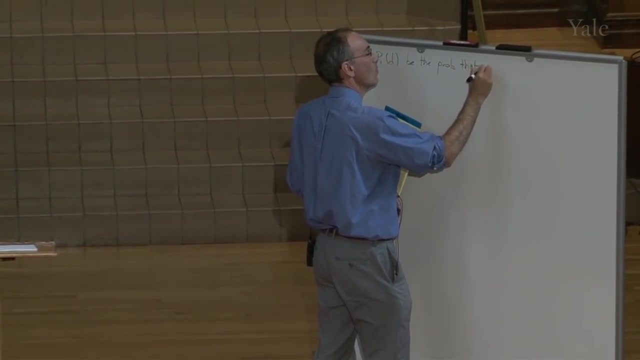 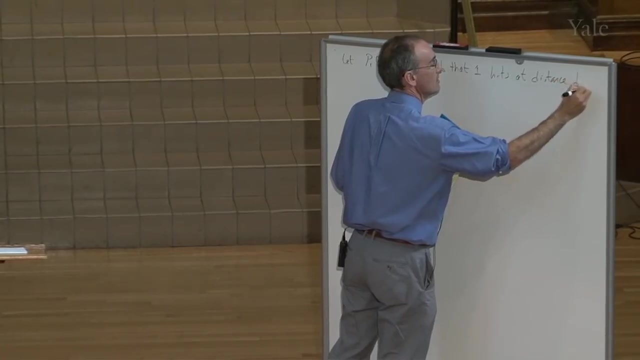 Let P1 of D be the probability, so I'll call that prob that 1 hits at distance D. So I'm going to use P1 of D to say we have to write it every time. P1 of D is the probability that player 1,. 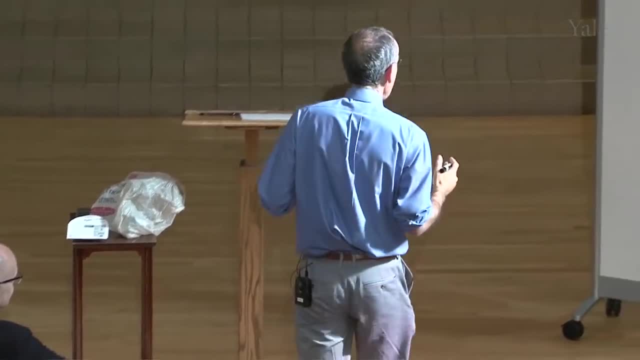 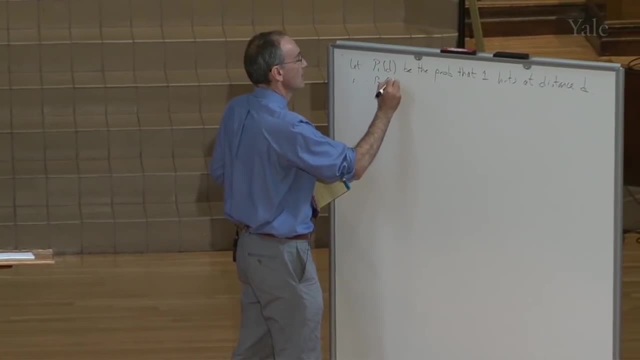 who, I guess was. who was player 1?? That was James hits. were he to shoot or throw a sponge at distance D? And similarly, let P2 of D be the same thing for player 2.. So I'm going to draw. 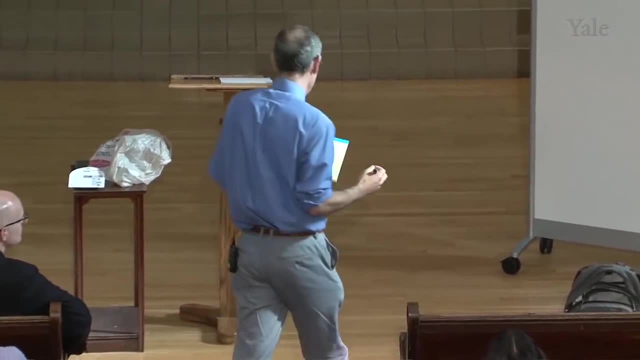 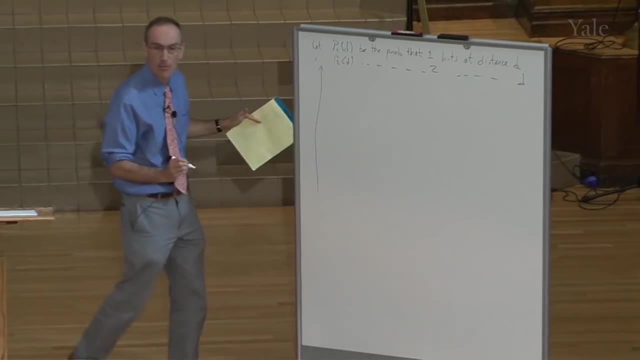 what I think these probabilities look like. I'm going to use a picture. We're going to use this picture for a while, So the notation is not as important as the picture. How low can I go before I lose the back of the row? 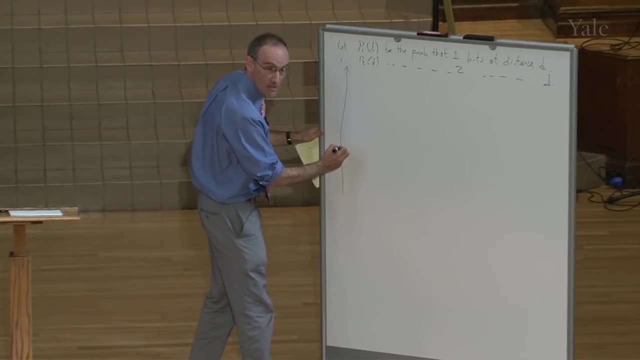 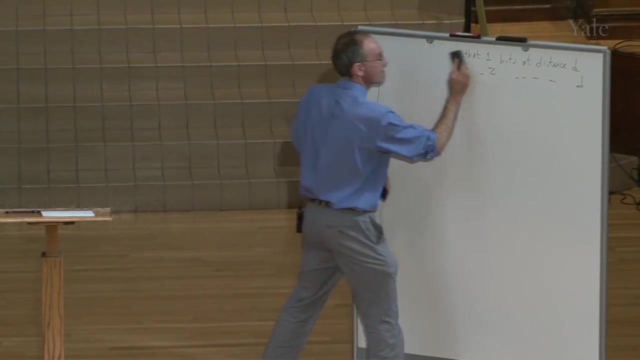 Oh, higher, Is that okay, Charles? No, Higher, still, Way higher. In that case, I'm going to delete the top line. Everyone know what P1 of D is. now I'm also going to push this back, perhaps, so you have a little bit of angle. 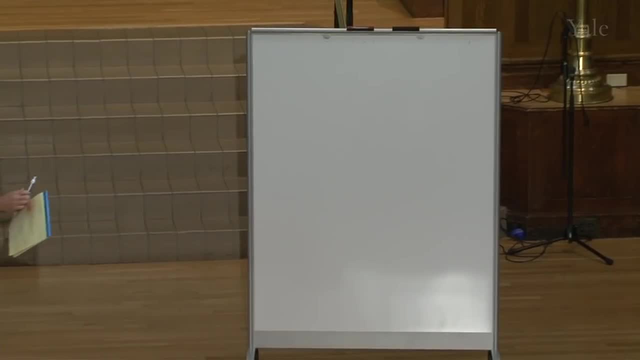 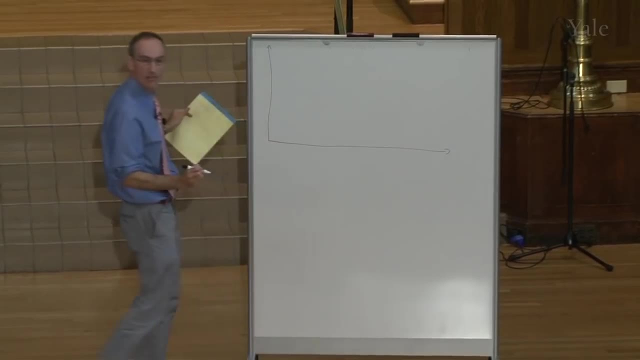 Don't hold it up on the stage. Is that better at all? All right, so let's try and do it right at the top here. Is that okay? Is that okay, Charles? Yeah, Okay, good, All right. so on this axis I'm going to put. 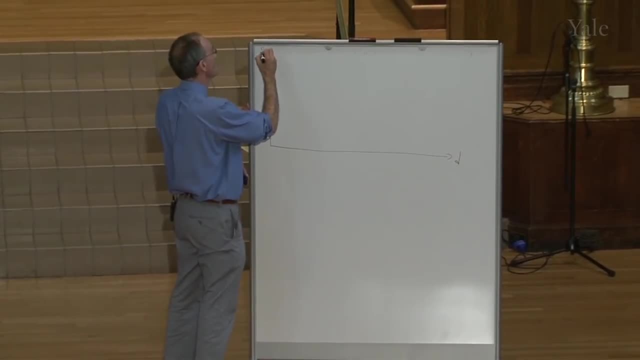 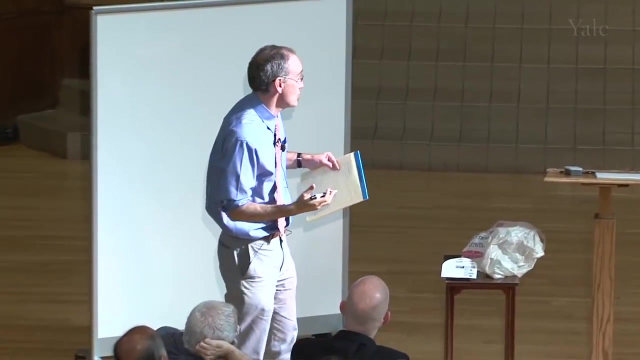 D, which is distance, and on this axis I'm going to put probabilities and I'm going to make some assumptions about the way in which these probabilities of hitting depend on distance. And at least two of these assumptions I think are inoffensive. and the third one: 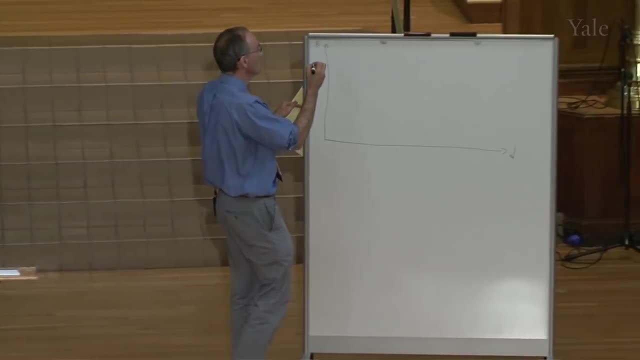 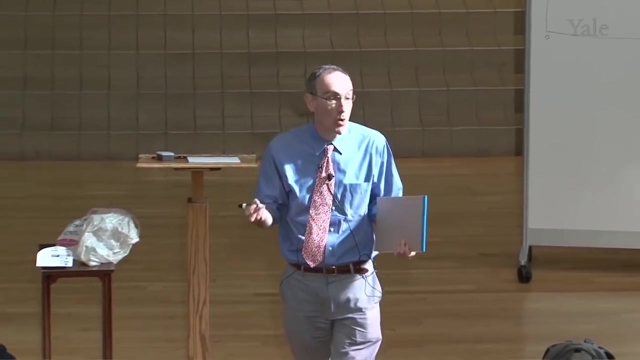 is offensive, All right. so the first thing I'm going to assume is that if you were at distance 0 and you shot at distance 0, what would be the probability that you hit if you shoot at distance 0? 1.. Okay, so 1.. 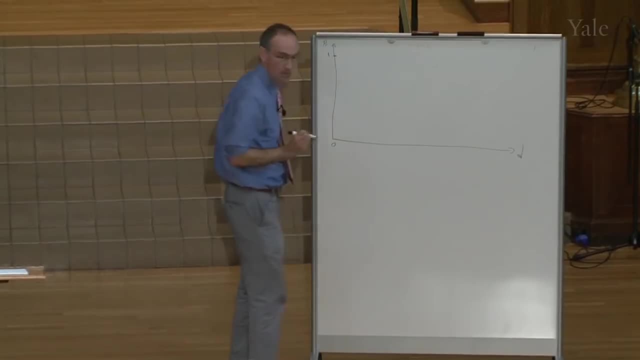 So that's an assumption, but it seems a reasonable assumption. So I'm going to assume that these probabilities start at 1 if we were at distance 0. Remember, I'm drawing this as distance, but of course the game is really going in this direction. 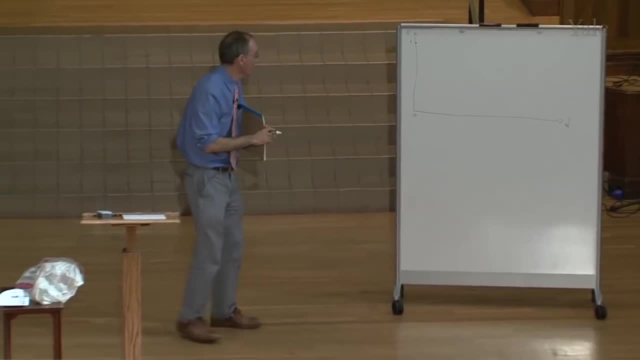 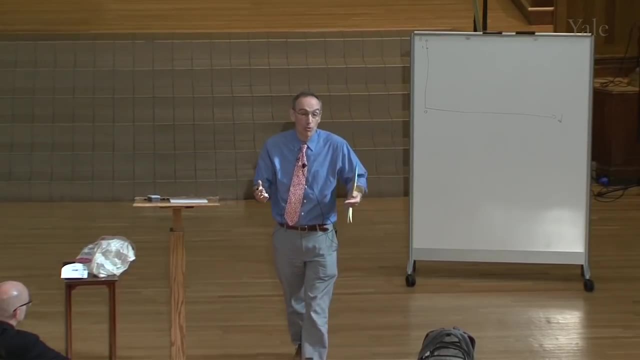 So we're starting far away and getting closer, but I'm going to draw it with distance in the standard way, going left to right, All right. so the second assumption I'm going to make is that, as you get further away, the probability 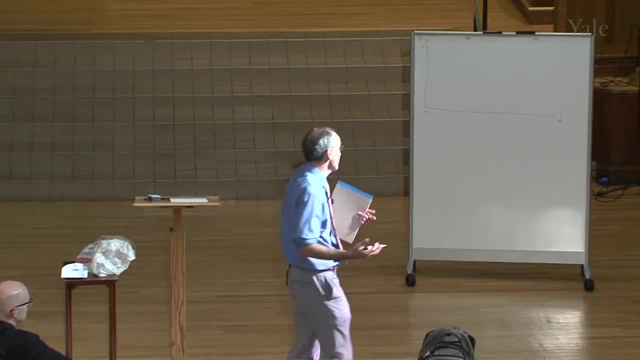 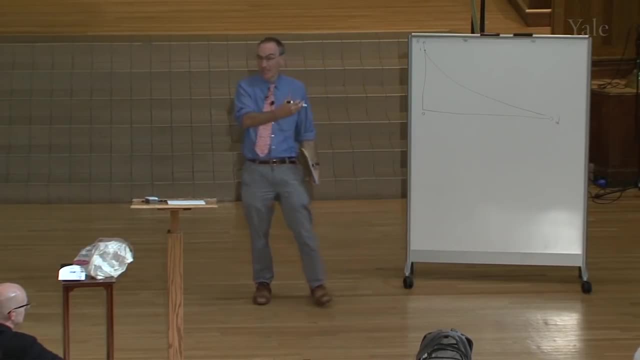 of your hitting goes down, All right. so the further away you are, the less likely you are to hit if you shoot at that distance. So I don't know, it could look like this Same. It doesn't have to be exactly like this, I'm just going to assume. 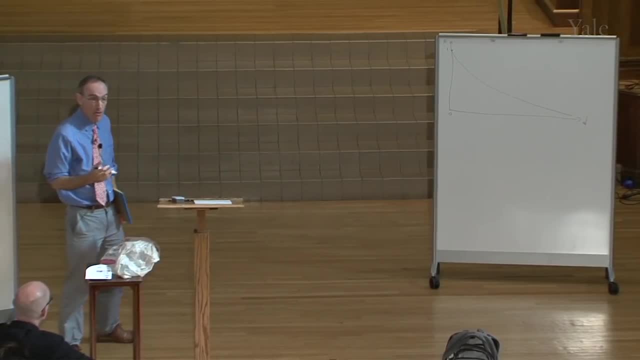 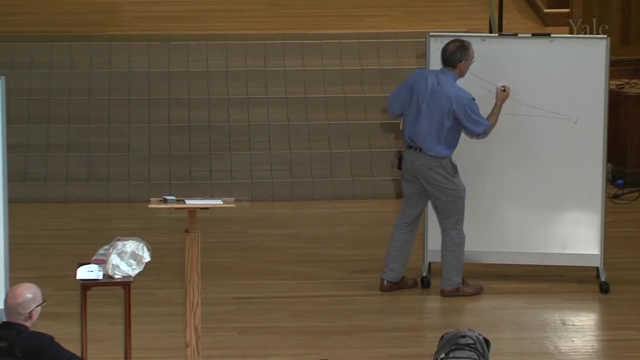 it slopes downwards. Now, I'm not going to assume that both players are the same here, So it could be the case that the other person has a different shape curve. that does this All right, and actually for what I'm going to say today. 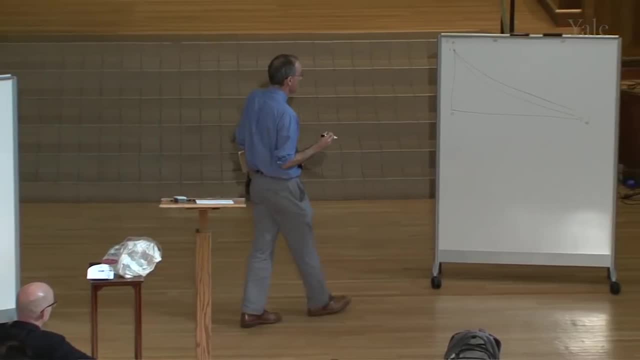 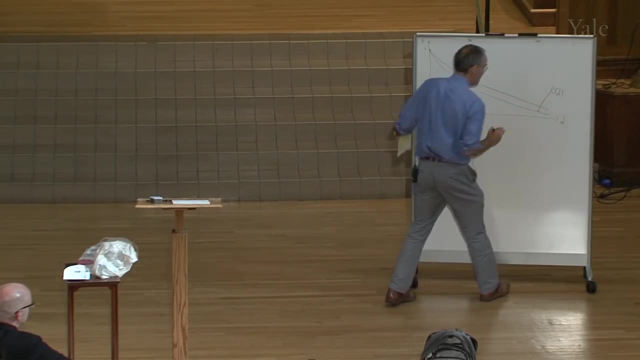 it wouldn't matter if these things crossed, All right, but all I care about is that they're both downward sloping, So in this case, perhaps this one is P1 of D, it's Player 1's probability of hitting, and this is: 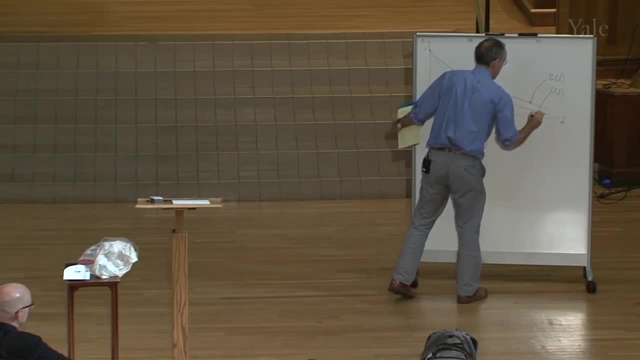 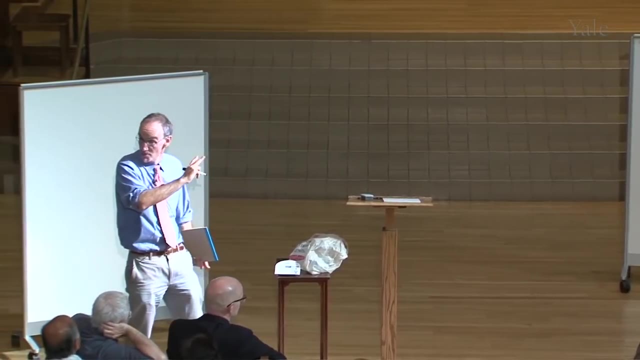 Player 2 of D. All right, so the way I've drawn it, who is the better shot, Player 1 or Player 2? Player 2.. Player 2 is the better shot because at any distance we happen to talk about, were they to shoot at that. 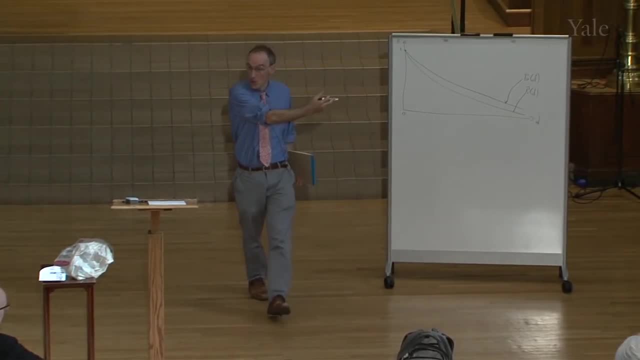 distance, Player 2 has a higher probability of hitting Everyone. okay with that. So Player 2 is the better shot. Now, again, I don't need that assumption. I just need them to be downward sloping. It could be that Player 1 is better. 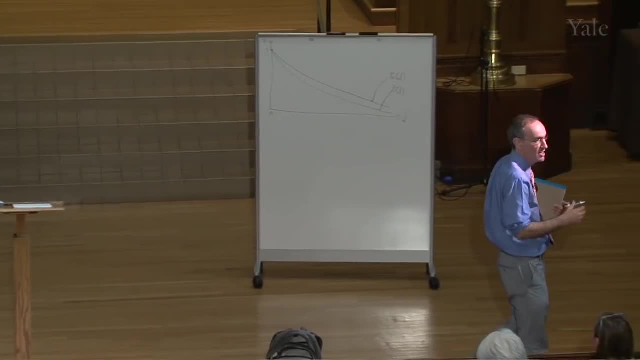 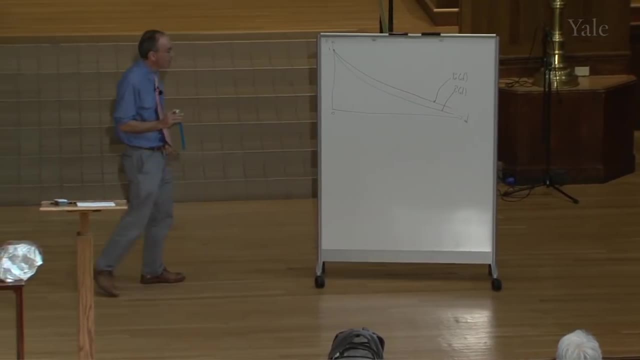 at shooting at close distances and Player 2 is better at shooting at long distances. That's fine, But we'll use this one today. it won't matter. All right, so far I haven't assumed anything particularly difficult. I think Here's the difficult thing. 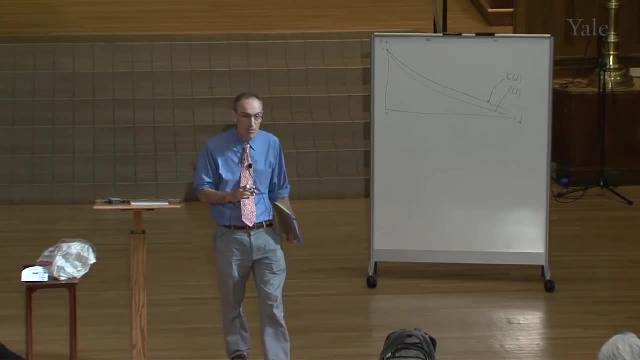 I'm now going to make an assumption that's not real, but I'm going to make this assumption so we can analyze it today in what is most of your first ever game theory lecture. So I'm going to make an assumption. that's not true, but 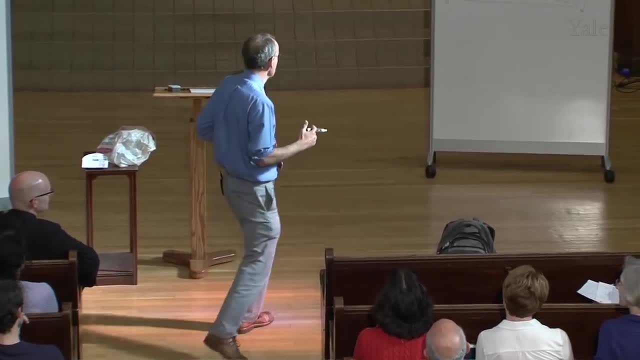 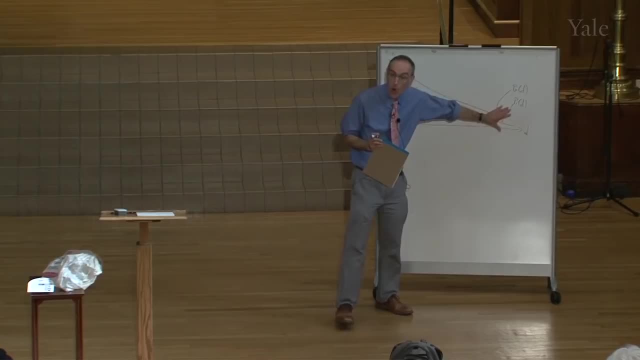 will help us analyze it. It's hard enough even with this assumption. Sometimes it's useful to make a simplifying assumption. I'm going to assume that each player not only knows their own probability of hitting, but they also know the other person's probability of hitting. So I'm going to assume 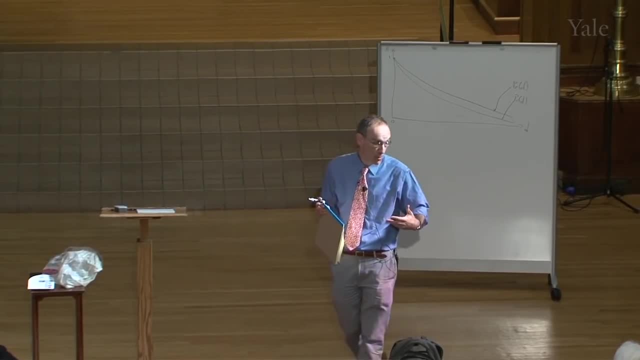 actually I'm going to assume even more than that. I'm going to assume that these are commonly known. So I'm going to assume that Player 1 knows their own ability, they know the other person's ability and they know that the other person knows their ability, and so on and so forth. 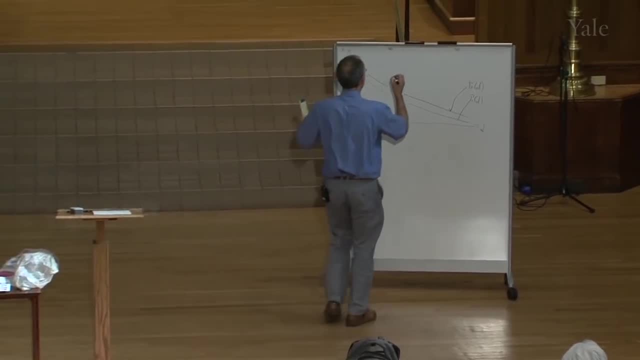 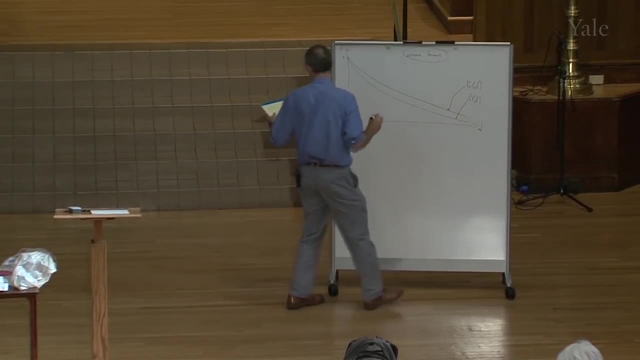 So I'm going to assume that's all known. So that's a big assumption, but it's enough for today to solve it. I'm going to assume that these are known. Now imagine it in fact is the case that one of these players 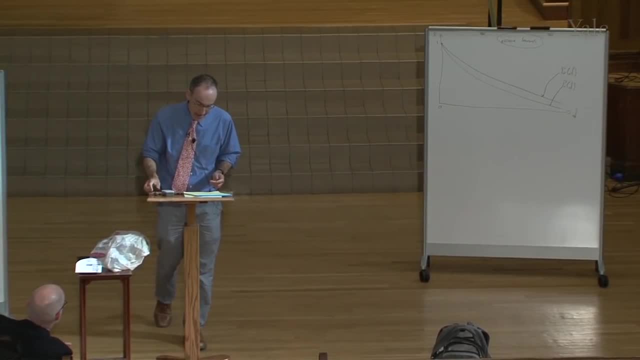 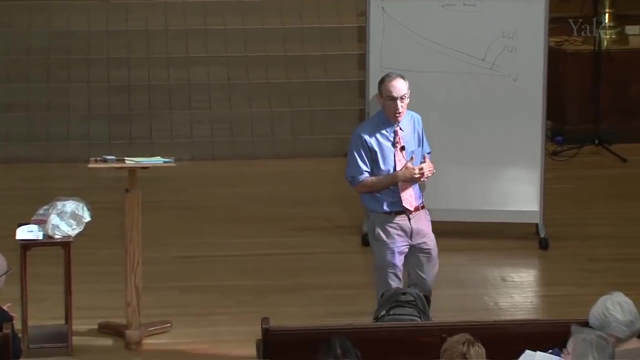 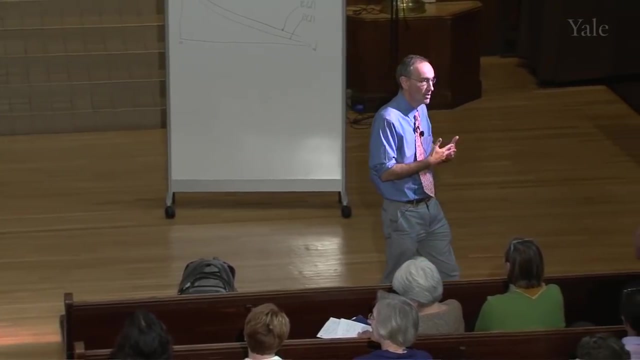 is known to be a better shot than the other player. Let's ask ourselves a question: Who should shoot first, The known better shot or the known less good shot? Who should shoot first, The known better shot or the known less good shot? 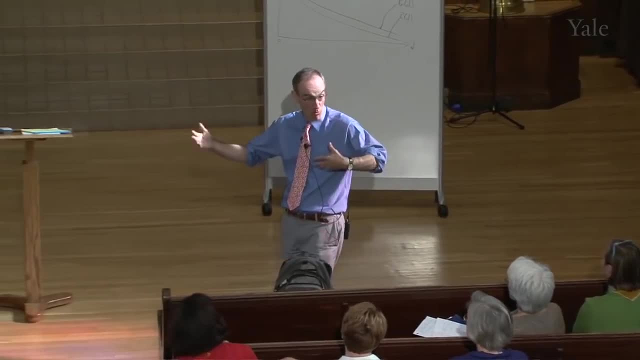 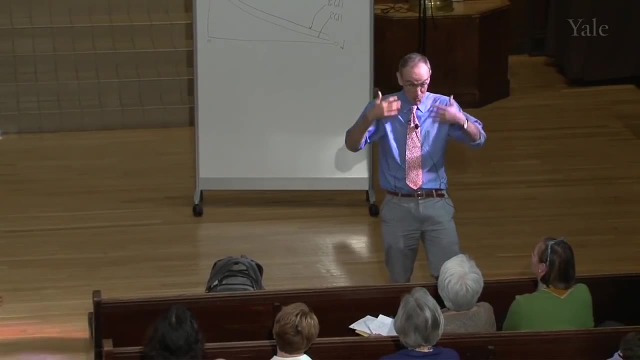 Well, here we are playing the game. Should, meaning normatively- put them in their shoes. when you're in that person's shoes, from that person's point of view, who do you think should shoot first? Who thinks the better shot should shoot first? 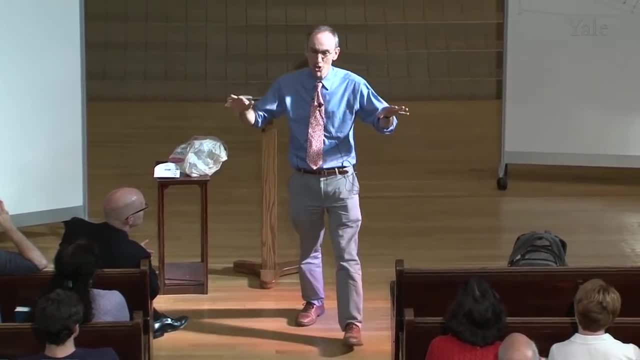 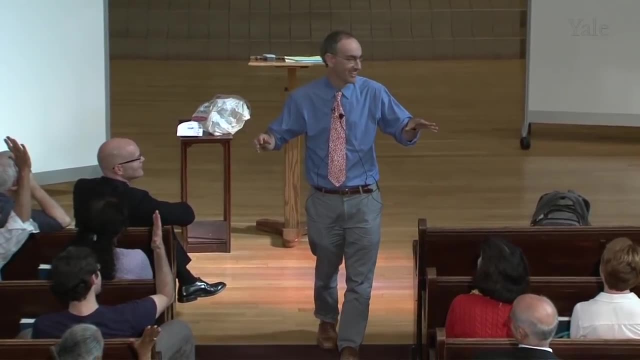 So hang on, let's have a poll. Who thinks the better shot should shoot first? Raise your hand. Who thinks the less good shot should shoot first? Who is hedging their bets? All right, so let me try and talk it through. 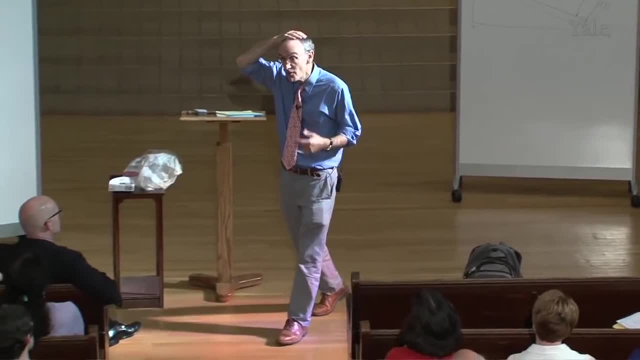 So the people- I'm guessing the people who are thinking the better shot should shoot first, they're thinking something like this: They say, well, the better shot has a better shot of hitting the other person at this distance. So you compare two people. 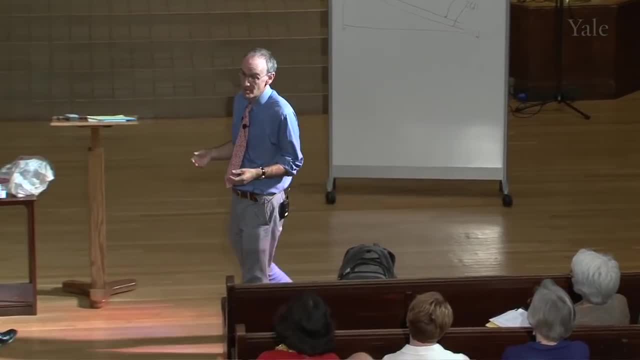 at an equal distance, the person who's more likely to hit is the better shot, so the better shot should shoot first. I don't know exactly where they should shoot, but the point at which they should shoot is earlier, since they're the better shot. 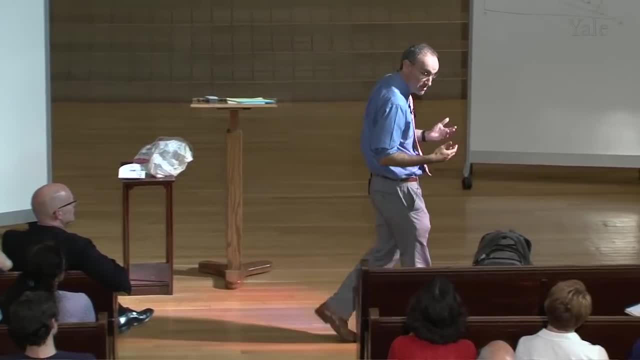 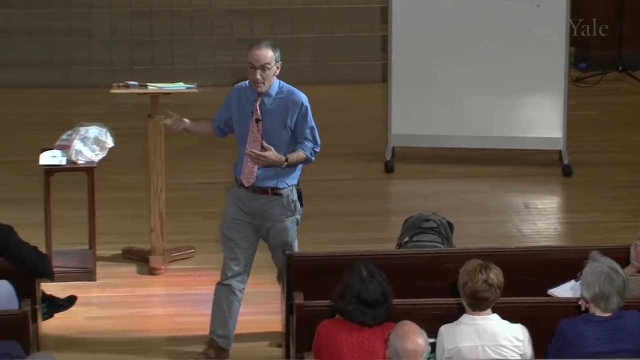 All right. and then the people on the other side- I'm guessing, tell me- are thinking something like this. They're saying: well, the other guy's a better shot than me, so I better shoot first to preempt him from shooting me. 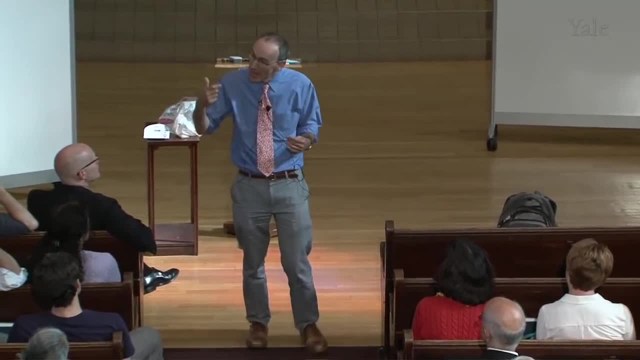 Is that right And we could take this further, Then the better shot could think: hang on a second. I know this is all known right, so I know the other guy knows that I'm the better shot and therefore thinks I'm going to. 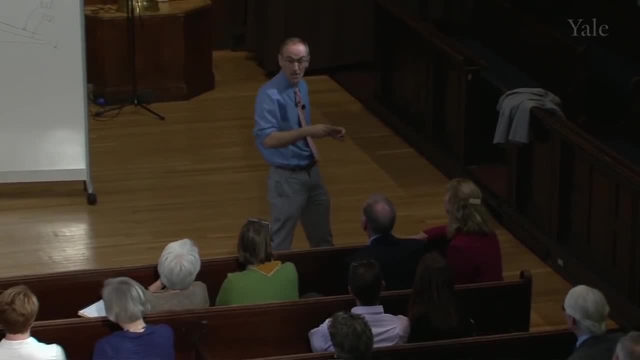 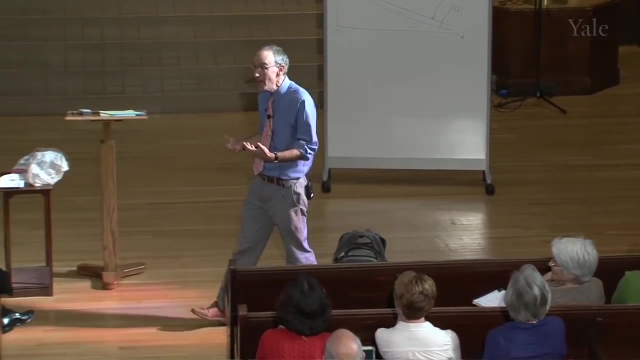 shoot first and therefore he's going to shoot first to preempt me shooting him. so maybe I should move even earlier to preempt him from trying to preempt me. All right, and we could go on with this discussion for a while, and I think once we've 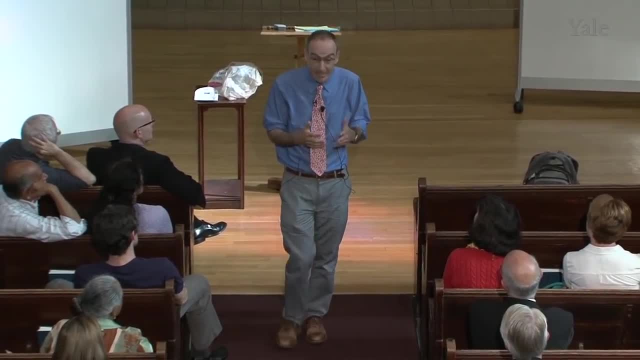 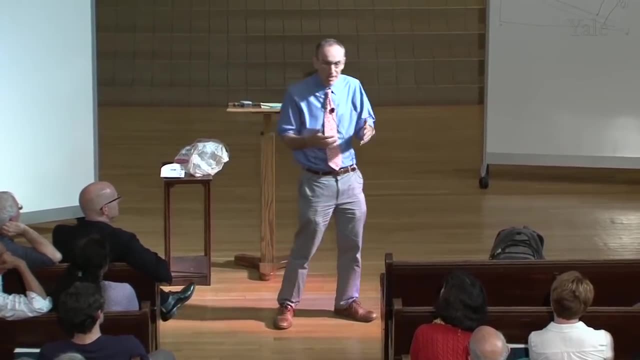 opened up this particular Pandora's box, you can see it's not going to be that easy right. It's not obvious who should shoot first. At first it seems obvious got to be the better shot, but it's not obvious at all. 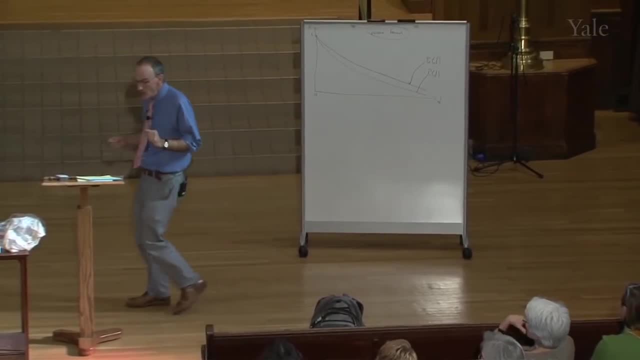 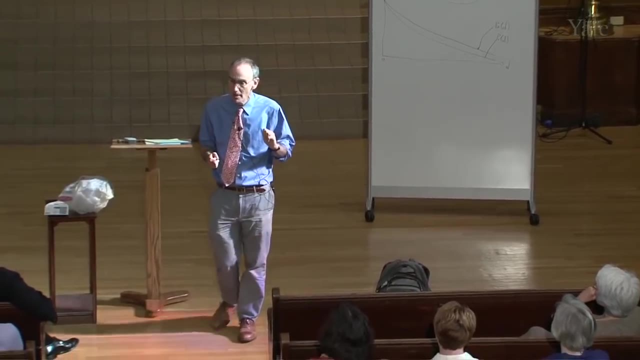 All right. so here's what we're going to do: We are going to figure- and I'm going to emphasize that word, we again. We are going to figure out who should shoot and we are going to solve this exactly. We're going to figure out exactly. 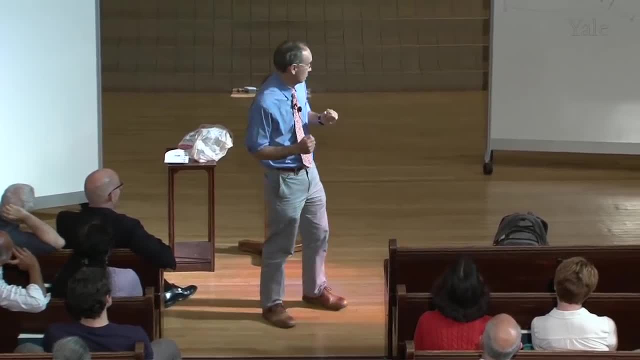 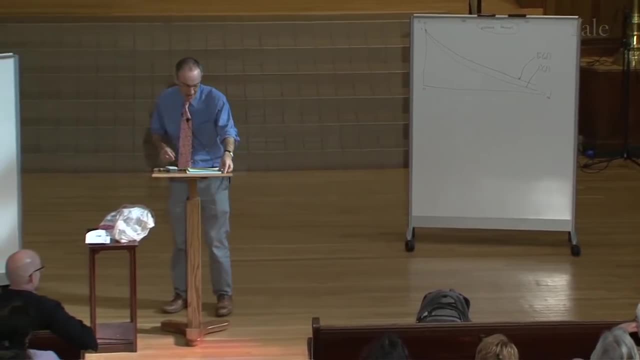 when they should shoot. All right, so we're going to figure that out For the physicists and mathematicians in the room. you can see some. You know the answer already, but pretend you don't. All right, so all right, On the way. 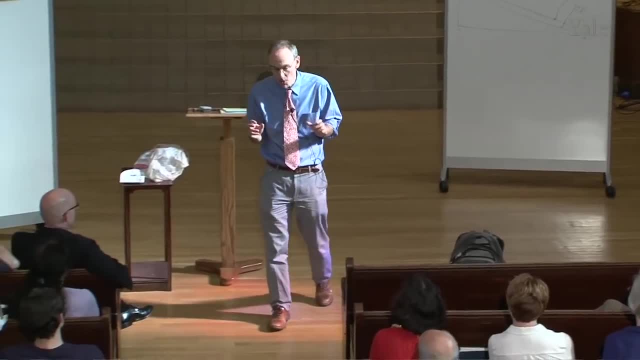 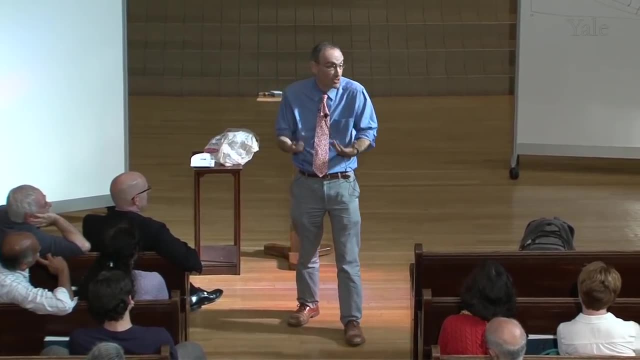 I'm going to point out two ideas- I hope I remember to do this- that are more general than just this game. All right, so we're going to work through this game, but since I want to use this as an illustration for ideas you might use elsewhere in life, 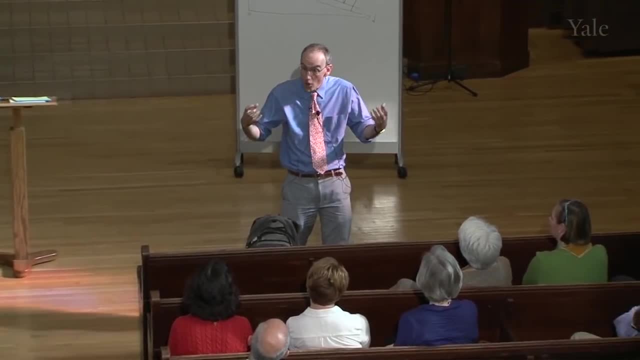 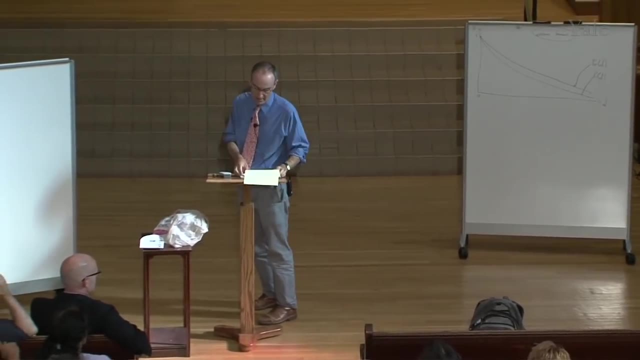 or when you're playing games or wherever. I'm going to try and draw out two larger ideas as kind of take-home things for you. All right, so remind me to do that if I forget. Okay, Oh look, I brought Pushkin with me. 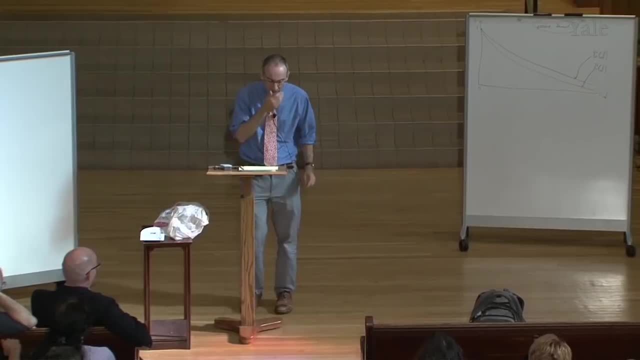 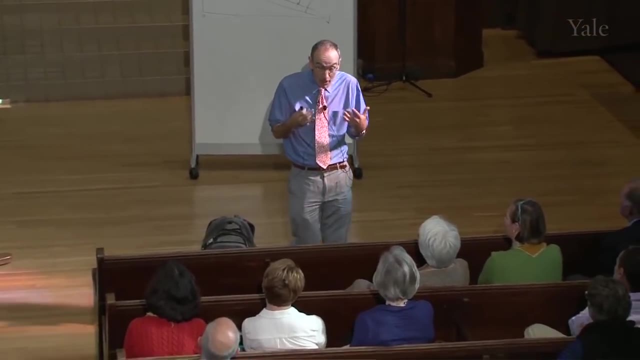 Somebody can have a copy. I was going to read it out, but I guess we haven't got time. All right, So to do this, we're going to do this. so one of the things we're going to learn- this is not one of my big general ideas. 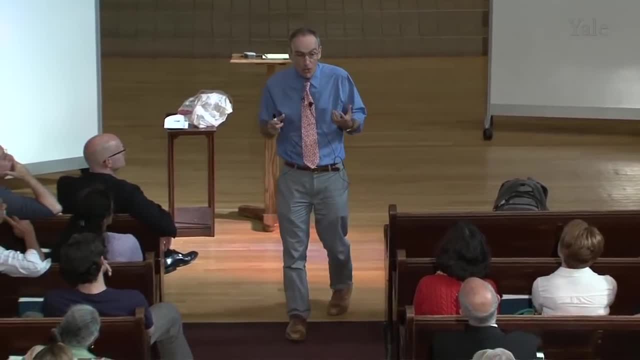 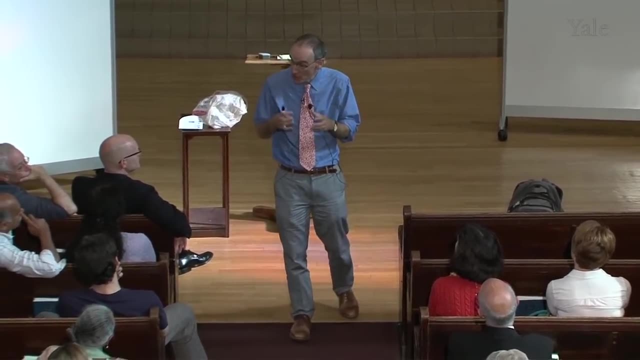 it isn't a bad one. one of the things we should learn is, when you have a difficult problem like this, it's a good idea to try to break it down into some smaller problems, because the whole problem just seems unmanageable. So what I'm going to do is I'm going to break it down. 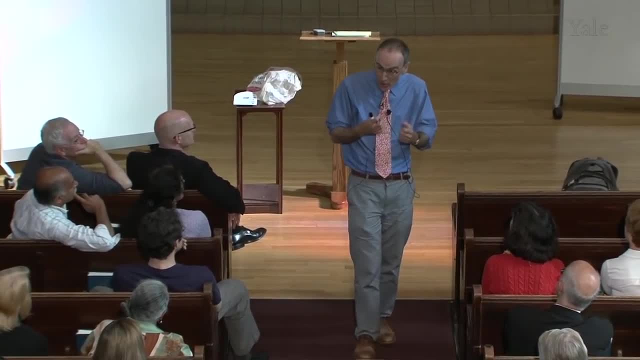 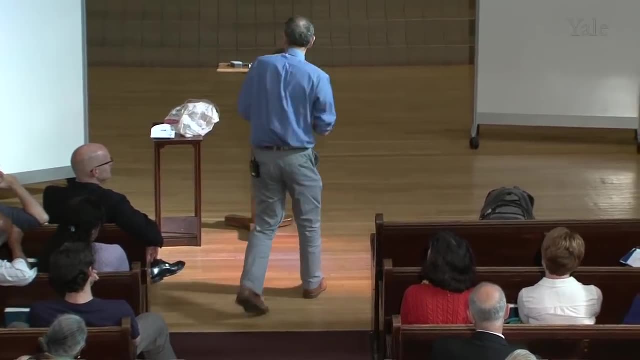 and see if we can figure out what to do in two kind of easy pieces and then use those pieces as building blocks to try and get the general answer. Okay, that's going to be my strategy here. All right, so the first building block. 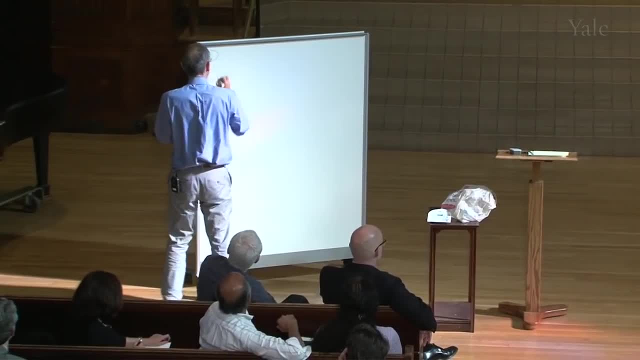 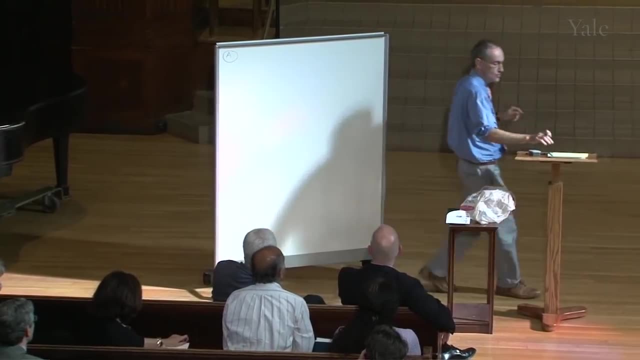 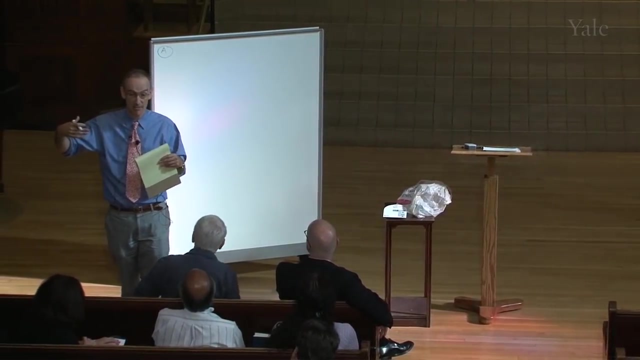 we'll call it A Building block A, And building block A is going to be a question, All right. so for both these building blocks, I'm going to assume. I'm going to assume that no one has shot yet, All right. so, assuming no one has, 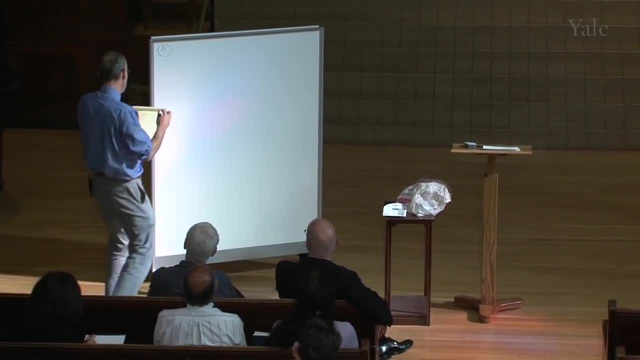 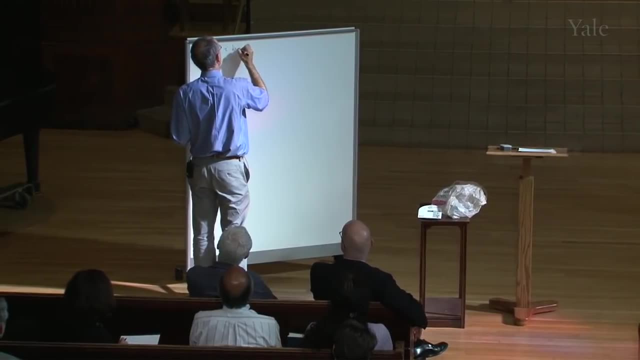 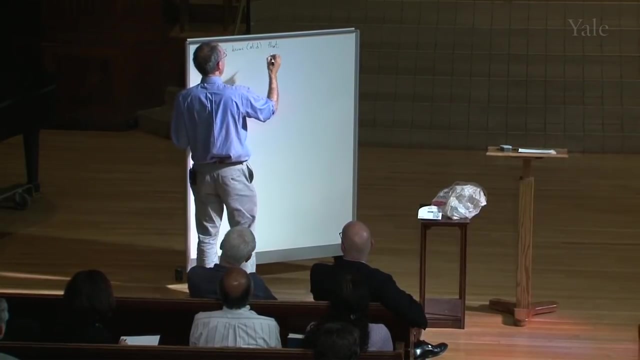 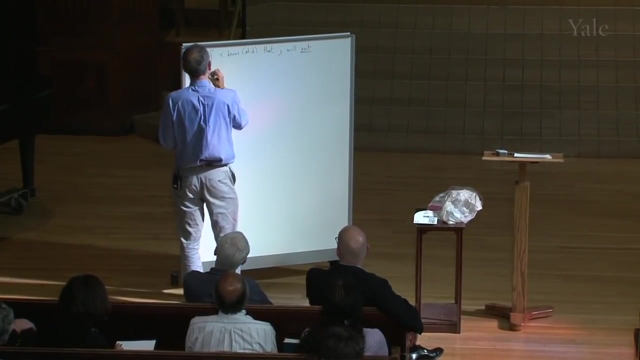 I could write that at the top, assuming no one has shot yet, then if player I knows at distance D say there, they are at D, that the other person- let's call the other person- J, that J will not shoot. 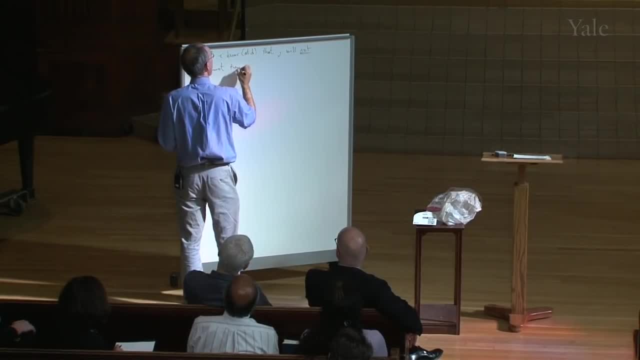 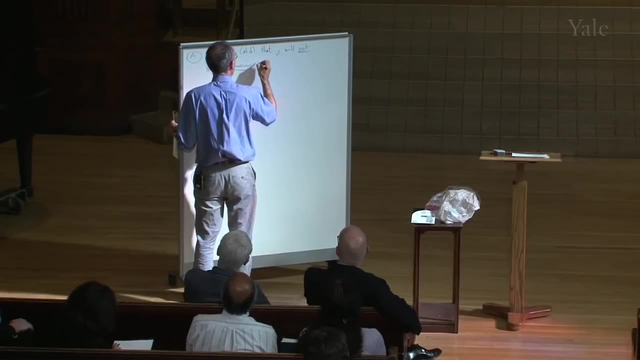 or throw, if you prefer, next turn. Can I use the word tomorrow for next turn? It'll save us having to write next turn every time. We'll not shoot tomorrow when it's player J's turn, Then what? So you're player I. 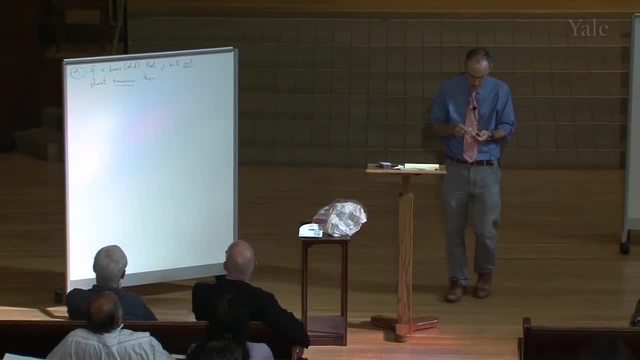 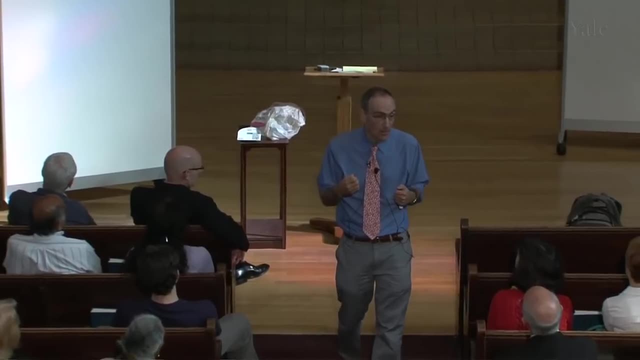 let's say you're Robert and you've got your sponge, and James still has his sponge and it's your turn and for some reason, you know, you, Robert, know that James is not going to throw next turn, assuming that no one threw it. 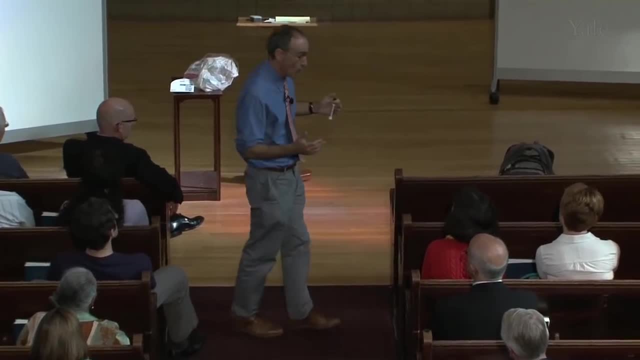 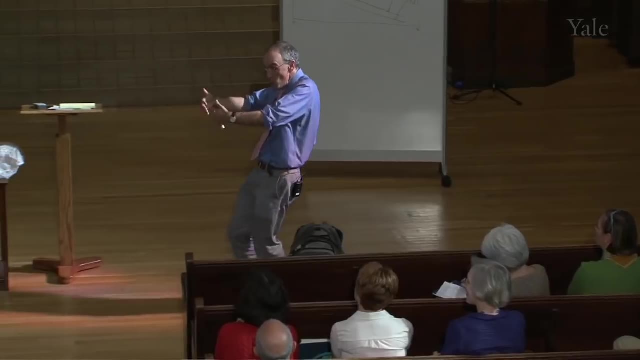 Should you throw now or not? You should not throw right. Why should you not throw now? In that circumstance, You've got a better chance next time. right, Because if you knew that the other guy is not going to shoot next turn tomorrow. 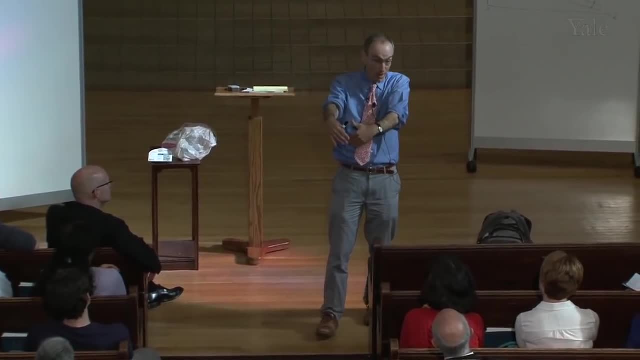 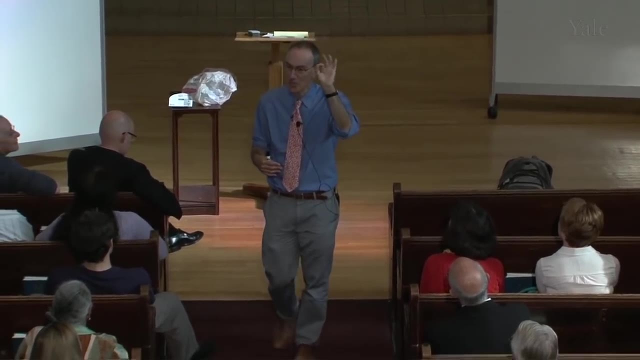 then you're going to get a better shot the day after tomorrow Doesn't mean you should necessarily shoot the day after tomorrow, but you're certainly shooting the day after tomorrow is better than shooting now, Is that right? Everyone okay with that? This is meant to be the easy fact. 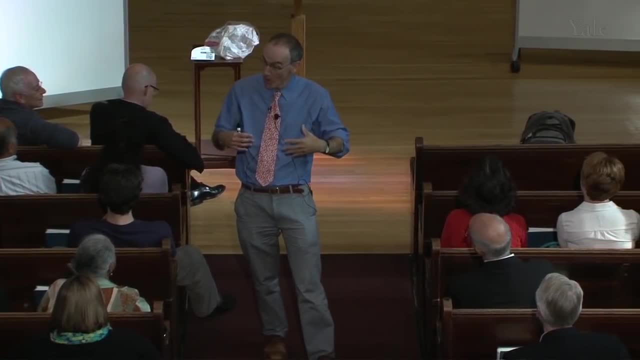 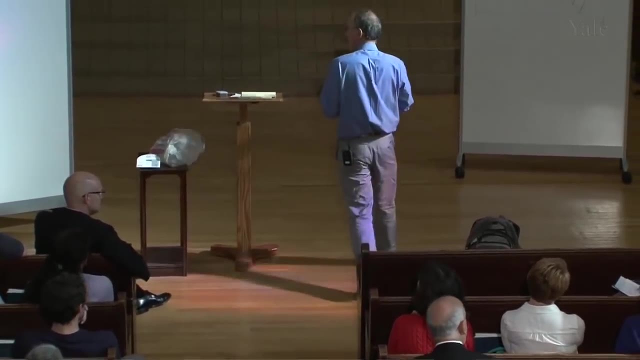 This is good, yep, So I know the other person's not going to shoot tomorrow, but I should not shoot now. I should wait until the day after tomorrow. We're good, David, we're good on that. Okay, I'm checking, because he's my teacher. 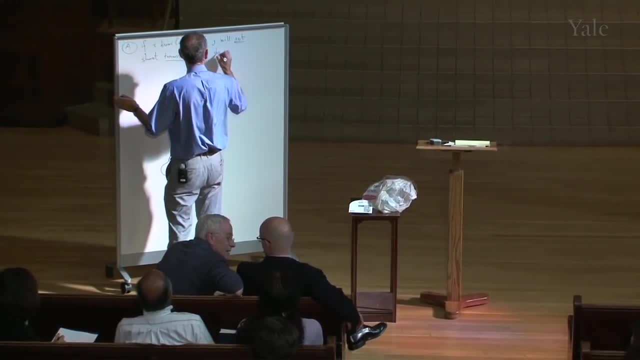 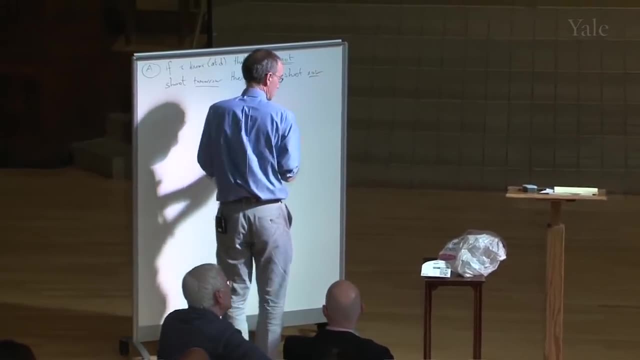 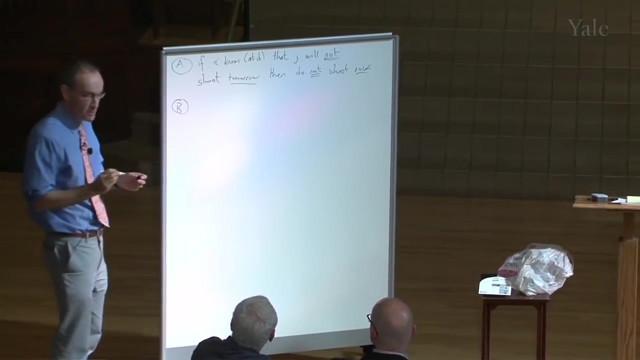 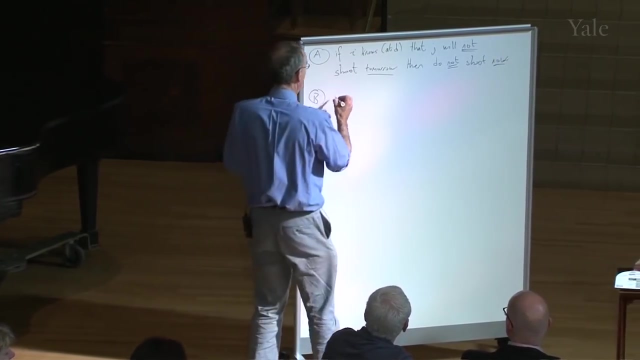 Alright, Then do not shoot, Alright. Alright, so that was Fact A, So Fact B. you can kind of guess what it's going to say. it's going to say, assuming no one has shot yet. suppose that I knows. 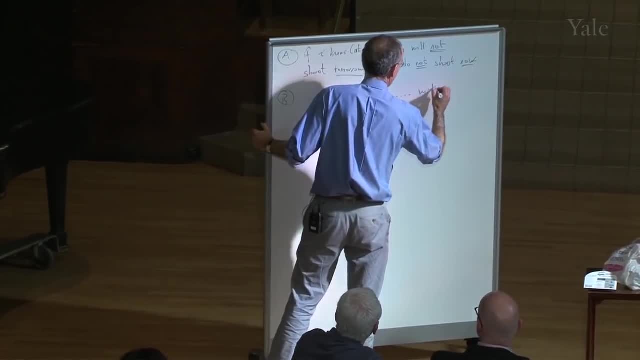 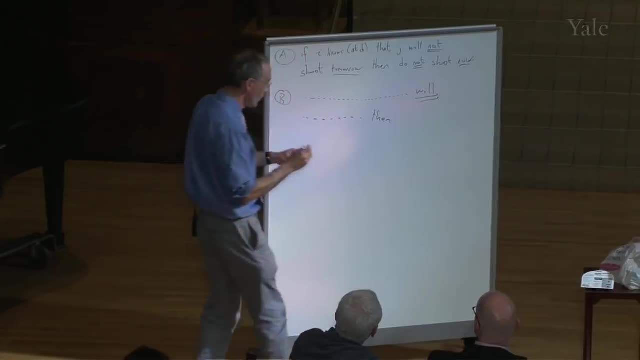 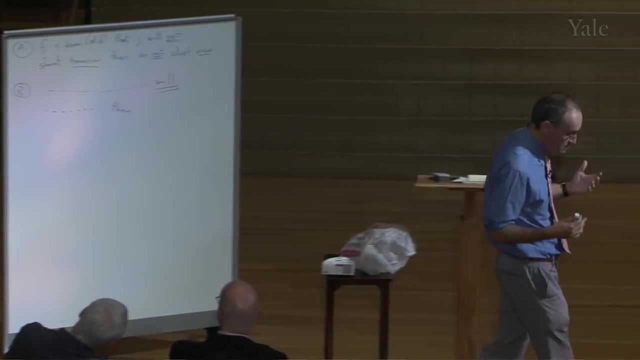 at distance d that J will shoot tomorrow. Same thing with will, not replacing will. So again, suppose you're Robert. no one's shot their sponge yet, no one's thrown their sponge and you, for whatever reason, you know that if you don't shoot now, 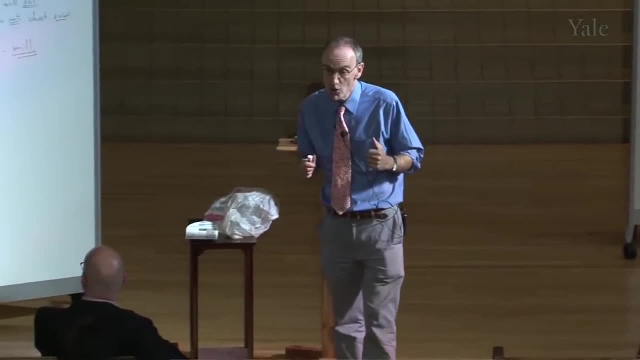 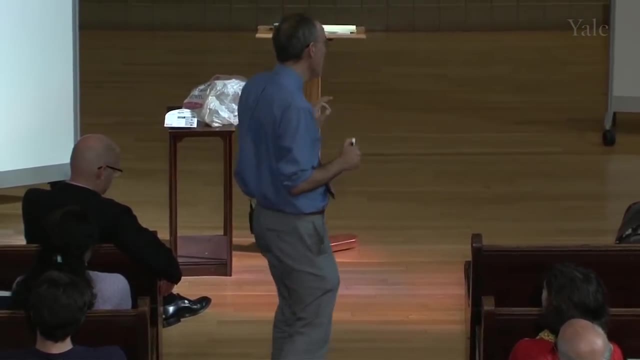 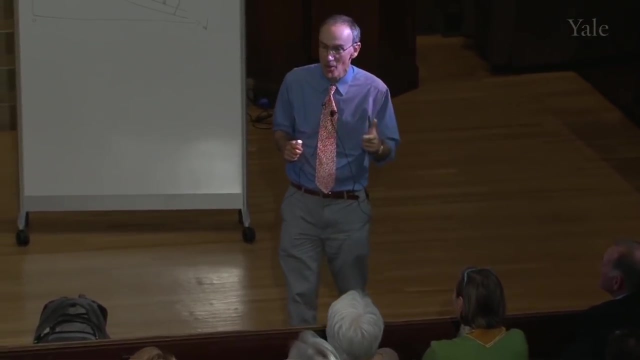 James is going to shoot tomorrow. what should you do? Alright, it depends, it depends, it does indeed depend. What does it depend on? Depends on distance. What else does it depend on? Okay, so, depending on distance and the reason. 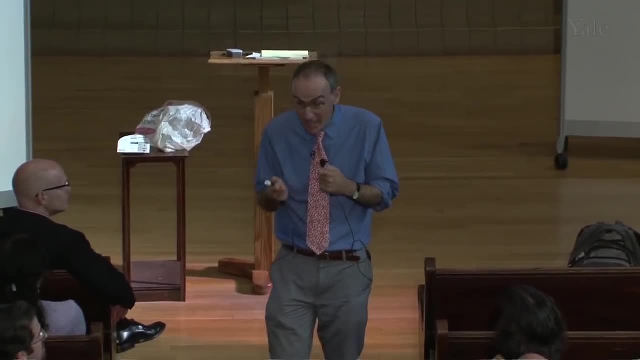 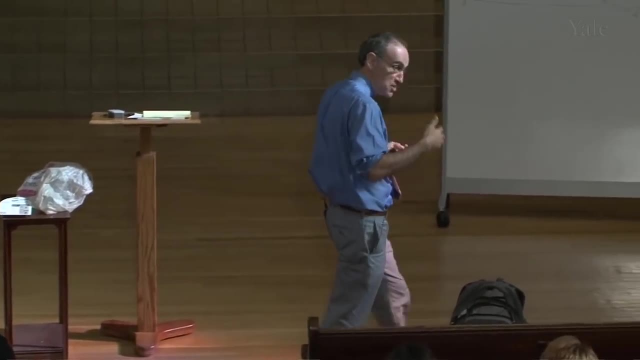 it depends on distance is? it depends on the probabilities, and it indeed depends on who's the better shot. alright, so it's going to depend on all those things. it's going to be more precise. So that's right, it does depend on distance. it depends on distance. 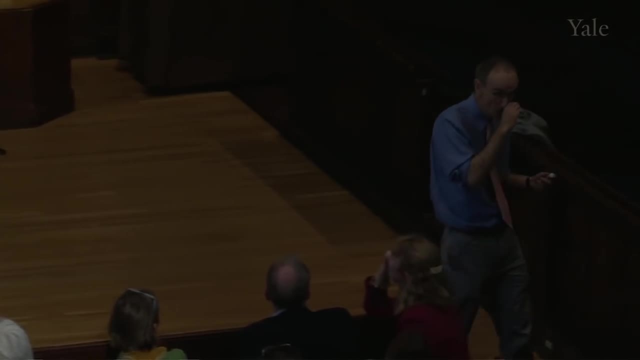 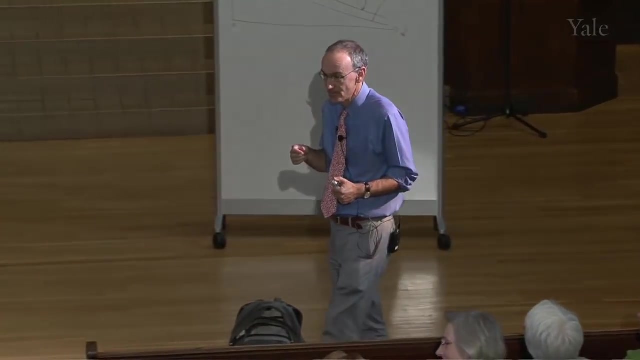 because the probabilities depend on distance and the probabilities themselves depend on who's the better shot. so it's right, it depends on those things. Can we be more precise? What's the probability that he'll hit versus the probability you'll hit now versus 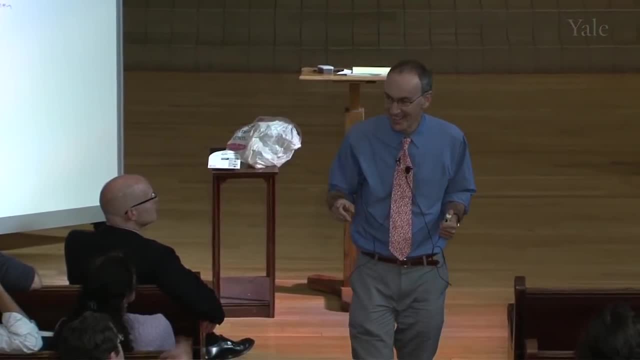 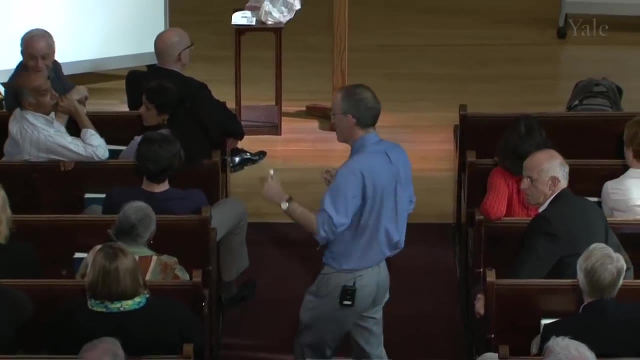 if you get two steps forward, Close. Well, I guess you're 100% if he misses. so Second, He's an engineer. shouldn't lie to the engineers. yeah, that's right. so okay, here's the answer. that's right. 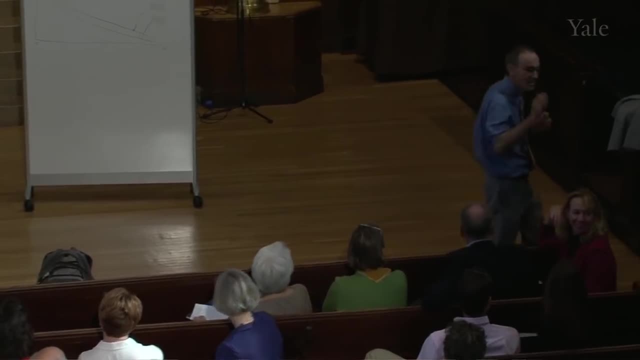 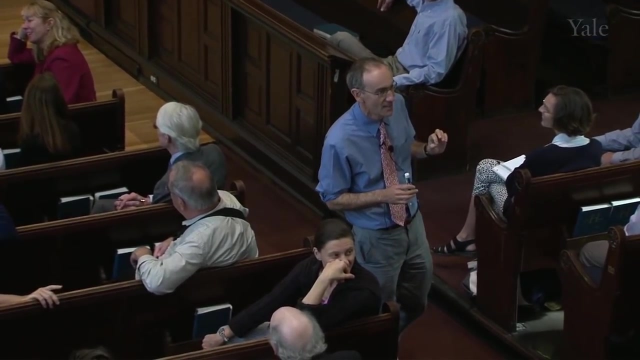 so what do you have to compare? You have to get Doug. yeah, go ahead When you fill those sponges with water and squeeze them out. how much does it compare to what that did, to the weight of the sponge? Do we need to calculate that as the weight? 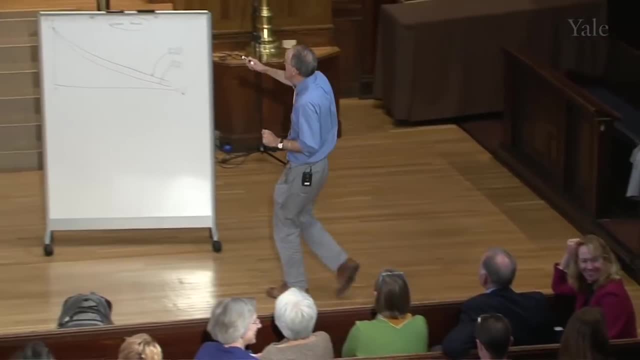 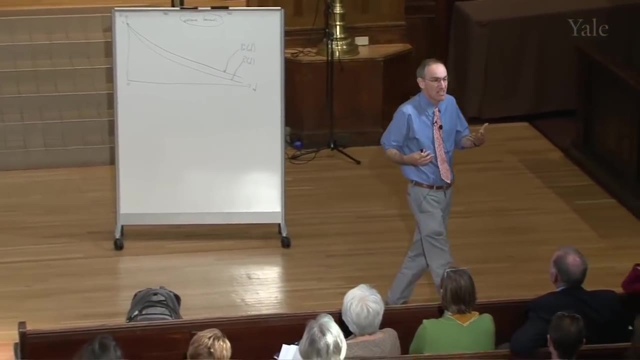 True, that's a good point actually, but notice that I've assumed. I've assumed that I've done that here. so the assumption that you know these curves means you really do know what these probabilities are. so, in some sense, even though we didn't play it that way, 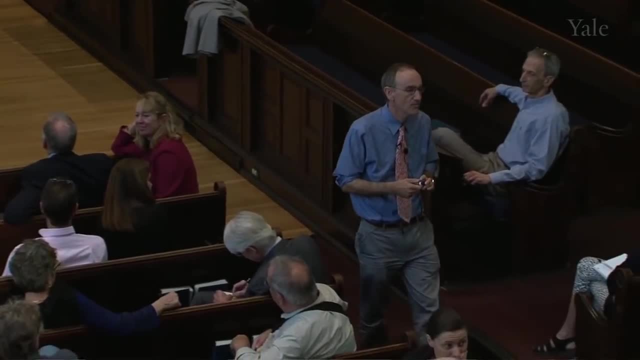 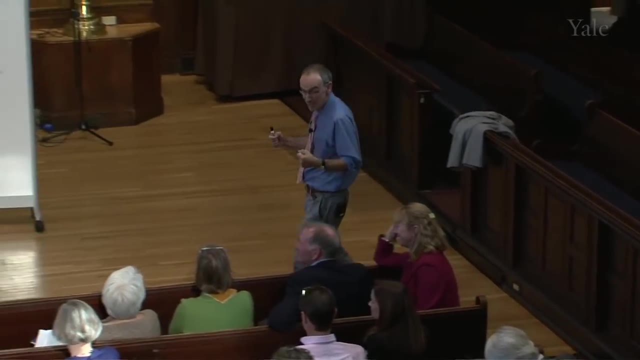 we've assumed that you know the weight of the sponge. Does this game calculate that as opposed to the sponge? So here's our difference between reality and the assumption. so in reality, James probably doesn't know his own ability or the weight of the sponge. 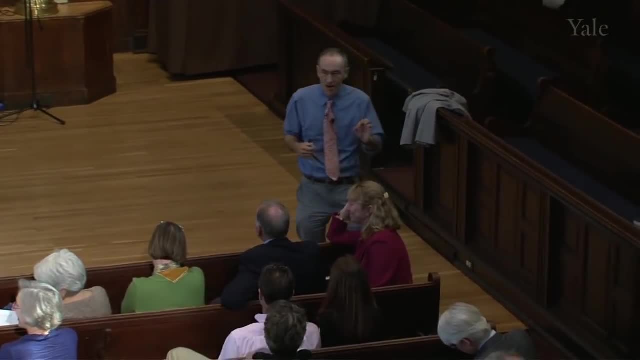 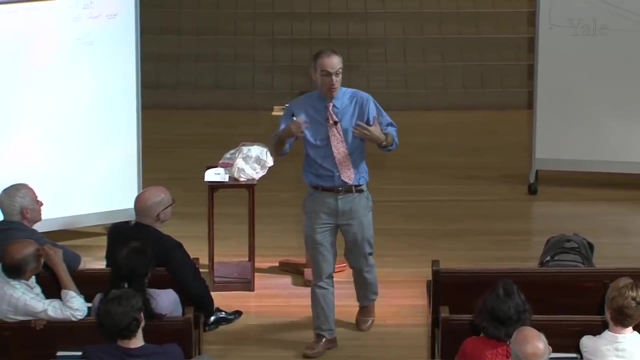 but we're going to assume for today that he does, just to keep things simple. So let's come back to that. it depends again. So what does it depend on If I throw now? let's state the question again before I answer it. the question is: 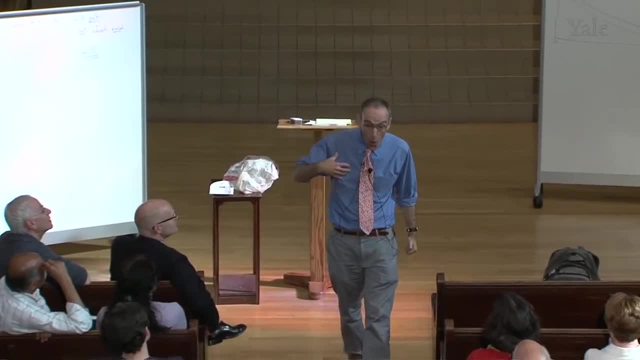 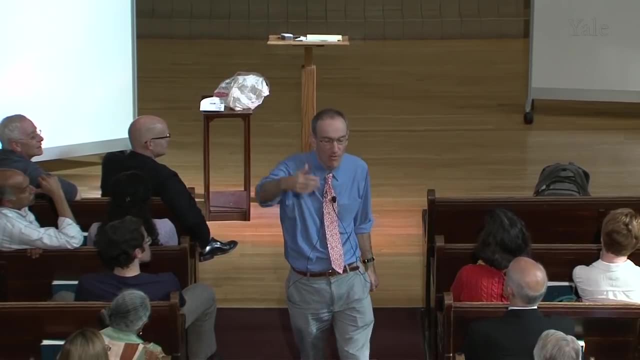 if no one has thrown yet and if I know that you are going to throw tomorrow if I don't throw today, sorry, I know that you are going to throw tomorrow. if I don't throw today, what should I do? That was the question. 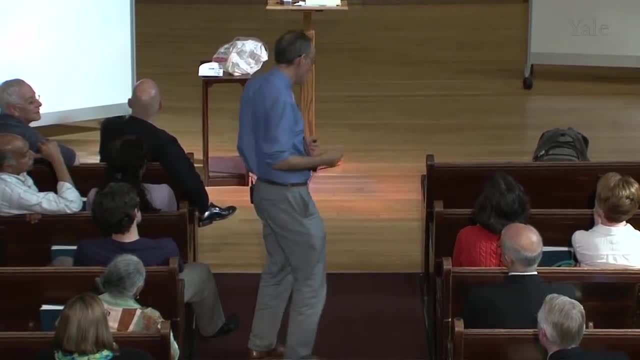 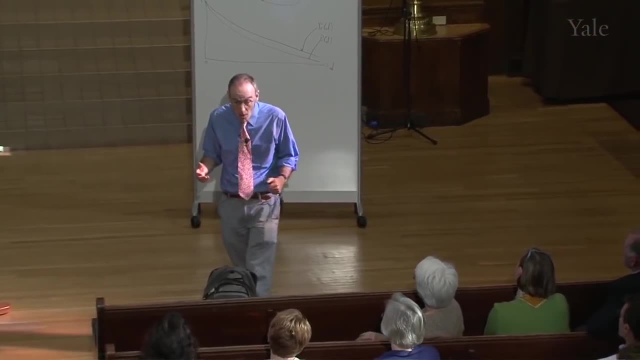 And the answer was: it depends. and then it's: what does it depend on? What do we need to compare? We need to compare what happens if I throw. If I throw, then my probability of winning the game is the probability that I. 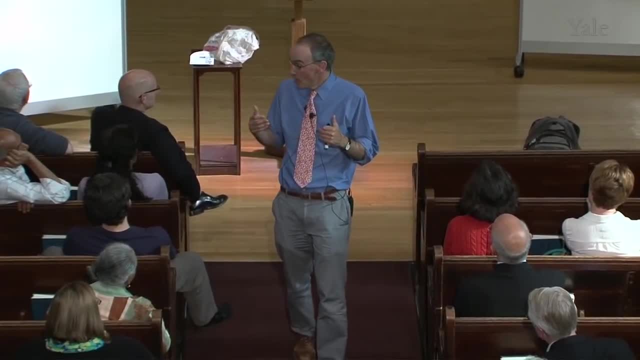 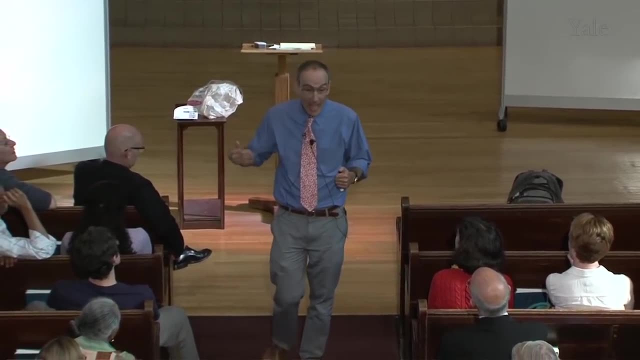 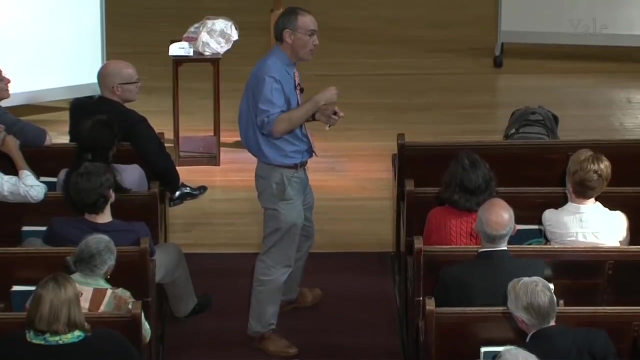 hit the other person, Alright. If I wait, knowing that he's going to shoot me tomorrow or shoot at me tomorrow, then my probability of winning the game is the probability that he misses tomorrow. Is that right? So I have to compare the probability. 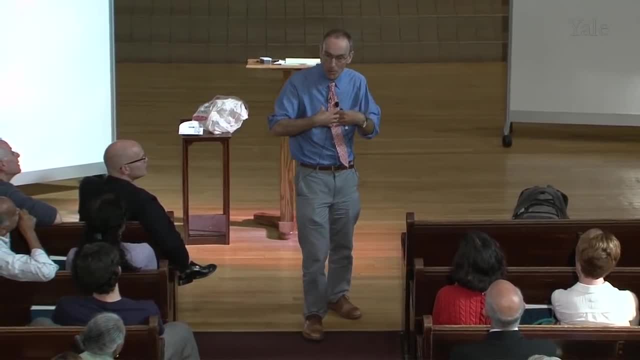 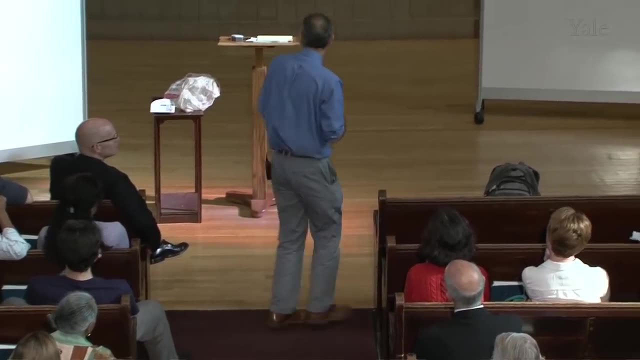 of my hitting if I throw today, with the probability of him missing if I leave it and let him throw tomorrow. Does that make sense? I need to compare apples with apples or oranges with oranges. so the answer is then: shoot or throw. 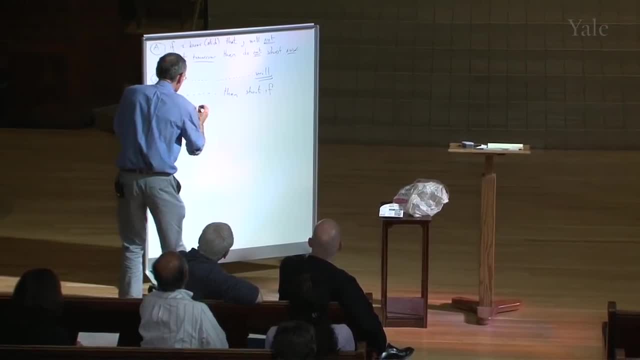 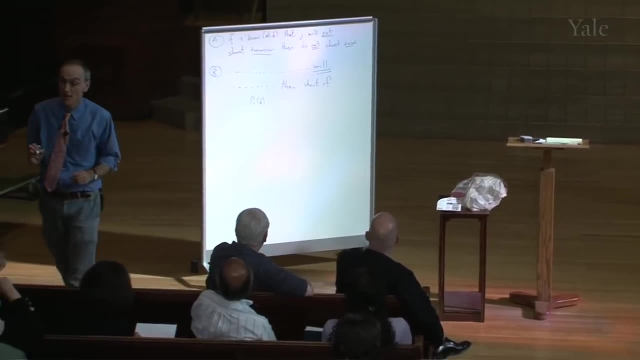 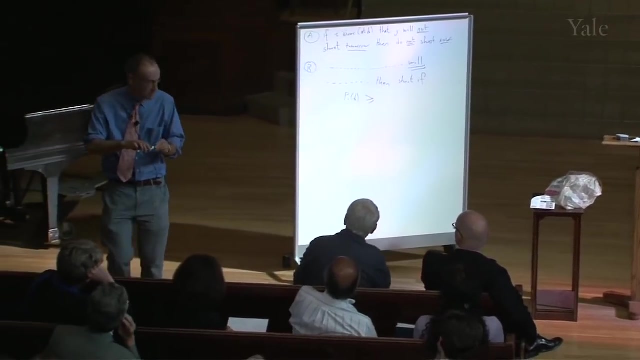 shoot, if alright, so let's use our notation P-I D. that's the probability that I hit. if I throw today is bigger, we'll make it bigger than the equal. let's not worry about the equals for now. 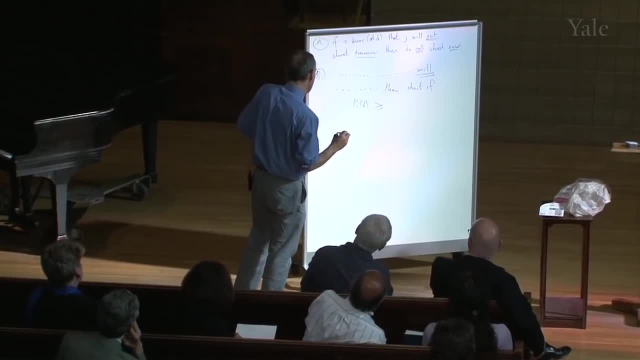 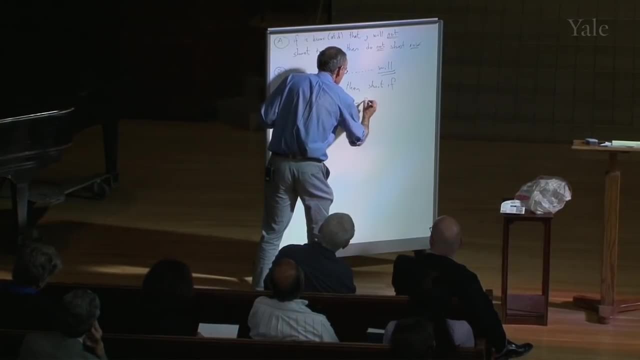 it doesn't really matter, so we'll make it bigger than the equals. as for today, P-I D is greater than or equal to the probability that he misses tomorrow, and that's one minus P, J D minus one, because we'll be closer together tomorrow. 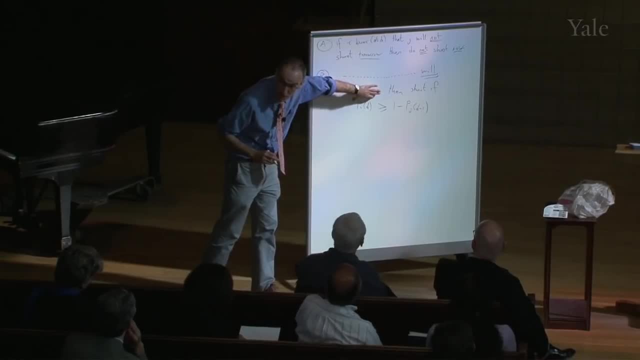 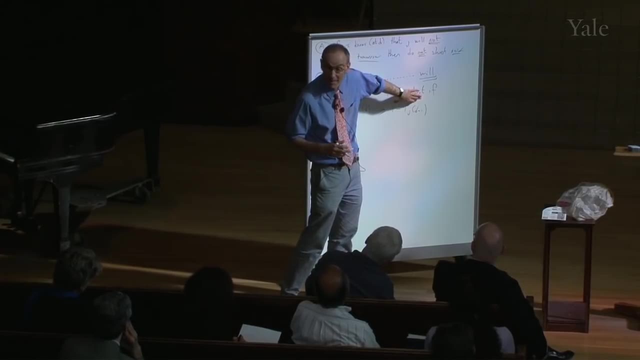 Alright, so this is the probability that I hit today if I shoot, and this is the probability that if I don't shoot and he then shoots at me, this is the probability that he misses tomorrow, Everyone. okay, that one minus makes it the probability of him missing, and D minus. 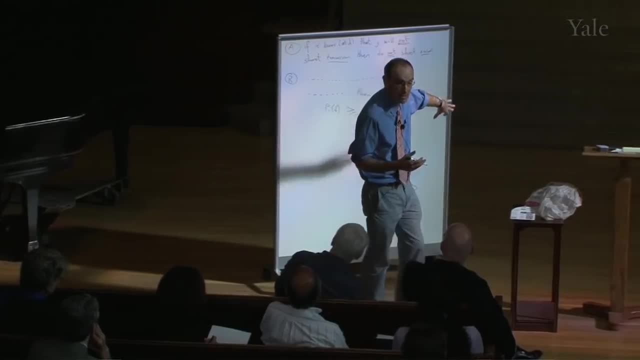 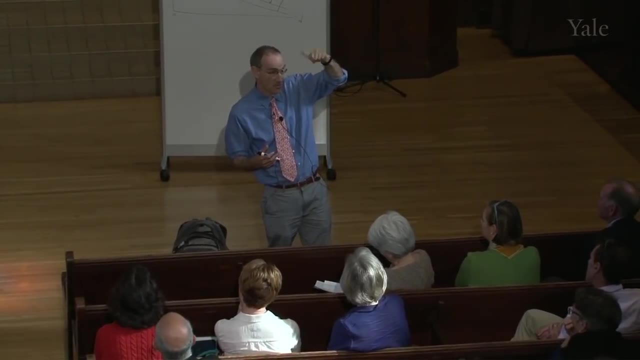 one because we're closer together tomorrow. Alright, everyone okay with that. Yeah, Somebody can wave. if they're not, it's okay. should I do it again? Good, Good, or do it again, Yes, On, Okay. so this is the probability of 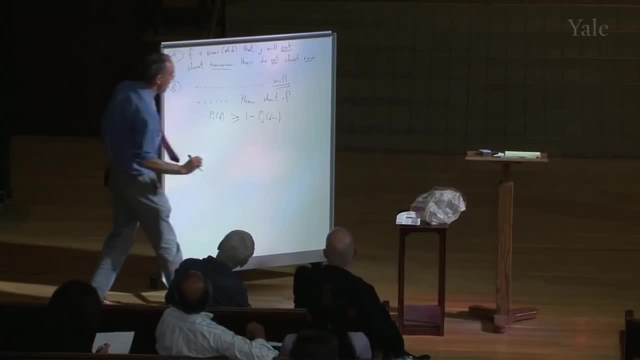 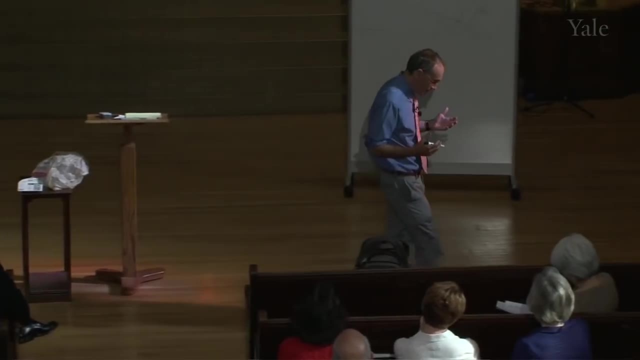 winning by my hitting and this is the probability of me winning by his missing. Okay, now I'm actually going to do some real math, and I know that some of you are not. you know, didn't excel in math in college and are pretty math nervous. 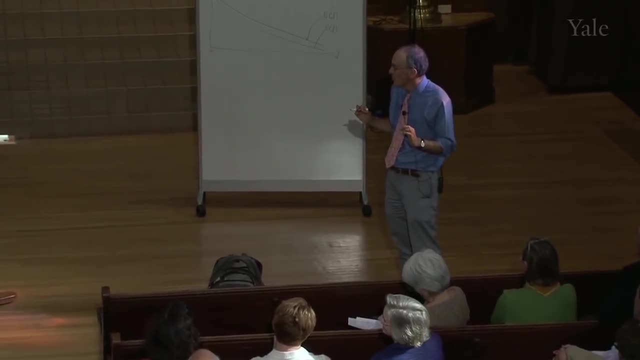 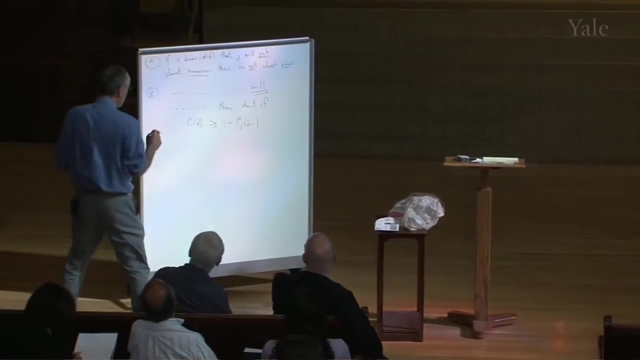 so this is the only actual math I'm going to do. so those people who are nervous, can you please hold onto your seats underneath the cushions, just for a second. I'm going to add, I'm going to add P-J D minus one to both sides of this thing. 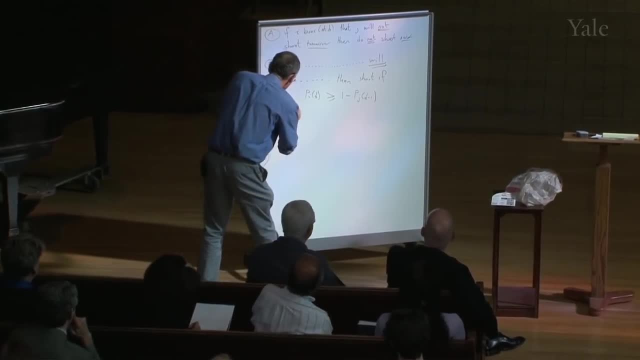 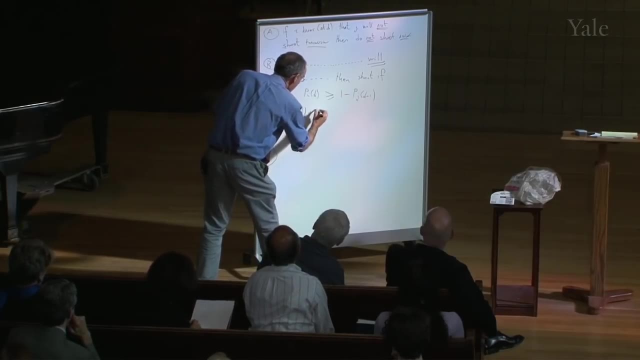 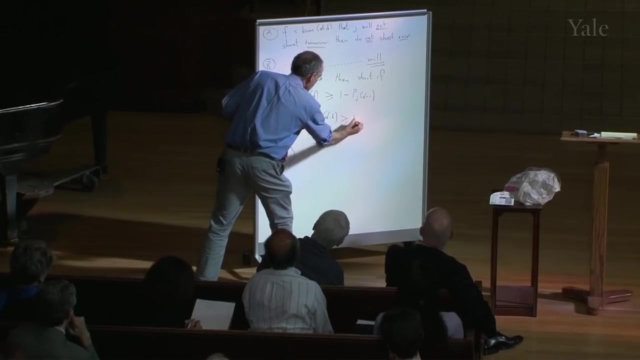 Alright, okay, that's the only math I'm going to do here. Okay, so this is the same saying: shoot if, and only if, P-I D plus P-J D minus one is great and equal to one. Okay, everyone okay with that bit of math. 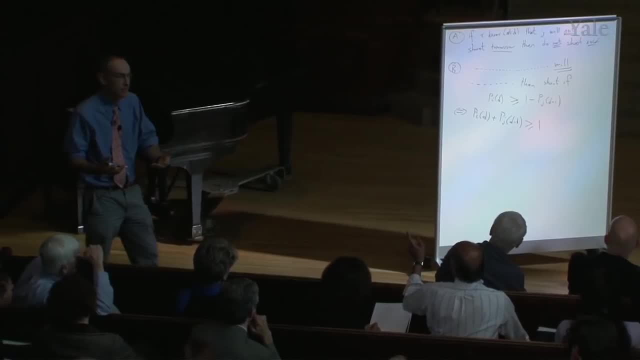 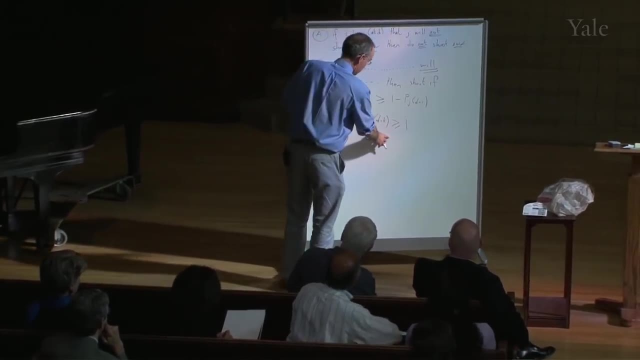 I've just added something to both sides of an inequality. Yeah, I know the physicists are okay with that. I mean everyone else. Is that going to be too hard to see? should I drag it back? Alright, let's, Can people? 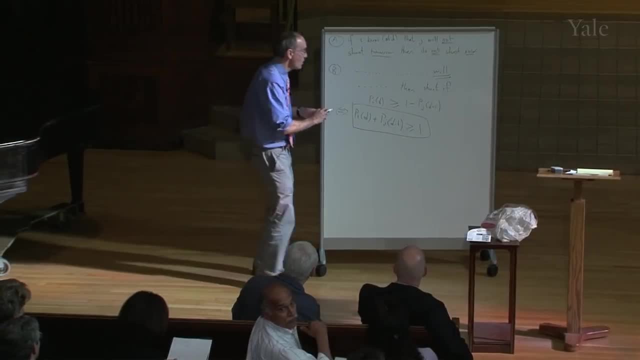 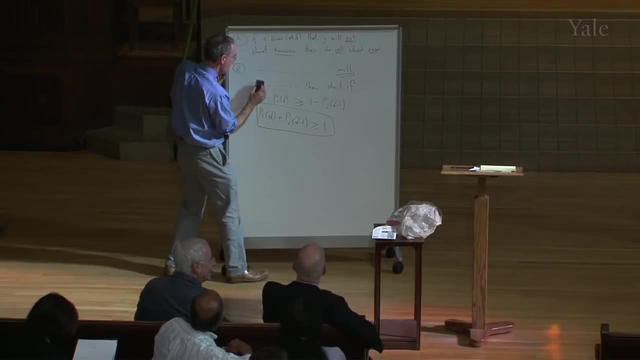 Charles, can you see that Up? it needs to be higher. Okay, we're going to raise it up. How much higher? If it was here, it would be okay. Okay, so we'll just rewrite it, Da-da-dum. 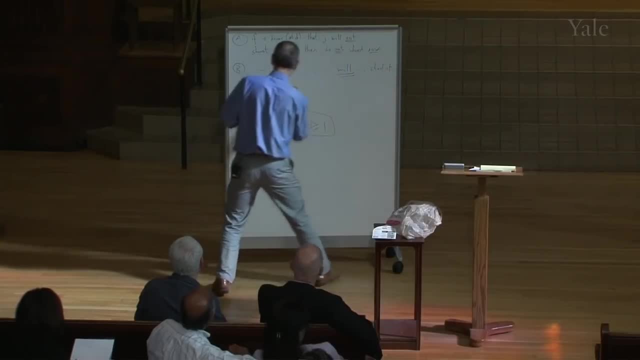 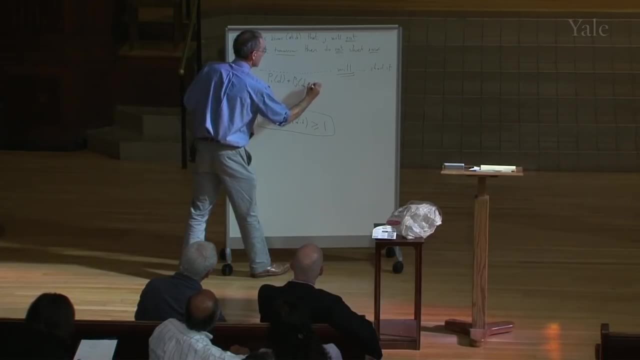 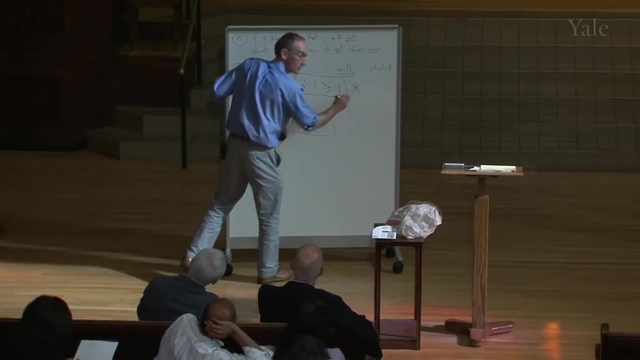 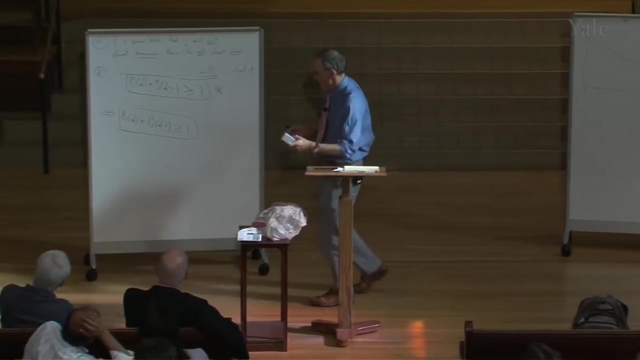 Shoot if- and I'm going to rewrite this rearranged equation, which is P-I D plus P-J D minus one, is greater than or equal to one. There it is Charles, okay, Okay, Alright. so what do we know? now? We know what you. 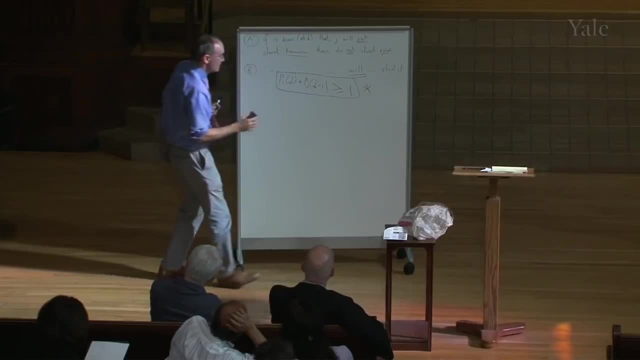 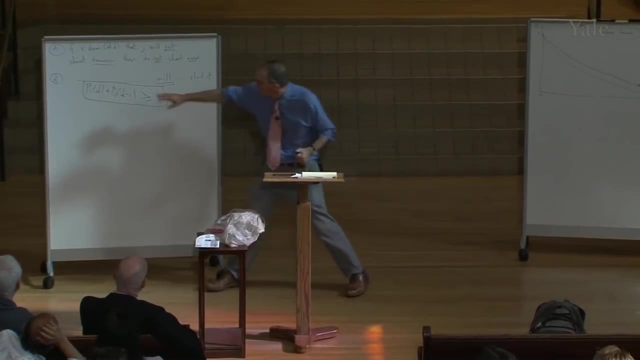 should do if you know the other person's not going to shoot, that is to say, you should step, And we know what you should do if you know the other person is going to shoot, which is you should shoot if, and only if, this sum. 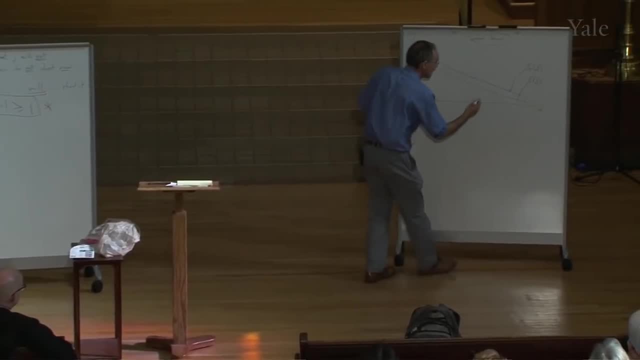 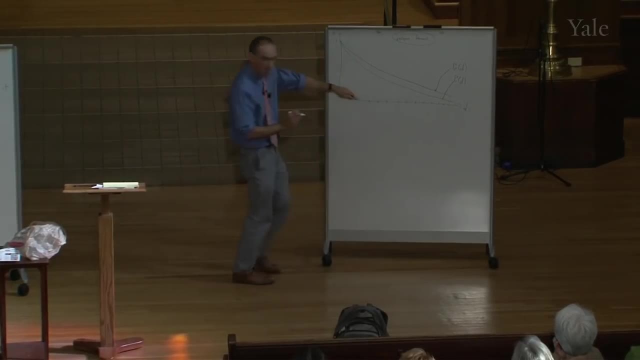 is bigger than one. Let's go back to our picture. Let's put some steps in. So these are very little steps because it's a very little picture. I'm not insulting the foot size of the beans, it's just. you know, I've scaled it. 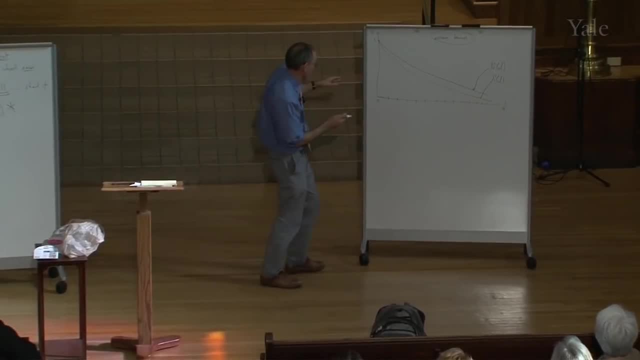 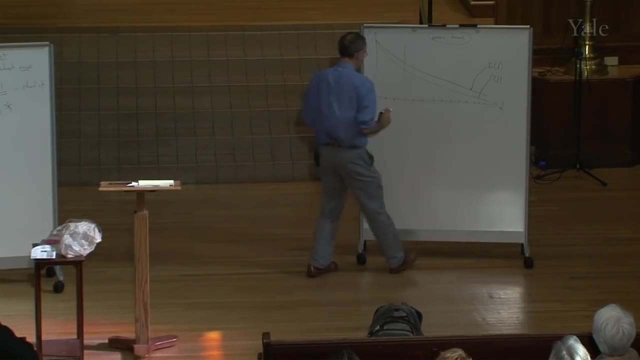 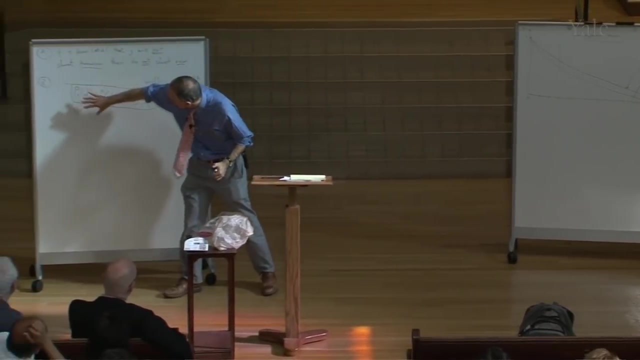 down, okay, And let's see where would this be roughly So, probably here Guessing Alright. so let's ask the question: when is this equality as in equality met and when is it not met? Okay, So at the beginning of the game. 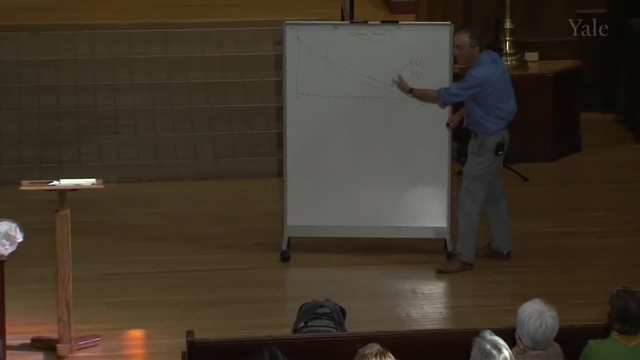 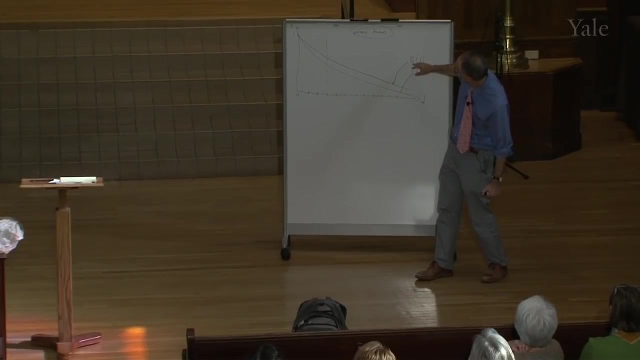 when people are out here. if we ask the question, is PID or P1D at the beginning? P1D plus P2D minus one, is it bigger than one? Is it bigger than one out here? No, it's small right. 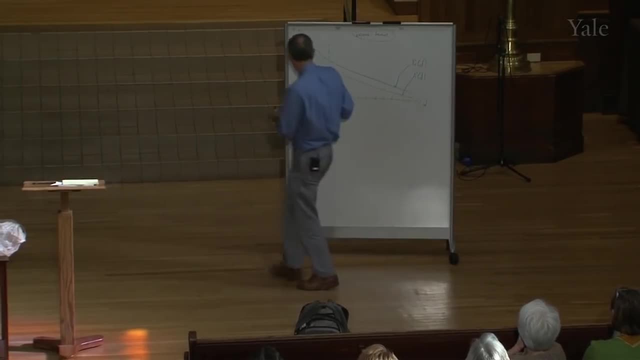 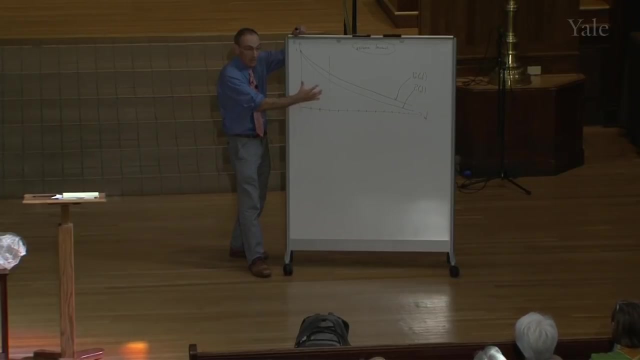 These are two small things, so it's going to be smaller than one. On the other hand, once we're in here, once we're in really close, there's some of these two probabilities, that's bigger than one. Okay, Everyone okay with that. 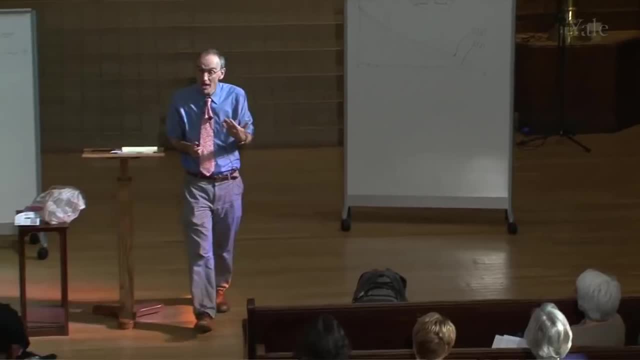 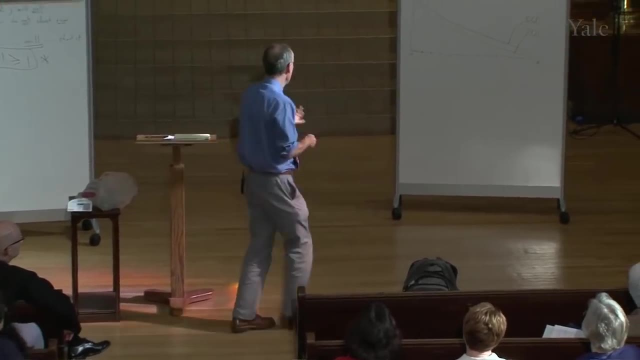 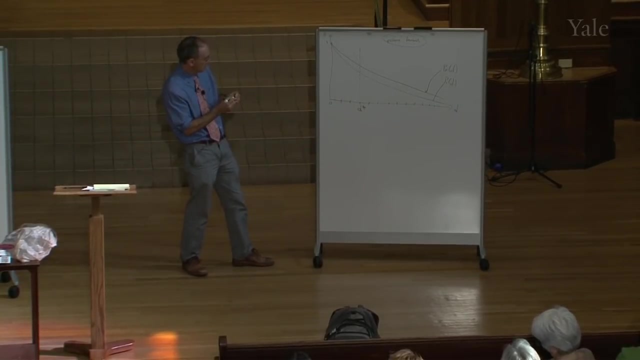 And there's going to be a critical point when, for the first time, the inequality switches from being incorrect to correct, from being false to being true. Alright, and we're going to call that distance d star, Alright. so I'm drawing it approximately here, but pretend it's accurate. 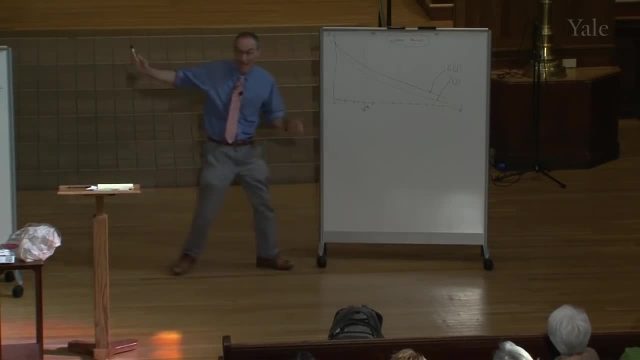 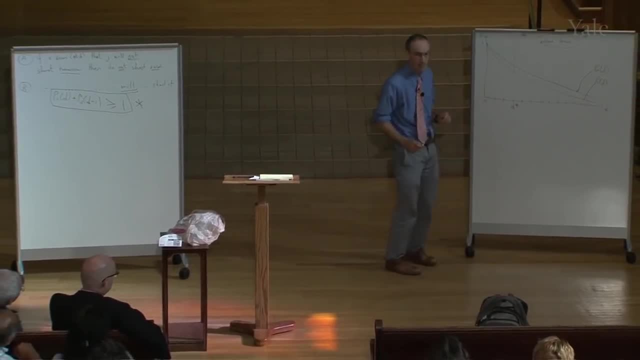 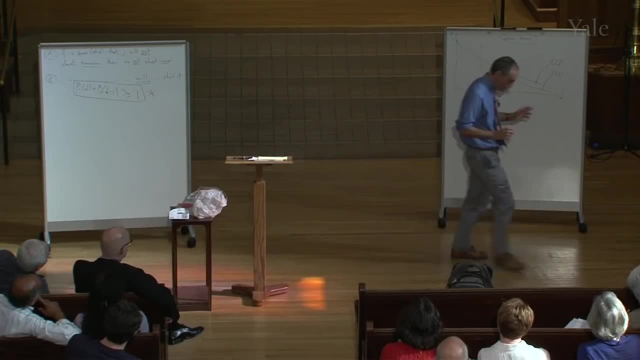 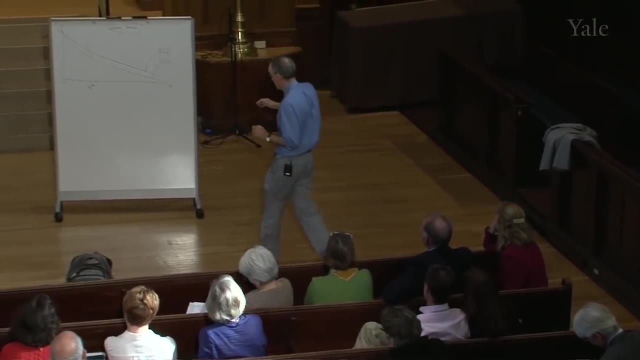 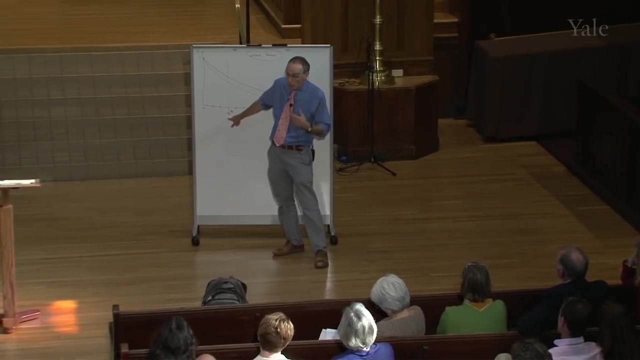 So I claim that the following is true. I claim that nobody should throw their sponge until d star, But whoever's turn it is at d star should throw. And were it to be the case that they didn't throw at d star, then the next person should throw at d star minus one. 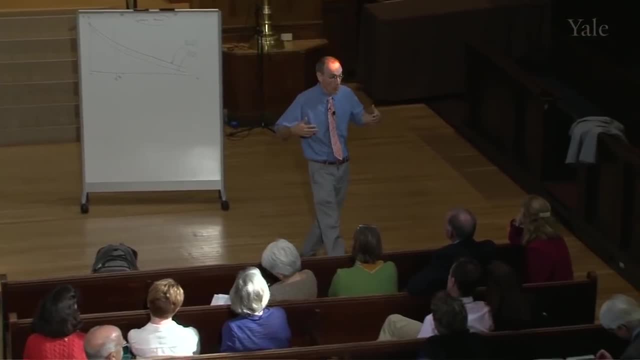 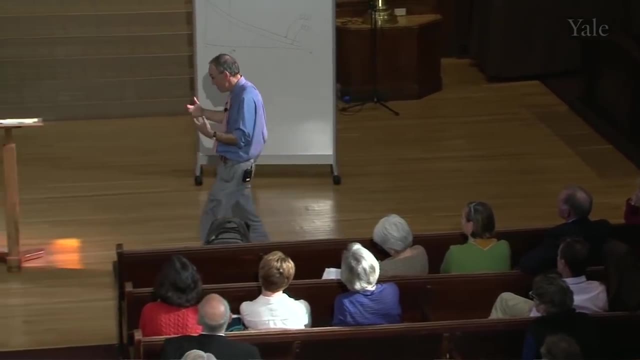 So here's my claim: Nobody throws before d star, but at d star you throw whoever it is. Okay, that's what we're going to try and convince you. try and convince you that that's true. Alright, To convince you that this is. 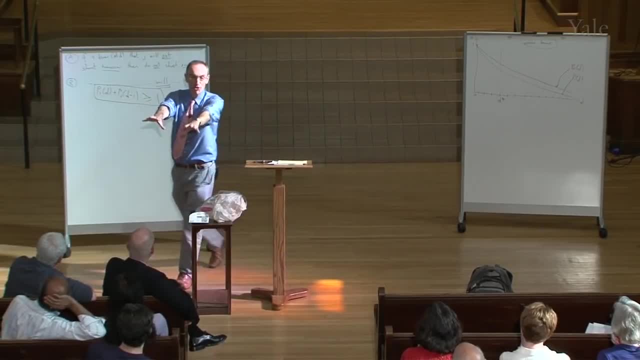 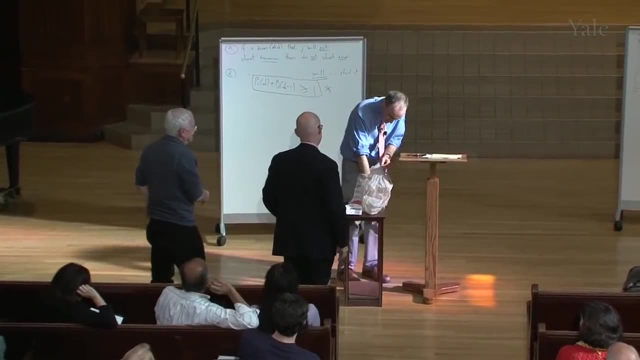 true, we're going to use these two facts and these two stooges, Alright. So I'm going to bring my stooges up again And convince them. we're going to. if this was ESPN, we would be playing things in slo-mo. 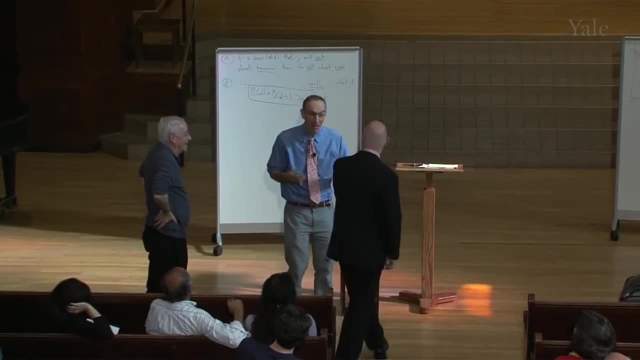 I don't have. actually in the drama school they probably have that, but I don't have slo-mo in here, So we're going to play slo-mo in kind of imagine slo-mo. So here we are, back at the beginning. 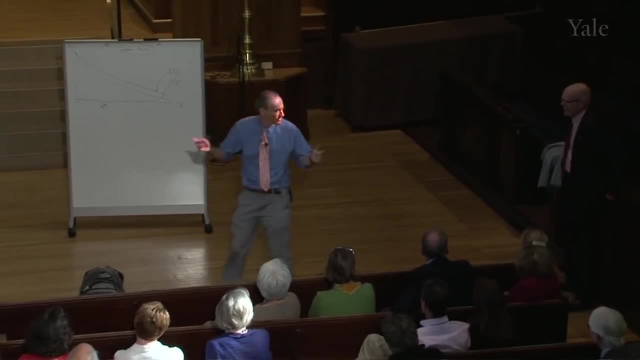 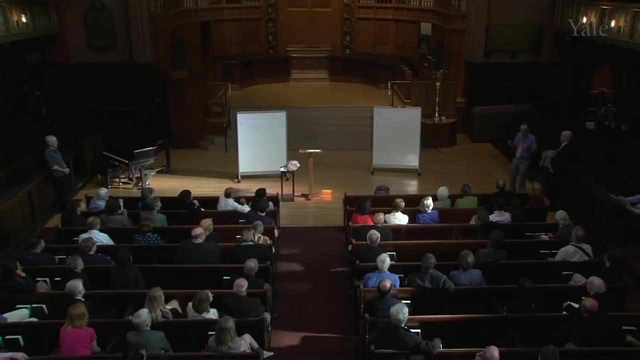 of the game and we're going to do slo-mo. And here we are. who was first? I've forgotten. So James was first. he's player one and he's thinking what should he do? Should he throw or step? 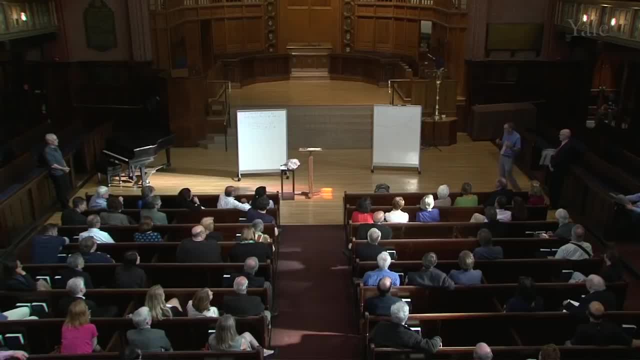 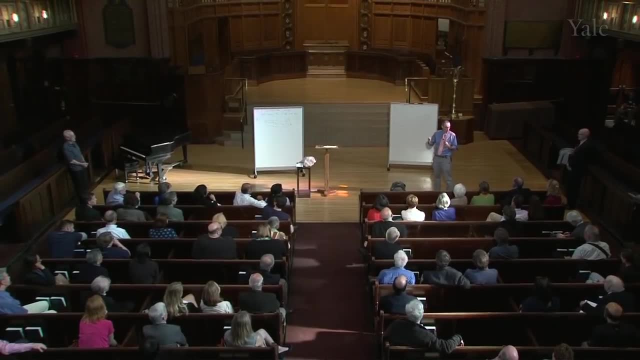 And we know the answer, but let's just walk through it slowly, Alright. So James can think the following way: Suppose suppose Robert was not going to throw next go. Suppose it's the case that Robert is not going to throw next go. 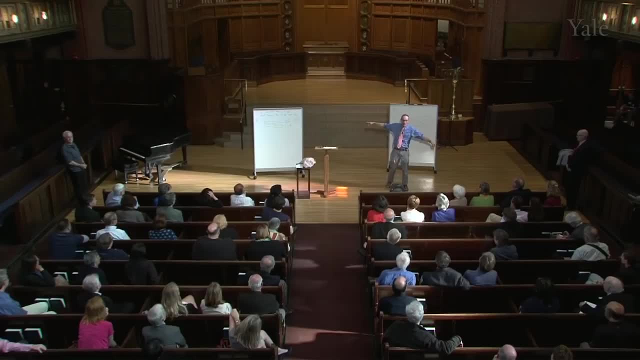 Then which fact should he use? Should he use fact A or fact B A? And what would his conclusion be? Step Okay, That's one thing that Robert could think. Sorry, one thing that James could think, But the other thing James could think. 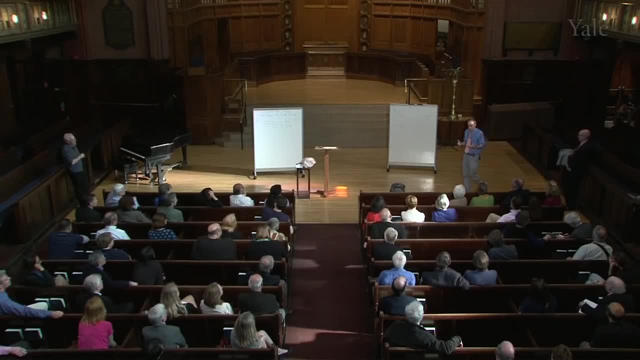 is he could think. suppose Robert is going to throw next turn, Right? So if James thinks that Robert is going to throw next turn, then he should use fact B And the conclusion should: be well, if he's using fact B, 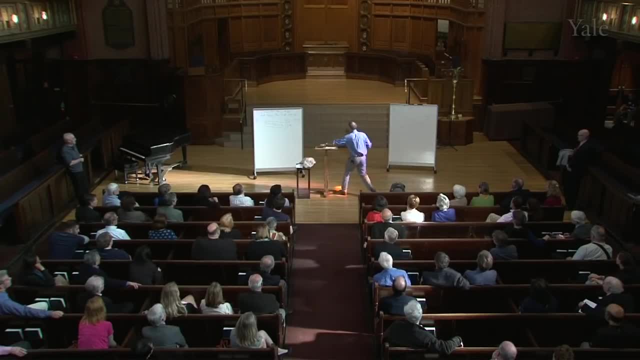 James should throw if his James' probability today plus Robert's probability tomorrow- there it is, I've just drawn those lines- is bigger than one. Is it bigger than one? No, So he should step. So in this case, whether James 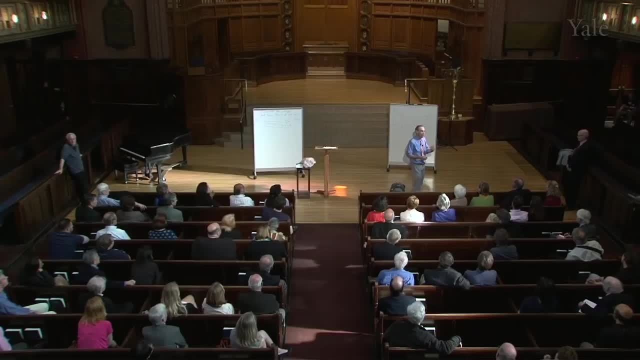 thinks that Robert is going to throw tomorrow, or thinks that Robert is not going to throw tomorrow, you arrive at the same conclusion, Namely, you should step, and therefore you should step. Okay, Step, Alright, Alright, So let's do this once more in Robert's 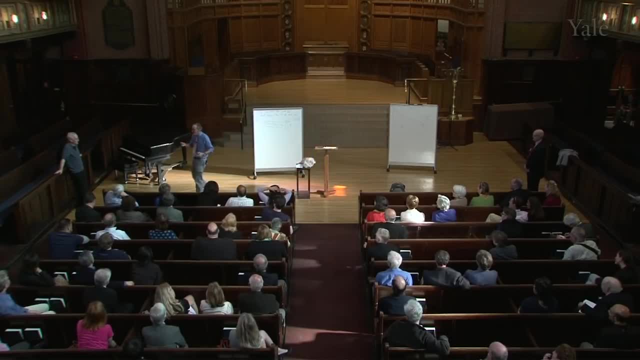 shoes, but you'll see the same idea, so I'll do it faster. I can speak fast. Here's Robert. Robert is thinking what James is going to do. If Robert thinks that James is not going to throw tomorrow, then by fact A. 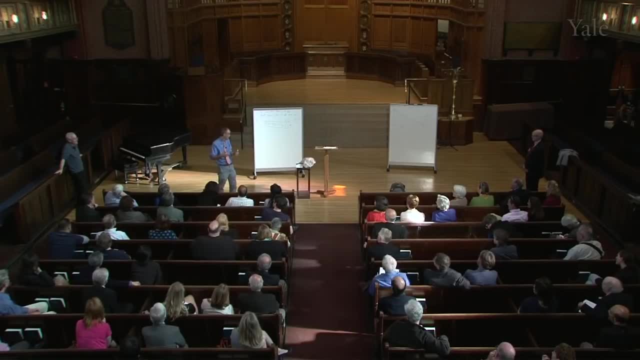 Robert should step. and if Robert thinks that James is going to throw tomorrow, then he should use fact B and look at these lines in here and say: throw if this line plus this line is bigger than one. but they're not bigger than one. 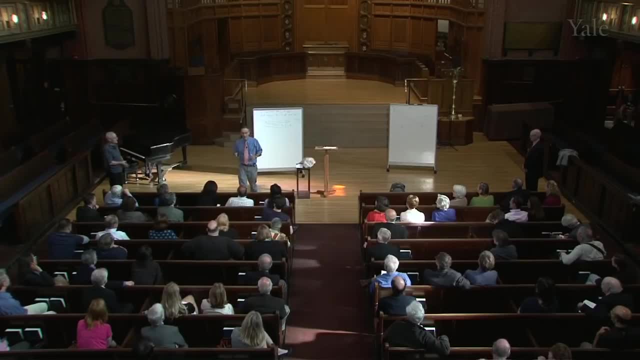 they're smaller than one and therefore, either way he should step, so he should step. Okay, Everyone okay with that argument? Okay, Okay, So just I promise I'd point out some things as I'm going along that are more general lessons. 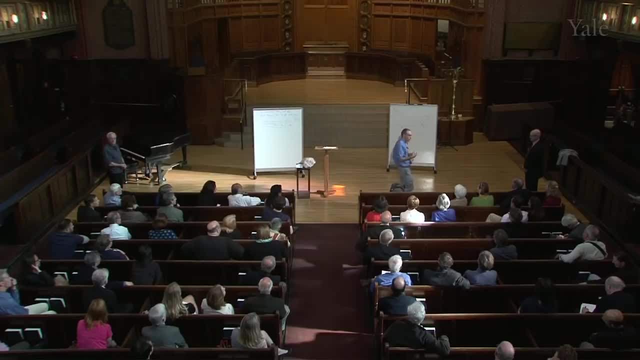 Alright. So the thing we just saw was an example of what's called a dominance argument. A dominance argument says: if I think A, if I think, I don't want to use A, because if I think P, then I should do X. 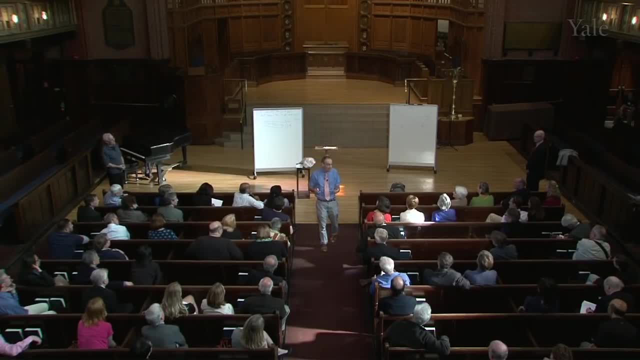 and if I think not P, then I should do X. therefore, I should do X. Alright, Dominance argument's pretty straightforward, but people get them wrong. Okay, so if you do the same thing, whether P or not P is true, then you should do. 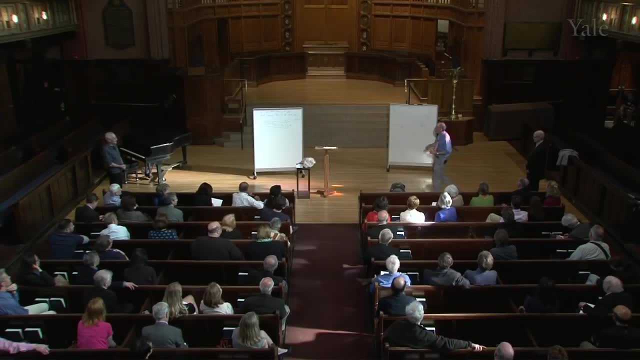 that thing. Okay, If I had time, I'd give you examples of movies where they don't do it, but never mind, Okay, so alright. so fine. so Robert should step, and then James will go through the same argument. it'll still be a. 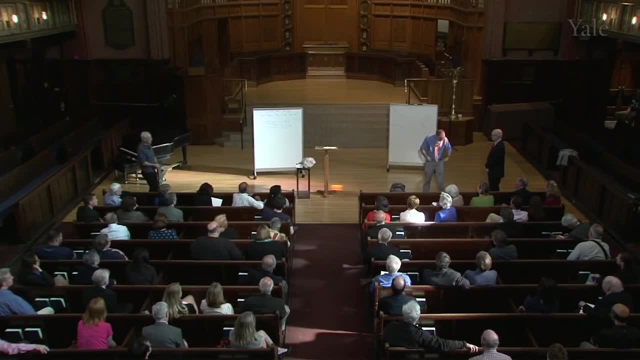 dominance argument. so he should step, and then Robert should step, and we're going to go in fast motion for a second, and this will go on being true until we get to about here. Come, come, come, come, come, come. 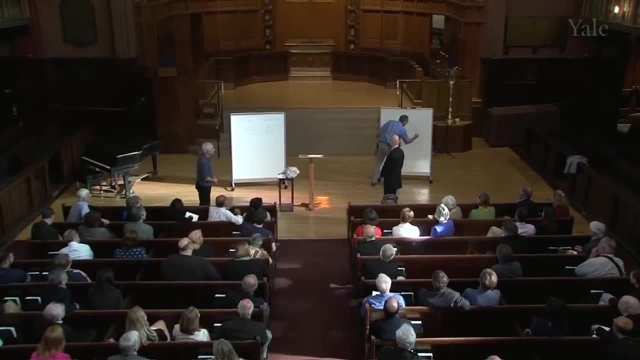 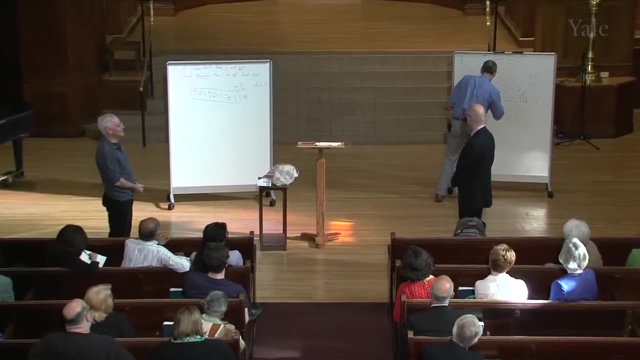 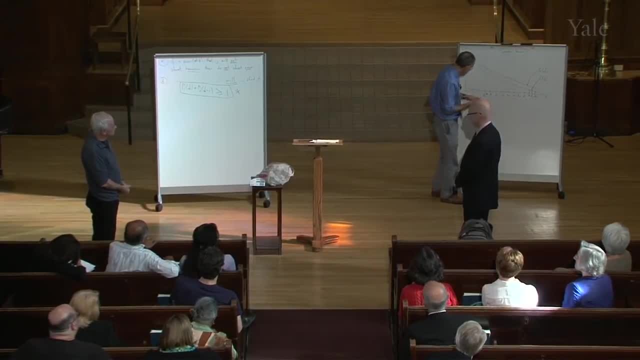 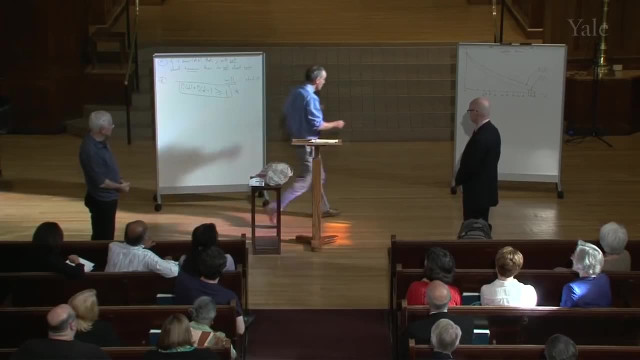 2, 1,, 2,, 1, 2,. so here we are finally at D start. all the way through this argument, including the last step, which was James' argument, at D star plus 1, the dominance argument said: 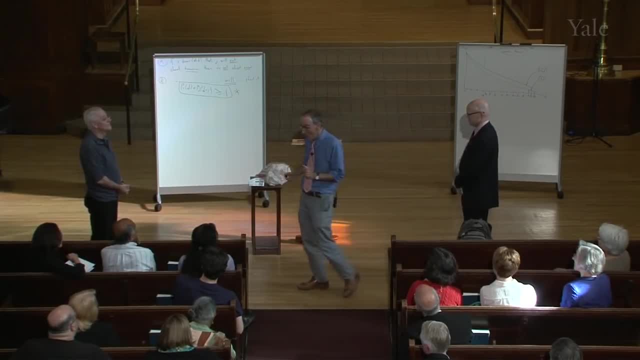 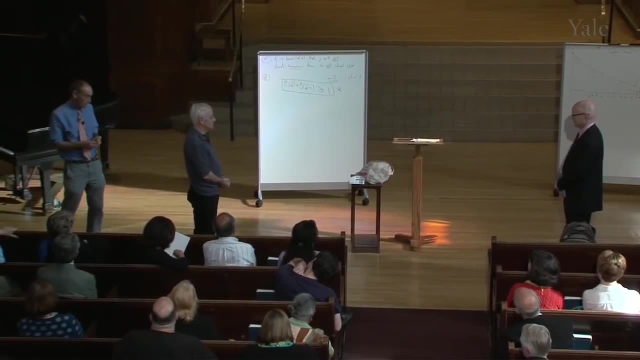 no matter what, I think I should step, so I step. Now, however, we arrive at D star, and here's Robert at D star and Robert's thinking through the same reasoning. So here we are. we're in Robert's head. 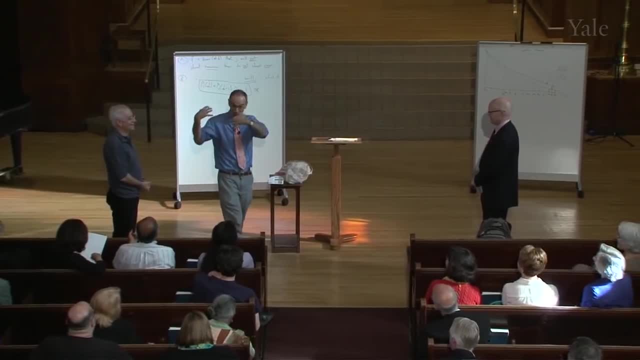 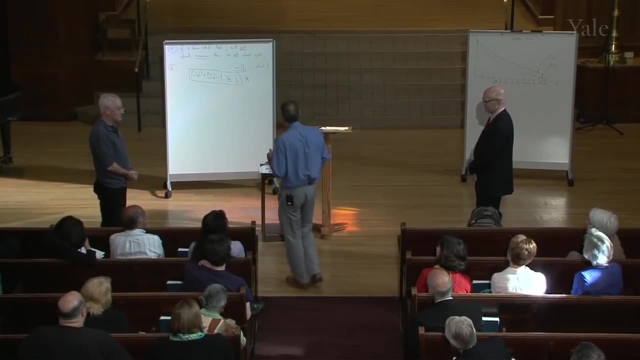 this is a good head to be in. I've read some of his stuff. so imagine yourself in Robert's head and Robert is putting himself in James' head and I think through and Robert is saying: if I think that James is not. 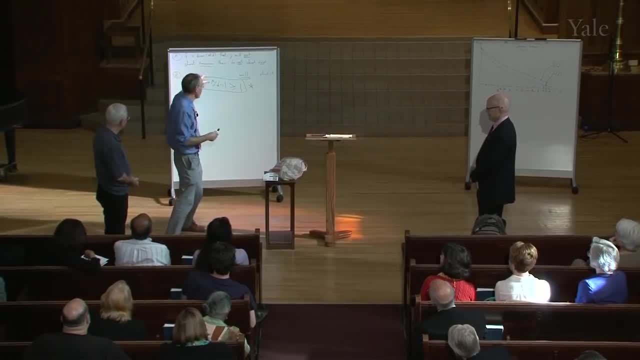 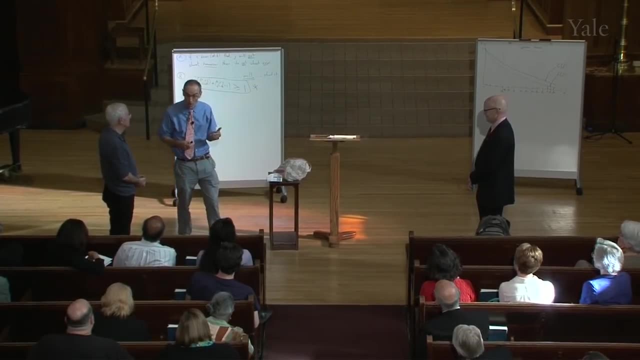 going to shoot tomorrow, then I should use Fact A, and that tells me not to shoot today. But if I think that James is going to shoot tomorrow, then I should use Fact B, and this time, for the first time when I walk my way through, 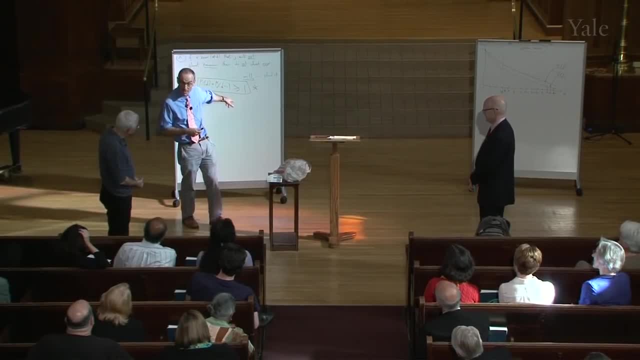 Fact B: it tells me I should shoot today. right, because I'm at D star. So now these two arguments are pulling in opposite directions. If I think the other guy isn't going to shoot, I should step. If I think, 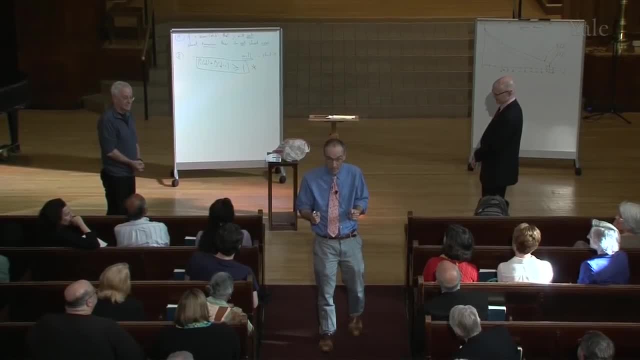 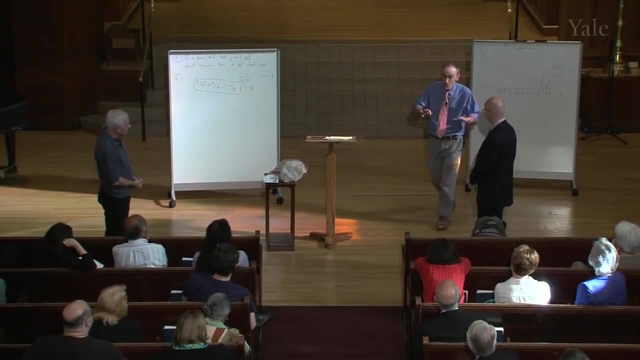 the other guy is going to shoot, then I should shoot. So I'm stuck, I'm stuck. So it was easy. up to now we had don't shoot, but now we're at D star. Now, if Game Theory could say nothing other than these: 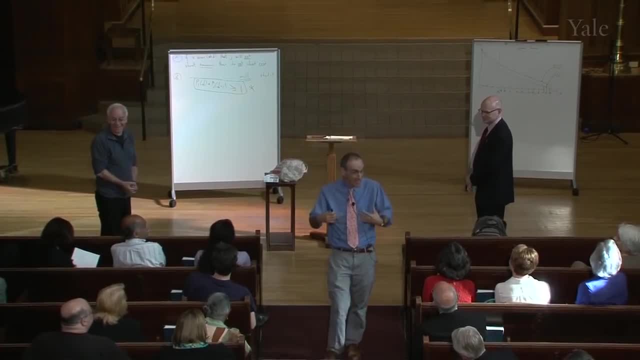 dominance arguments. you probably shouldn't take my course, So it better be the case. I've got some way out of this dilemma. This is a dilemma, but I've got a way out of it, So here's how we're going to get out of this dilemma. 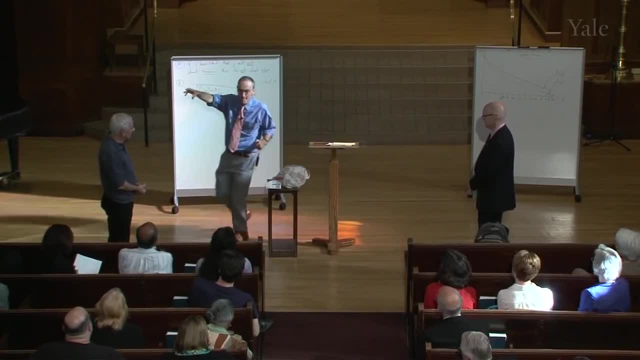 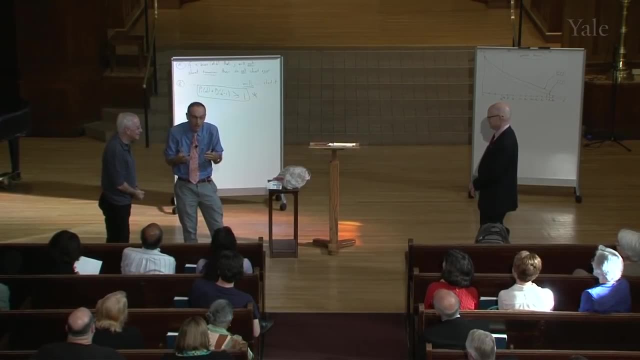 We're going to figure out. remember we're in Robert's head. Echoey in there, Here we are. it's like a church. So in Robert's head we're going to try and remember. this dilemma would be solved if Robert knew. 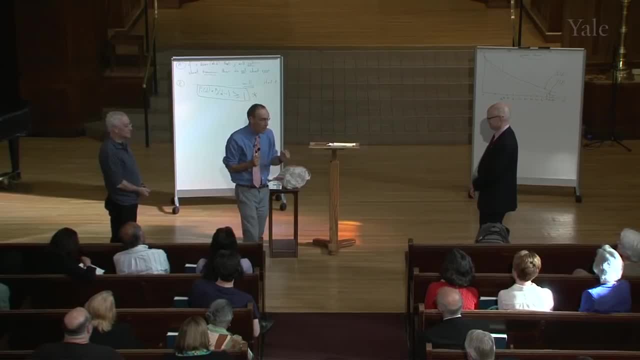 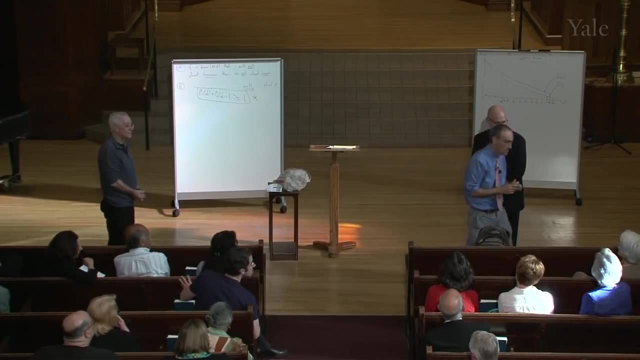 what James was going to do tomorrow. So we're going to work out what James is going to do tomorrow, But we're not going to do it, as was suggested just now by Mr Morse, by just taking one step forward. We're going to take 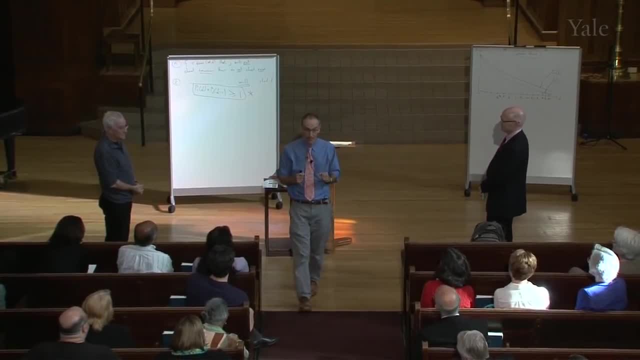 lots of steps forward. In fact, we're going to go to the end of the game. So what's the end of the game? The last possible step in the game. So come forward, come forward. No one shoots. Come, come, come. 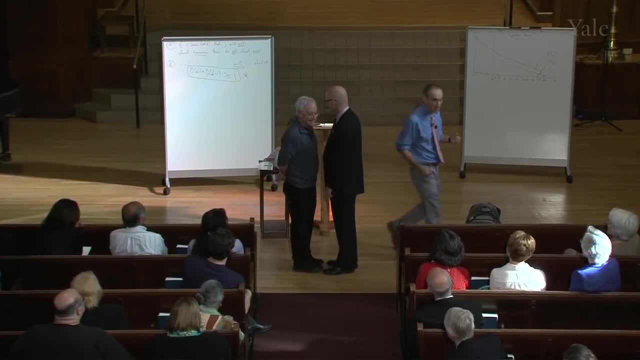 Come on personal space, but further forward. All right, okay, all right. So this is the end of the game. All right, No one shoots, no one shoots, no one shoots. Eventually, they're on top of each other. 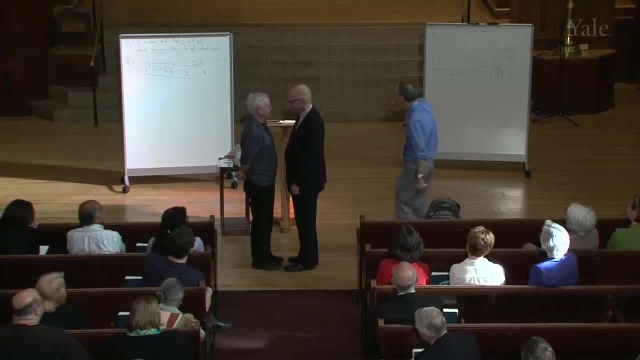 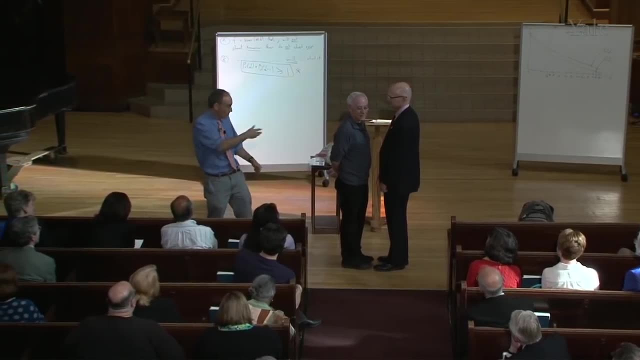 Their noses are touching. It's uncomfortable, All right, All right, Okay, And here we are at the end of the game and this turns out to be Robert's turn again. So if Robert finds himself at distance zero from James, if we get here, 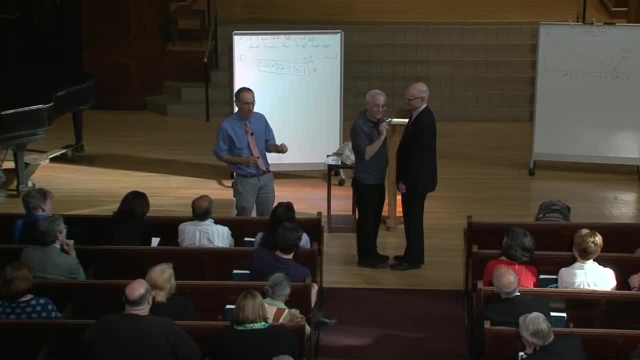 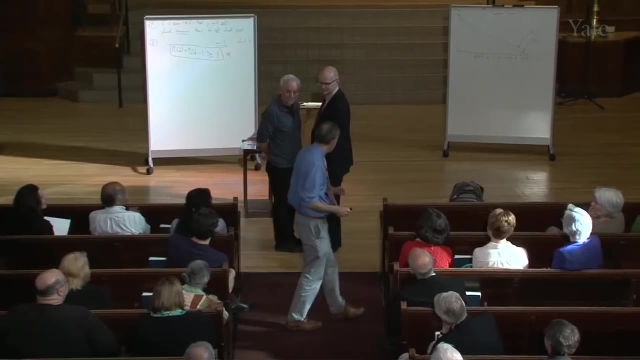 what should Robert do? Sorry, what should Robert do? He should shoot. Why should he shoot? Because he's going to hit with probability one, So he should shoot. Is that right? All right, so that was easy. So, if we get to, 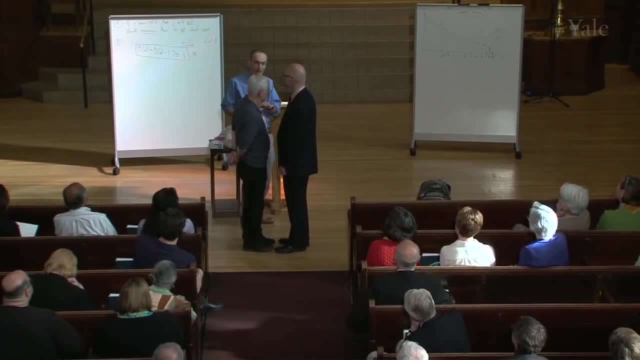 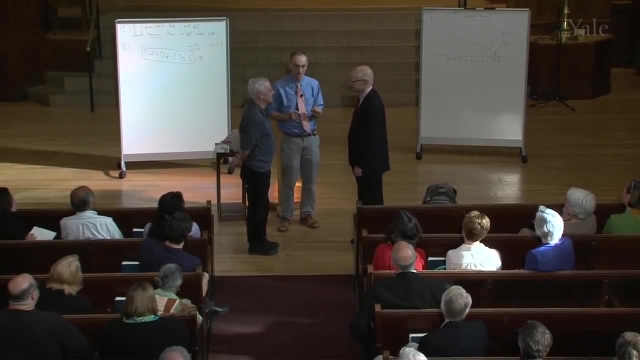 this stage. Robert's going to shoot. Let's go one stage back in time. No, no, no. it must have been his turn. It's your turn now. so the previous turn must have been James'. So James' is going to go back in time. Okay, so here we are. 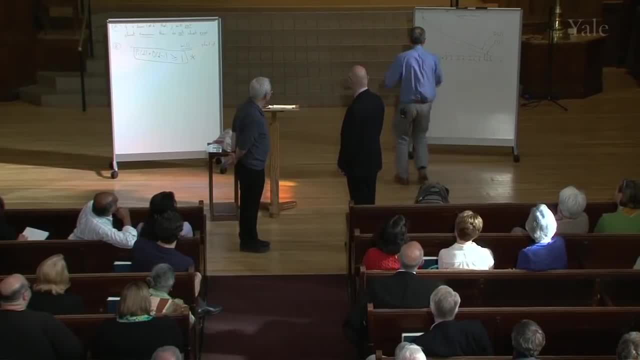 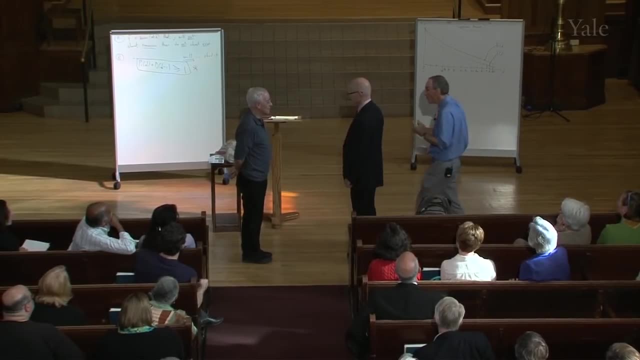 one. now. they're distance one apart. By the way, we had a shoot here right Now. they're distance one apart and it's James' turn. And now what does James know that Robert's going to do tomorrow? What does he know if James doesn't shoot? 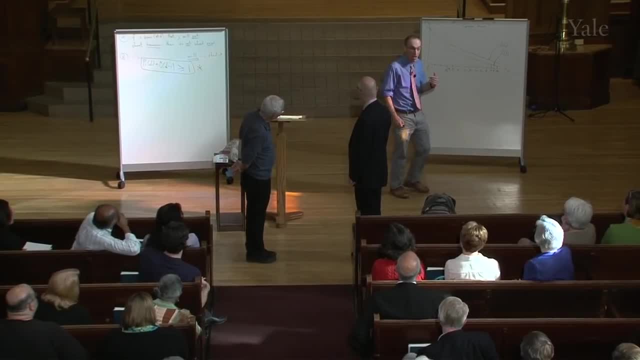 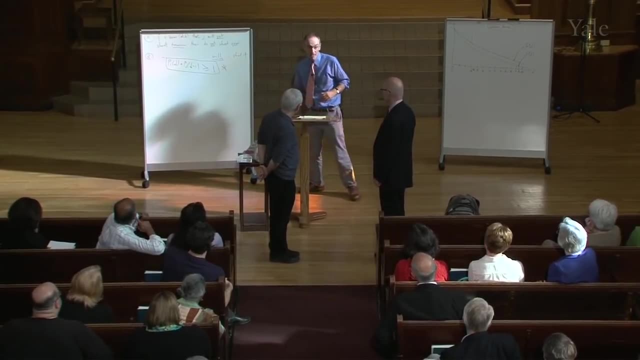 He knows, we just put it on the picture. he knows that Robert is going to shoot And therefore James should shoot. he should make that decision based on fact B, Is that right? James knows Robert's going to shoot tomorrow, so James. 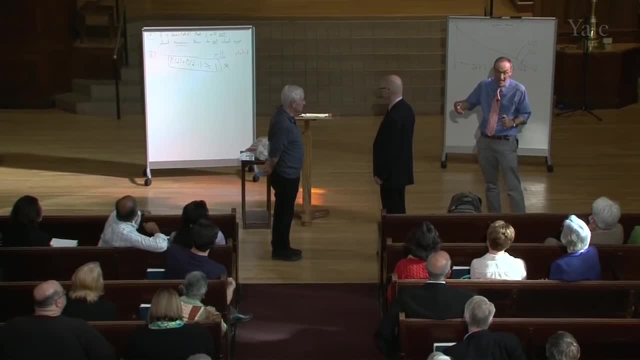 should shoot if his probability of hitting now plus Robert's probability of hitting tomorrow is bigger than one. and since Robert's probability on his own is one for sure, one plus something is bigger than one. That was the second bit of math, I lied. 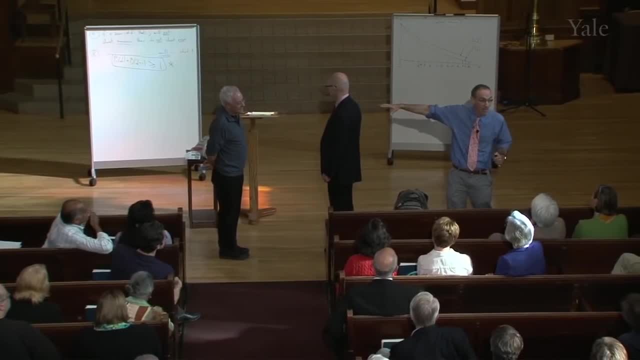 Okay, there were two bits of math in the course, So one plus something is bigger than one, so he should shoot, Is that right? So, James, you would shoot at this point, right? So now let's go back one more stage. 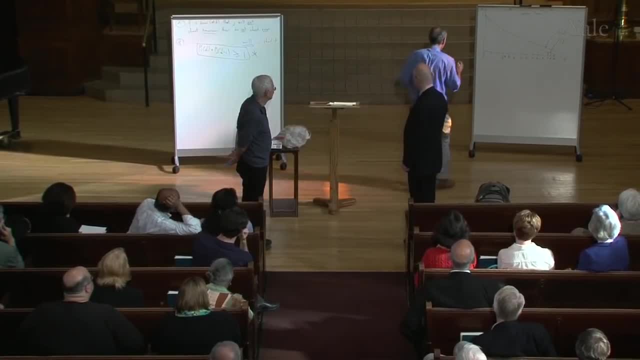 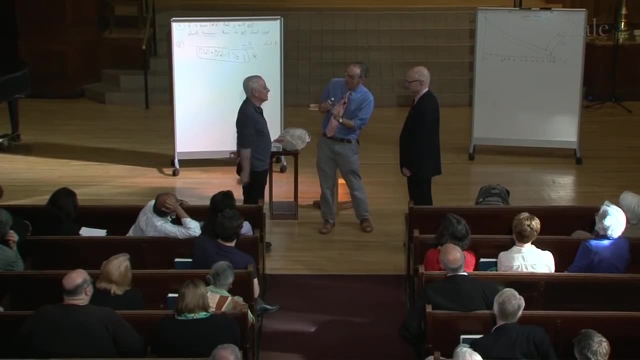 So here we are now. we're at stage two away, Alright, and now we're in Robert's head. and what does Robert know? He'll shoot. and therefore, what should you do? Shoot, right. Why should you shoot? Because you go through fact B and you find: 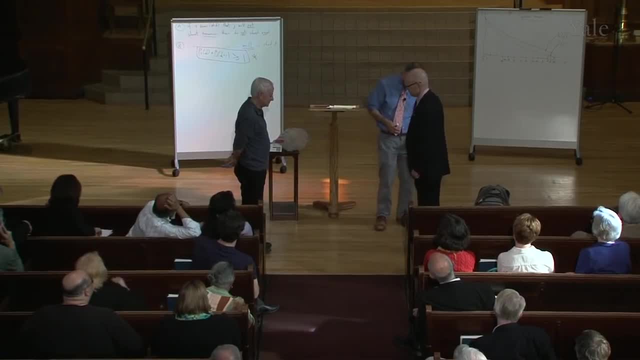 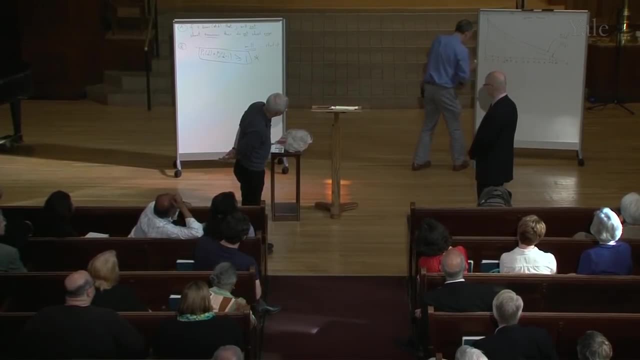 some of the probabilities are bigger than one, so he should shoot. So let's go back to another step. Alright, and here we are at stage one, two, three. Here we are at stage three, which is actually our d star minus one. 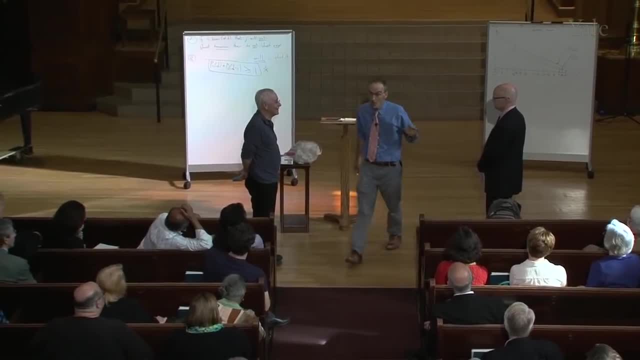 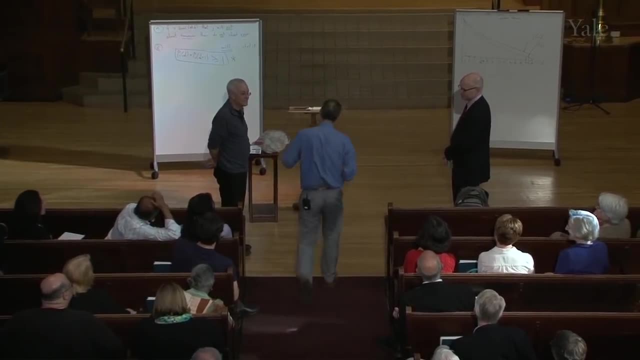 Here's James. This is what we were worrying about, right? So what does James know at distance three? What have we just worked out? He knows that James knows that Robert's going to shoot, and so James should use fact B. 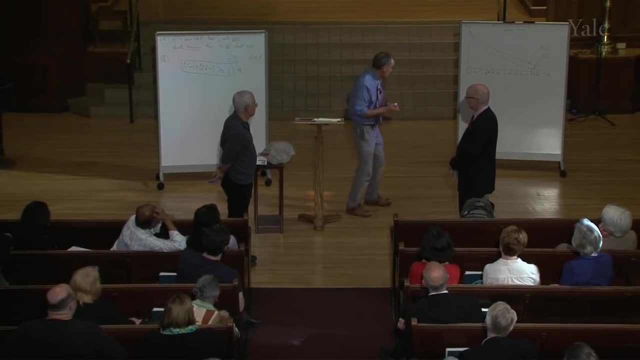 and, using fact B, he should shoot. Okay. so now let's go back one more stage. And now we're back where our dilemma was. Now we're back at d star. I've worked my way back to d star, But what's different Now, when I arrive at 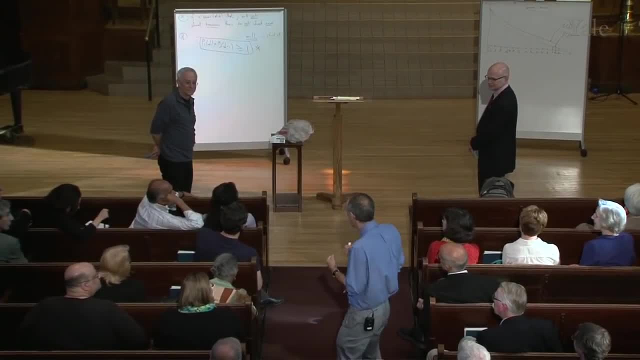 d star from the end. Remember, last time I was at d star I had a dilemma in Robert's head because I didn't know whether James was going to shoot or not. But now I do know what he's going to do. 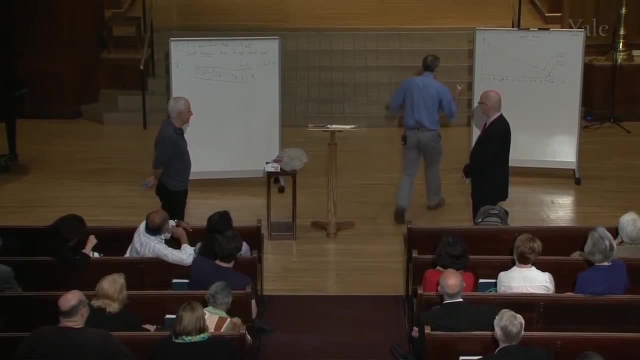 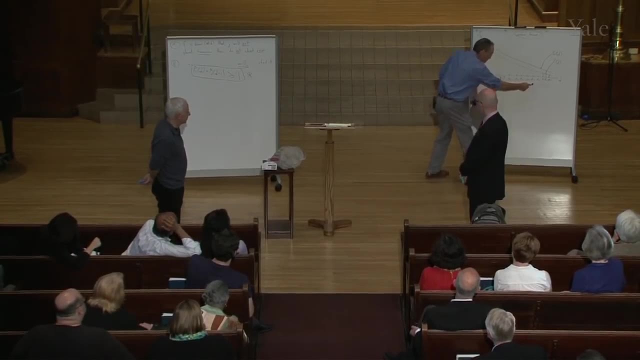 What's he going to do? Shoot, And therefore, what should you do? Shoot, There we go. So we've just shown that, at d star, Robert should shoot. In fact, what have we shown? We've shown: until d star, nobody should shoot. 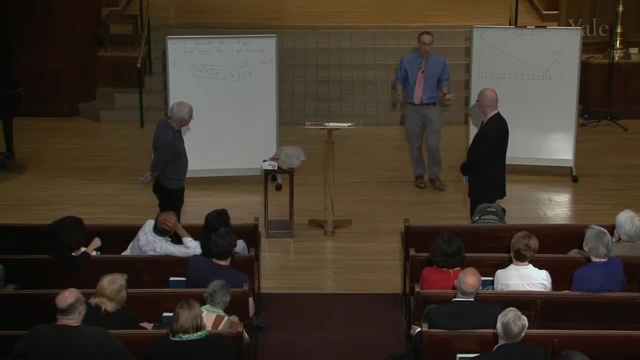 but at d star, and if you get there any stage afterwards you should shoot Alright. so thank you to my two doogers again sitting down again. Thank you, You can go to your seats if you want. Thank you. 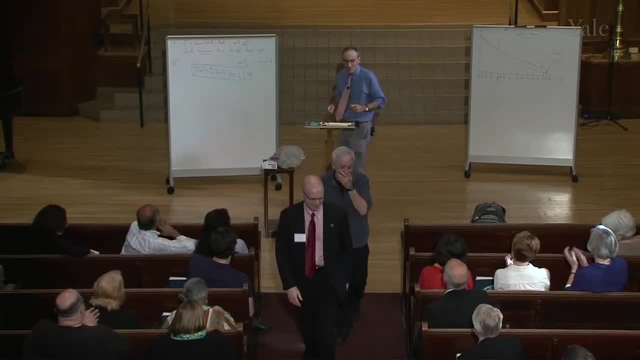 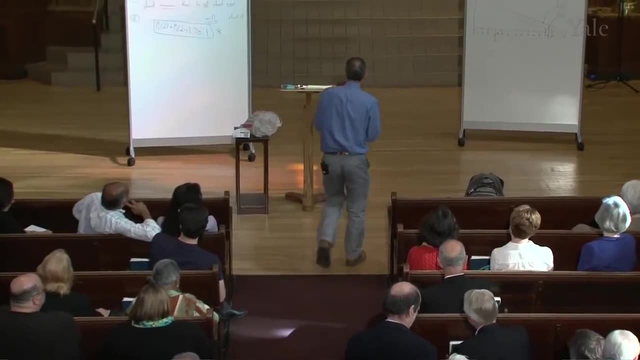 Alright, thank you. Alright, You expect them to be great actors and great interpreters of the law, so that's good. This is the law of game theory, Alright? so what have we just shown? Let's just make sure we understand what we just showed. 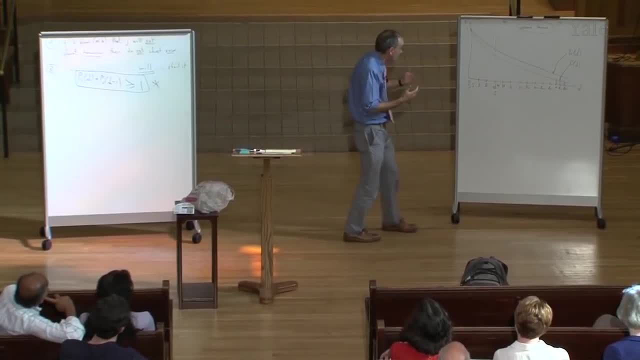 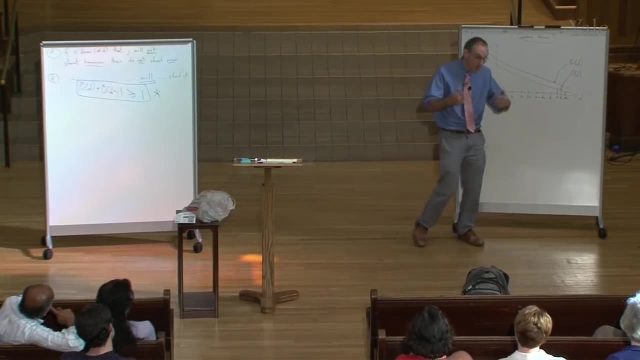 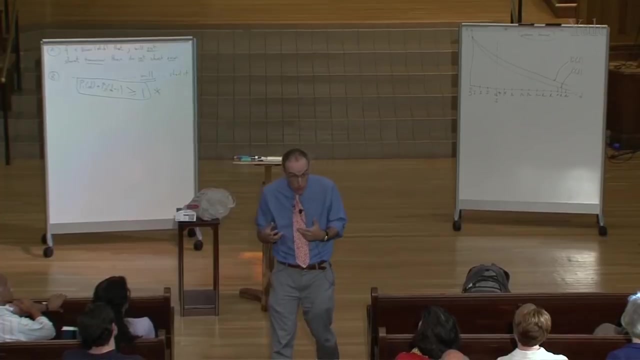 We showed that, what I claimed. we showed that no shot should occur until d star, and that at d star- which of course depends on people's abilities, but at d star, whoever's turn that happens to be should shoot. And we used two big ideas. 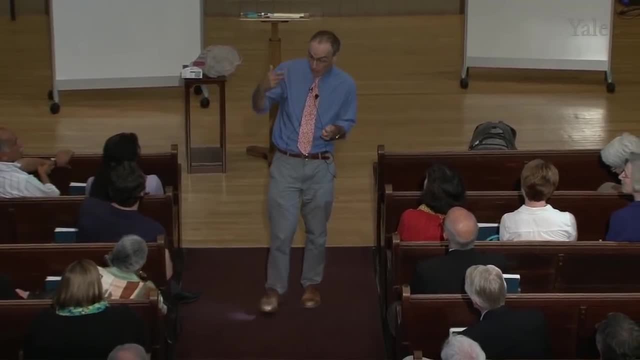 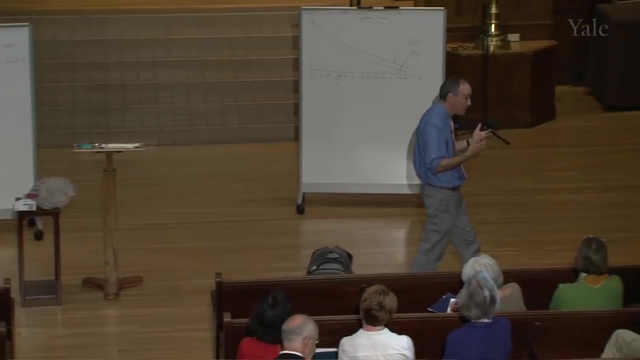 I didn't point out the second one, so I forgot. I'm going to do so now. The first big idea was this dominance idea, And the dominance idea was: if in circumstance p, you should do x, and if in circumstance not p you should do x, then you should do x. 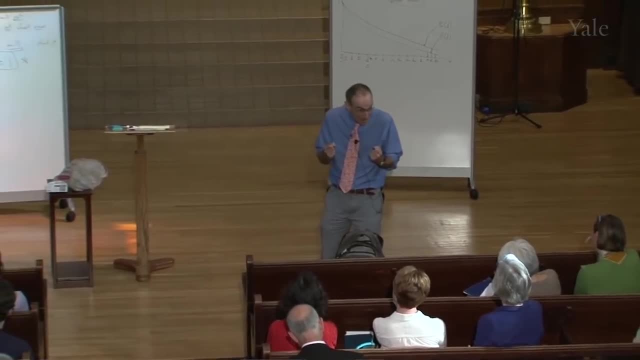 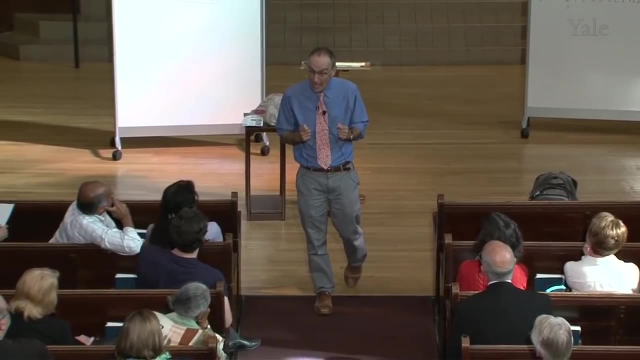 Alright, I'm saying that adamantly because it seems obvious. And that was one big idea. And the other big idea was: when you get stuck in thinking this way, a really good way to solve out a game is to go to the end of the game. 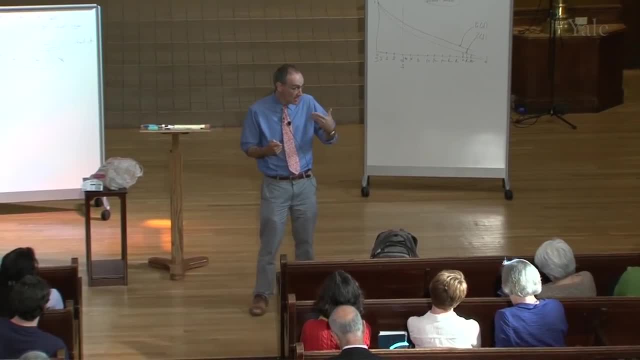 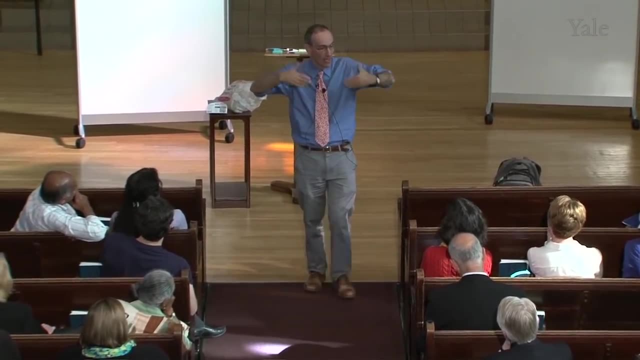 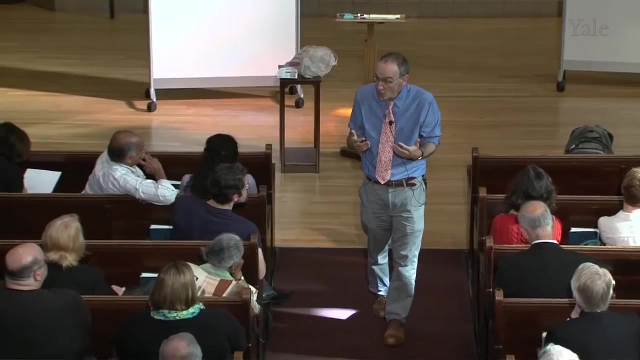 and work backwards. It's good to anticipate what people are going to do, and the best way to do that is to go to the very end of the game and then work yourself back forward again. Now that idea is called backward induction, And backward induction is 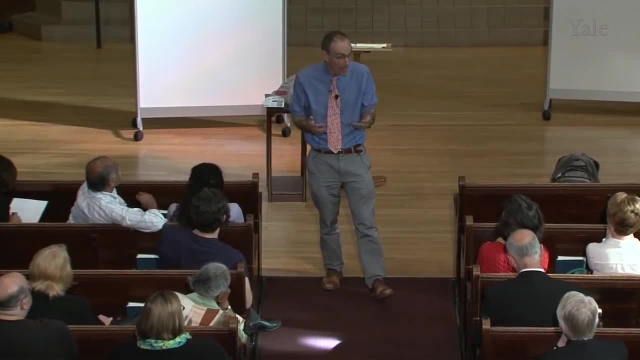 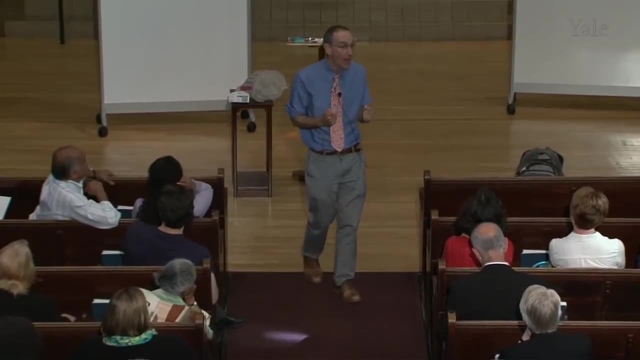 the most important thing you're going to learn if you take a game theory class. It's hard to do- actually It's hard to do because it's hard to make yourself do it. It's hard to have the instinct that I really should work backwards and not forwards. 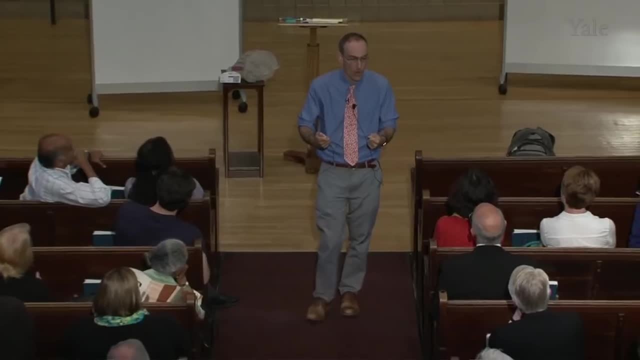 Time works forwards, Our logical way of thinking works forwards. But when you're trying to play a game with somebody trying to put yourself in other people's shoes, while they're putting yourself in your shoes, trying to anticipate what they're going to do, 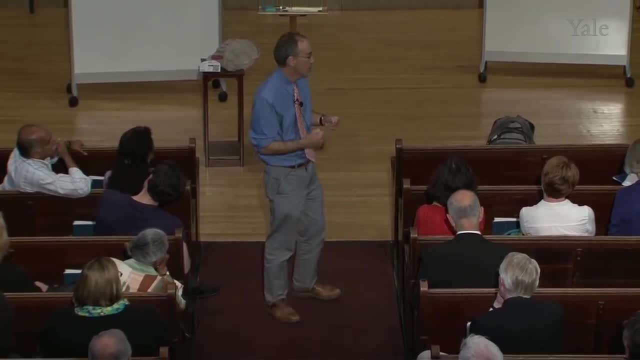 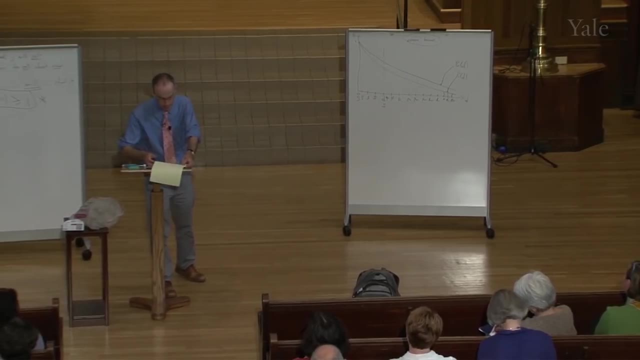 while they're anticipating what you're going to do, it's easier to work backwards, So backward induction combined with dominance tells us when we should shoot here. All right, So let's just go back to the beginning and just make sure we understand the game. 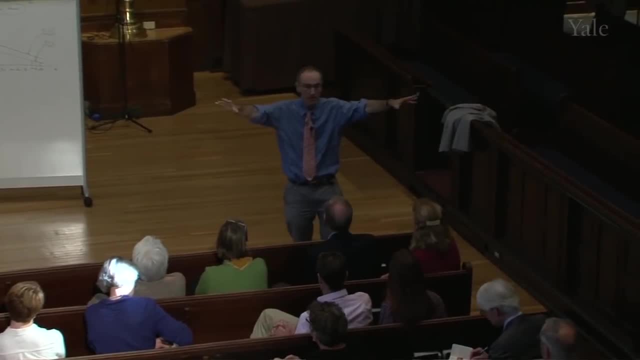 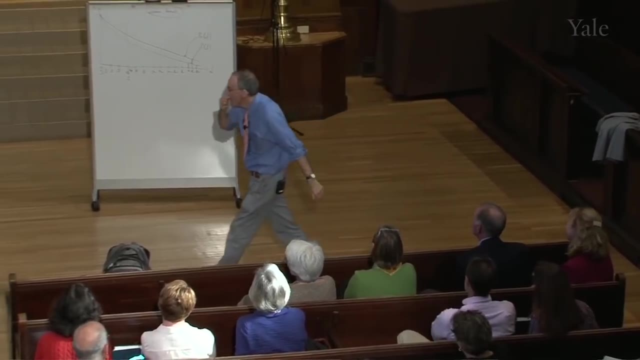 before we draw out any more general lessons. People, okay, at this point I don't particularly look like deer in the headlamps, which is a good sign to say: I haven't lost too many of you, Is that right? Good, Okay, so 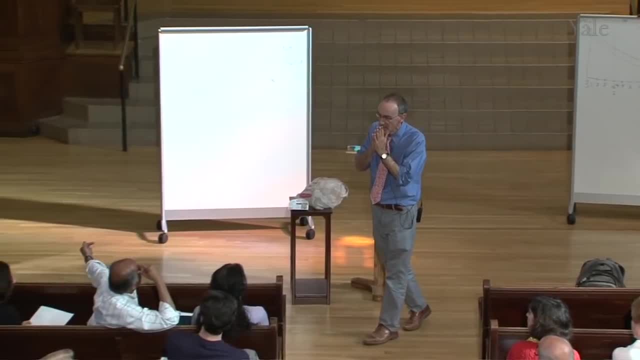 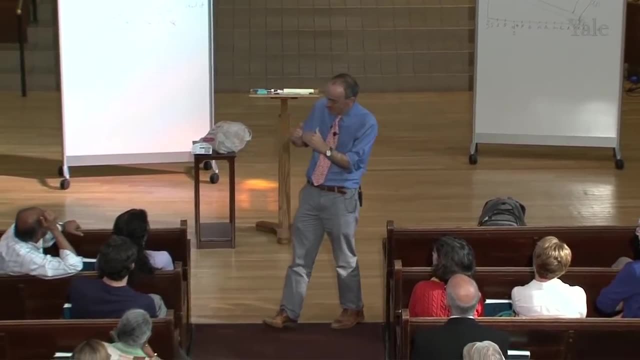 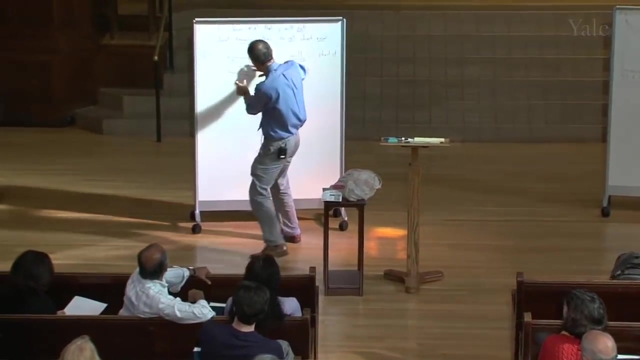 Yeah, Yes, It's, because if you look at those inequalities it's monotone. So I'll show you Basically. as you get closer, both people's probabilities are getting higher. So that pair of probabilities you're always going to cross one out and replace it. 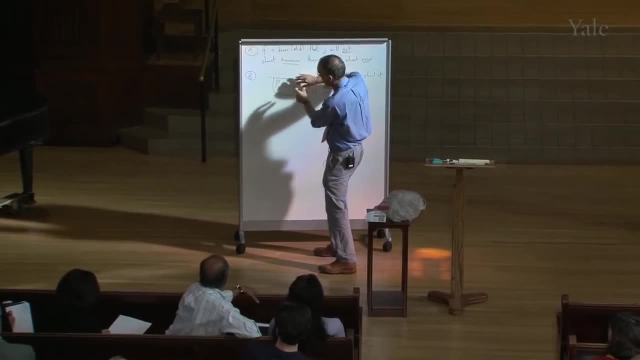 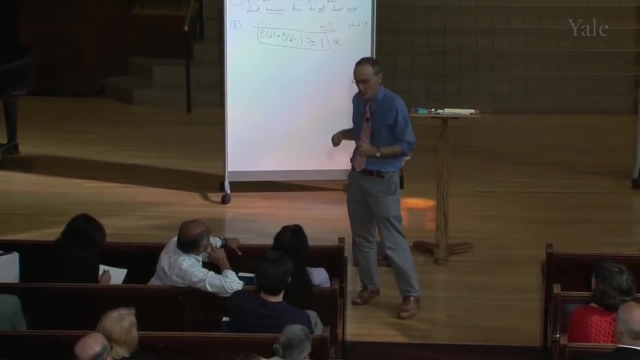 One of them will survive and the other one will be crossed out with something bigger. So once you cross this inequality, you can't go back. It's a strictly monotone sequence. That was a physicist asking the question, so I assume I answered. 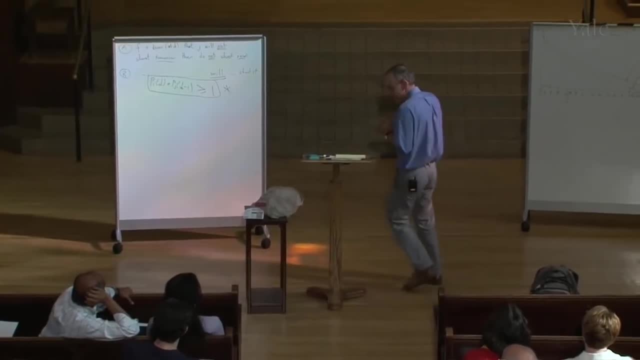 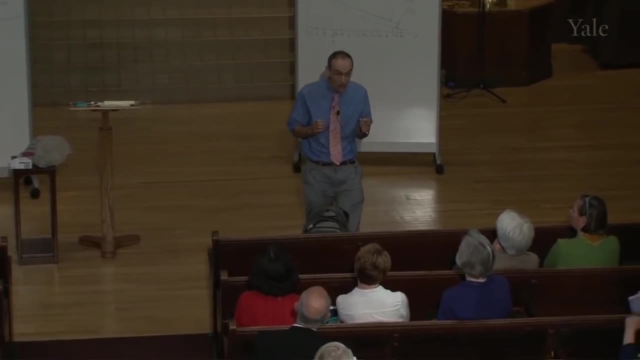 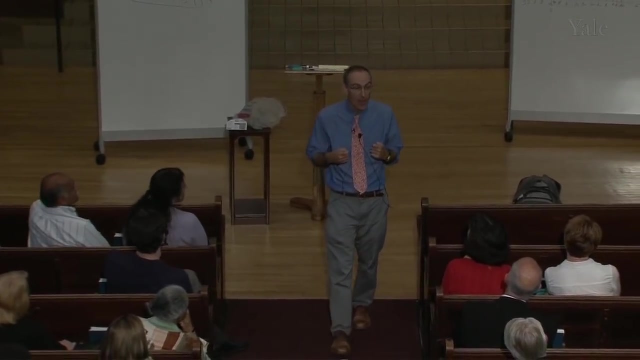 in the appropriate language. All right, good, Okay. So what do we show? We showed that it isn't as simple as asking: should the better shot shoot first or should the worst shot shoot first, And it isn't even a question of 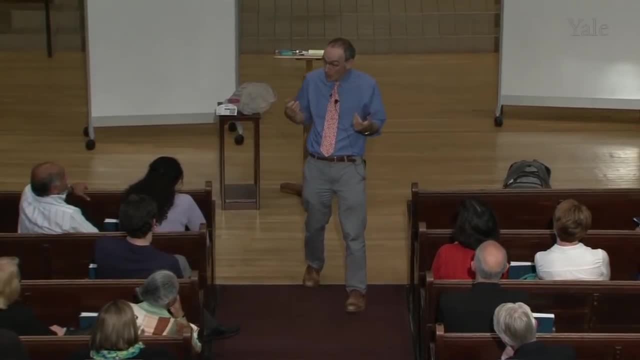 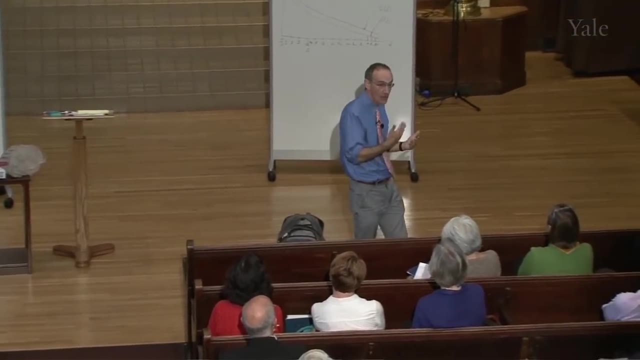 preemption and preempting preemption. It's a question of understanding both probabilities: working the thing backwards and finding out that there's a critical moment to shoot. I want to be careful here. I'm not saying that that critical moment to shoot doesn't depend. 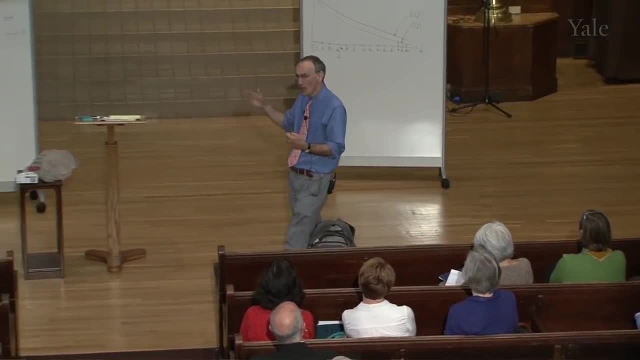 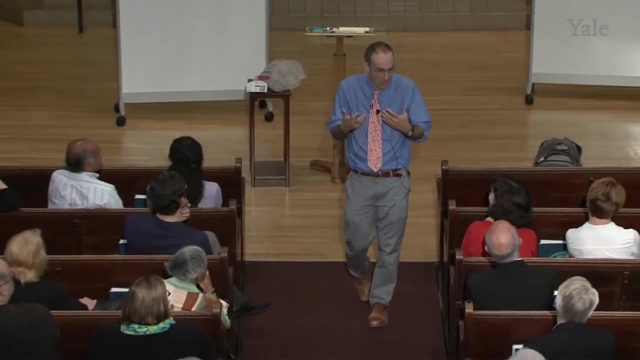 on abilities? It does depend on abilities. So it's very tempting to say: look, I've shown a critical point to shoot here, and this corresponds to when you see the white in the other person's eyes. Not quite true, because when you see, 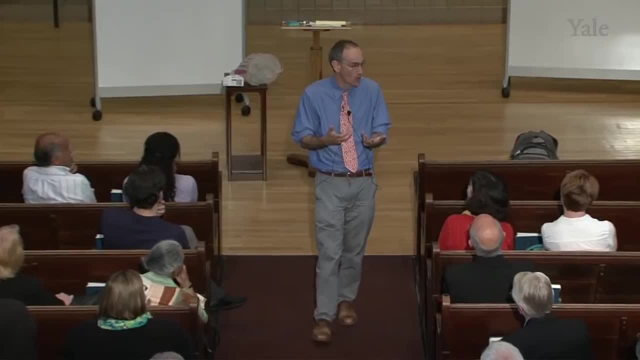 the whites in the other person's eyes depends on your eyesight, and when you should shoot probably depends on both your abilities. So I'm not saying there's a unique time to shoot, but I am saying it isn't a question of who the best shot. 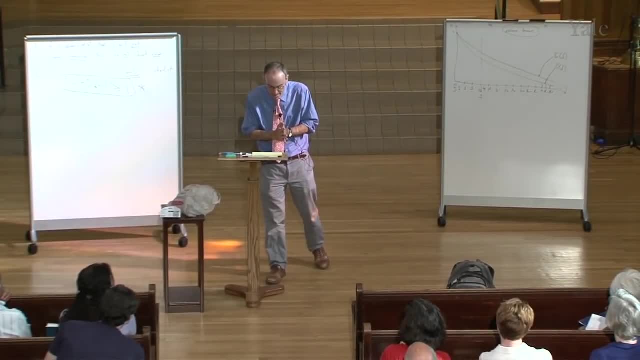 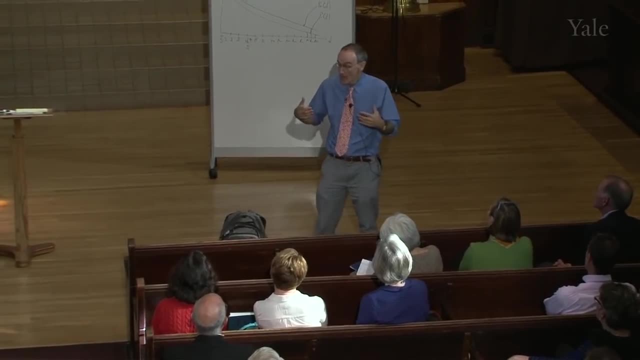 is. it's a question of both abilities put together. Now let's throw in some dust, Let's make this harder. So we now all know that if you're playing this game, you should shoot at D star. if you knew everything, you knew. 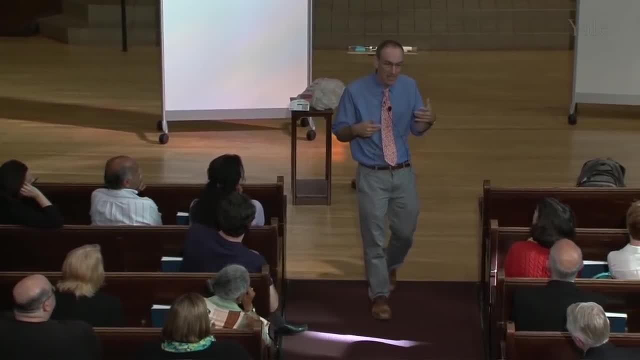 and if you'd taken the course? But you might say, that's fine. but it's fine if I'm reasoning, I'm playing this game against another person who's in the room, who's taken the course. but what if I'm taking the? 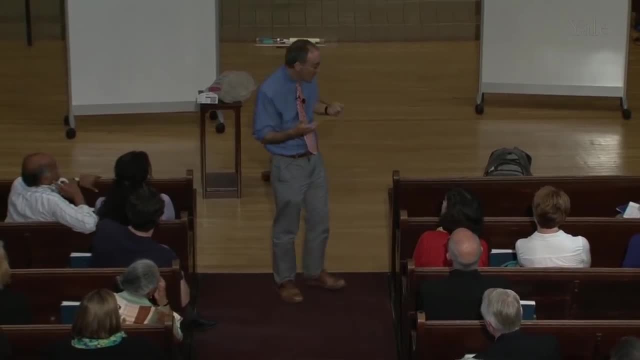 what if I'm playing this game? you know it's life and death. it's Jägen and Lemsky. neither of them took the Game Theory class. It's as far as I know. they didn't take the Game Theory class. 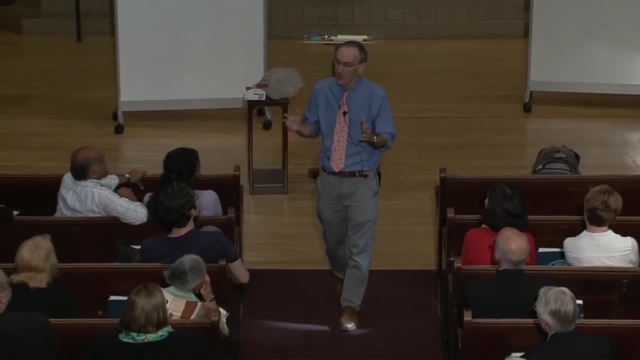 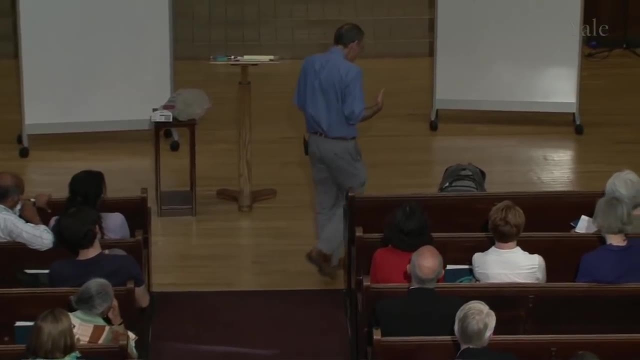 I'm looking around for a Russian scholar. I see a German scholar, but not a Russian scholar. But as far as I know, they hadn't taken a Game Theory class before the beginning of Jägen. And you might think: what if I'm playing against somebody? 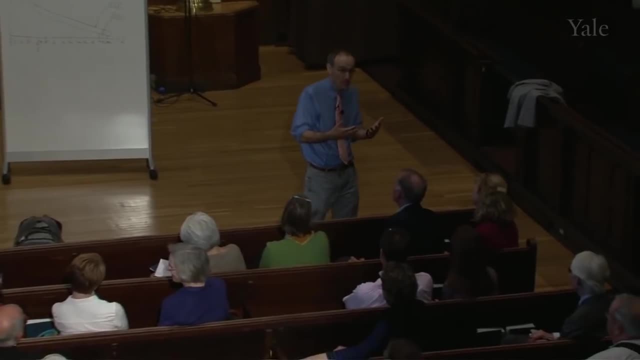 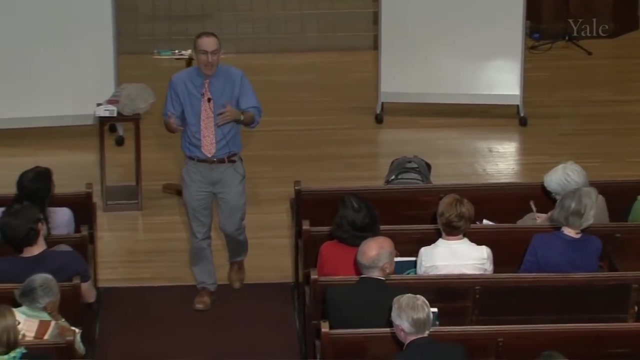 who's a little crazy. So what if I'm playing against a crazy person? I may have gone to Yale, but I could be playing against somebody who went to Harvard Who never had a chance to take a decent Game Theory class. So 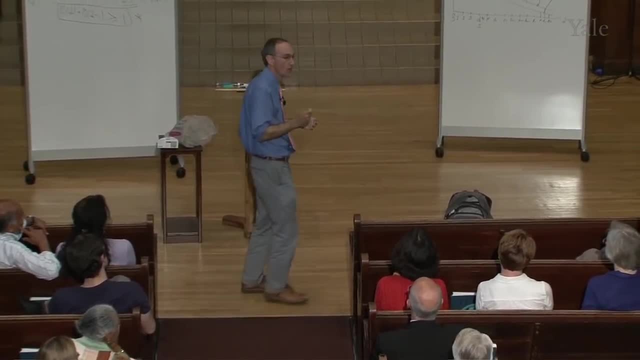 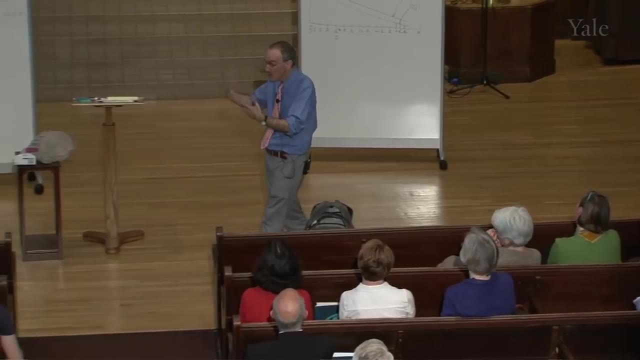 how would it change our argument if I thought the other person was a little crazy? Let's still assume that we know each other's abilities, but now I suspect the other person just isn't capable of reasoning through in the way we just did. How does that change the argument? 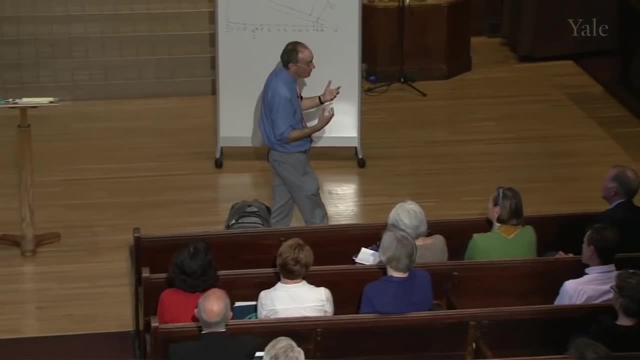 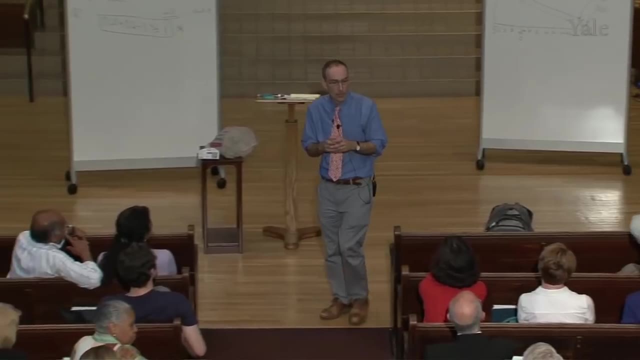 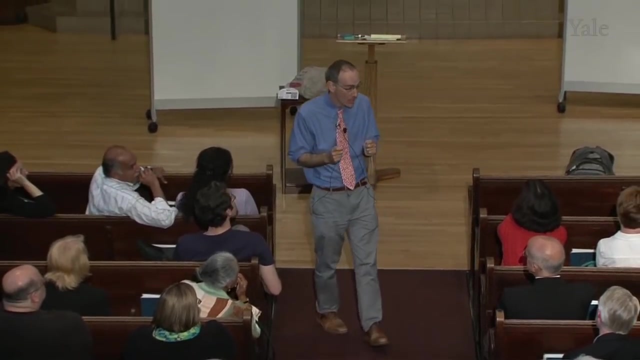 Would that make you shoot earlier? Would that make you shoot later? Would that make you? What do you think? Good, Good. So, even if you're playing against a crazy person, even if you're not confident in the other person's, 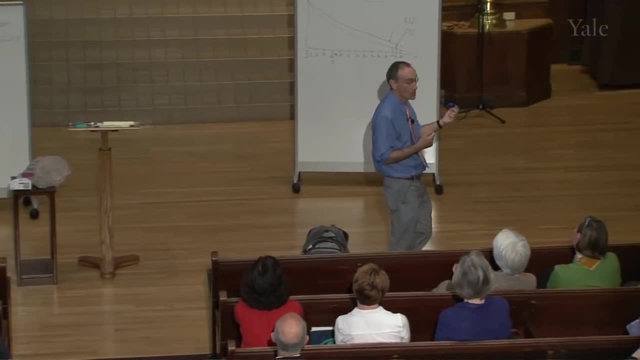 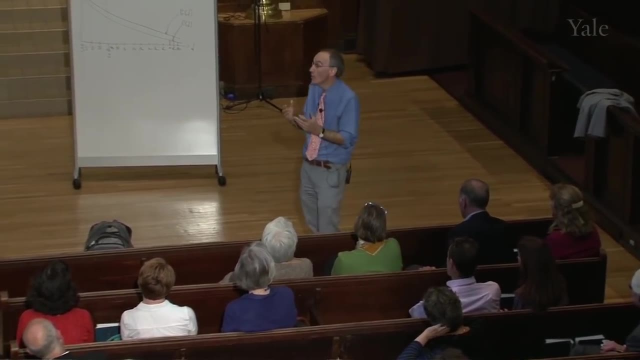 rationality, or even not confident in the other person's confidence in your rationality or any other such statement of that form, which is often true in the real world, even in that circumstance where you don't know you're playing against a sophisticated person. 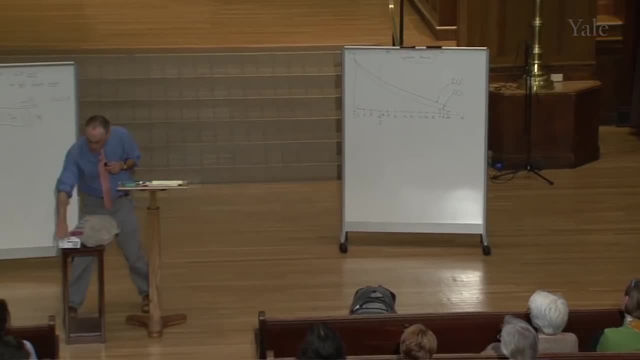 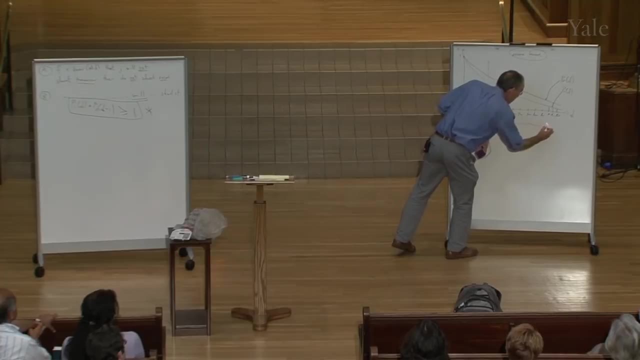 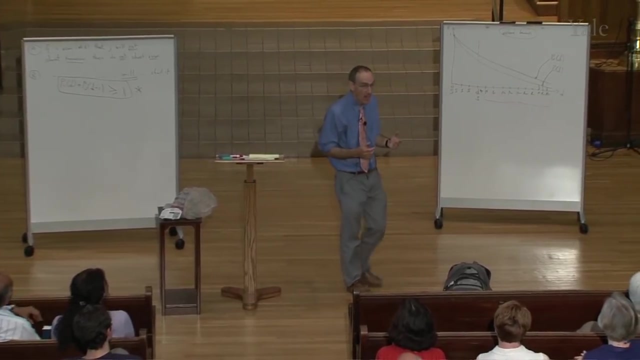 it doesn't change the argument. it doesn't change the argument in here, It doesn't change this argument And it doesn't change that argument, because that argument was a dominance argument. That argument said: I don't care who I'm playing against. 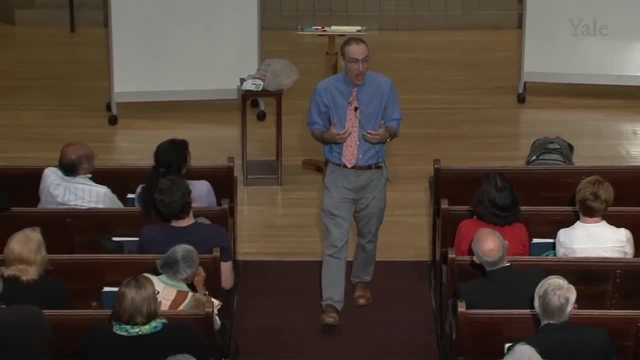 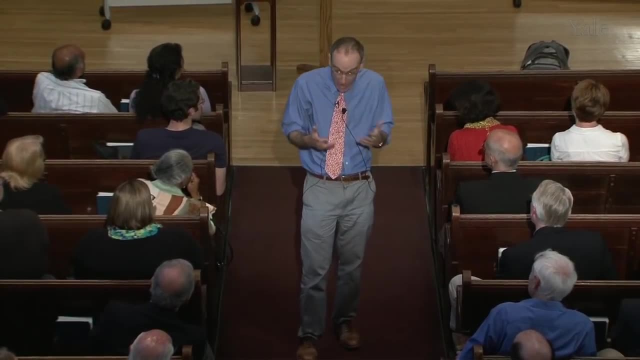 whether I'm playing against a Yale student or a Harvard student, I don't really care if the person's human. The person could be a bollard for all I care. all I care about is whatever's going to happen. I should. 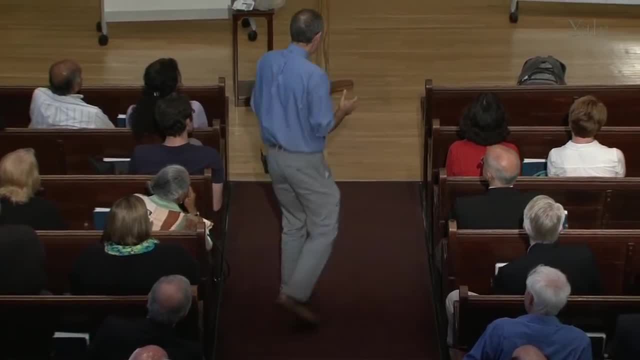 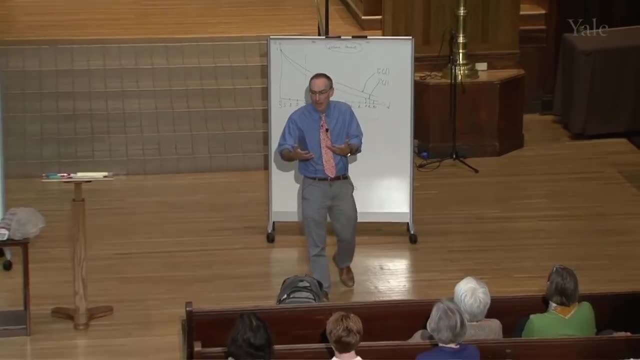 not shoot. therefore I should not shoot. So in the first part of the argument, the dominance part of the argument, there was no interesting thought of the form: if the other guy is rational, if the other guy knows I'm rational, or anything like that. It was just a dominance argument. 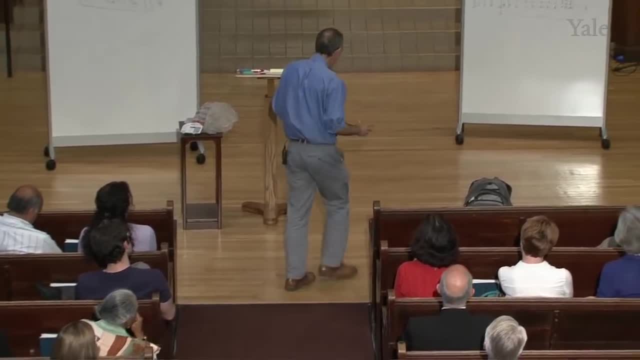 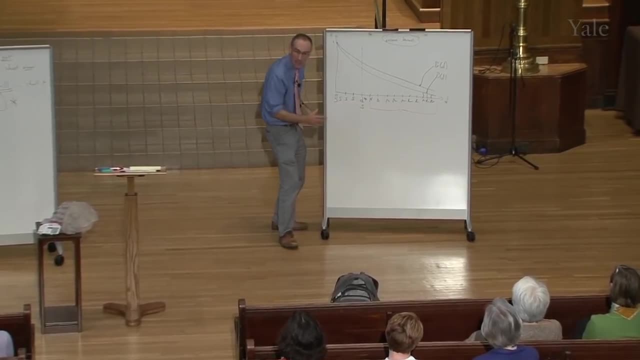 It's an incredibly robust argument. But in here while we were doing the backward induction argument there, I was thinking the other guy is rational and I was kind of thinking that he can figure out that I'm rational or that he can figure. 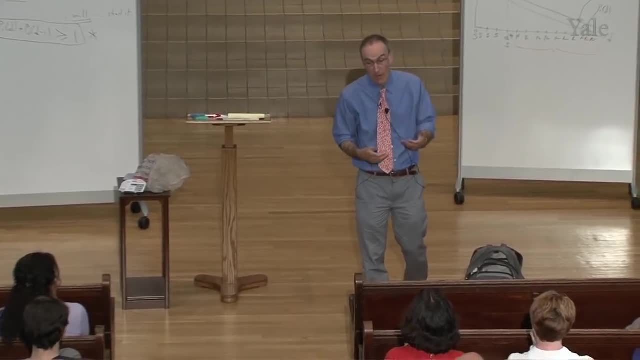 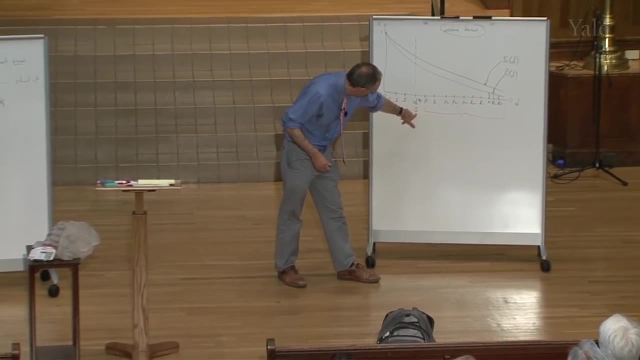 out that I can figure out that he's rational or she right. So it's he and she making it easier. So in this piece of the argument, Robert at d star had to figure out what James was going to do at d star minus one, and that 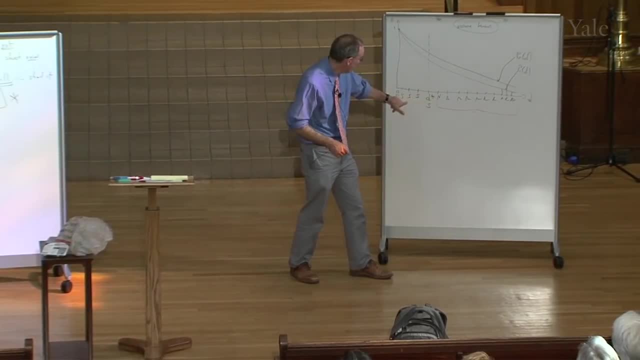 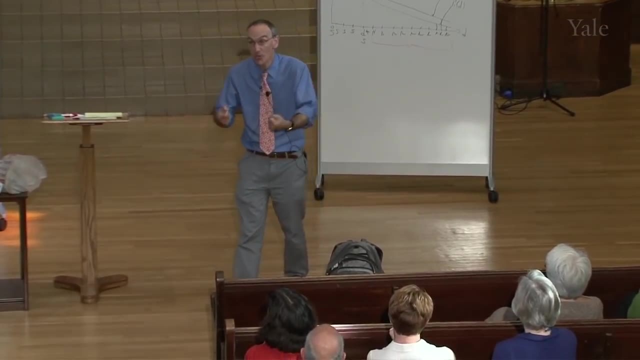 argument required him to have confidence that James would figure out what Robert would do at d star minus two, etc. So not only did it require thinking the other person, putting myself in the other person's shoes and thinking they're rational, it required putting myself in the other person's shoes. 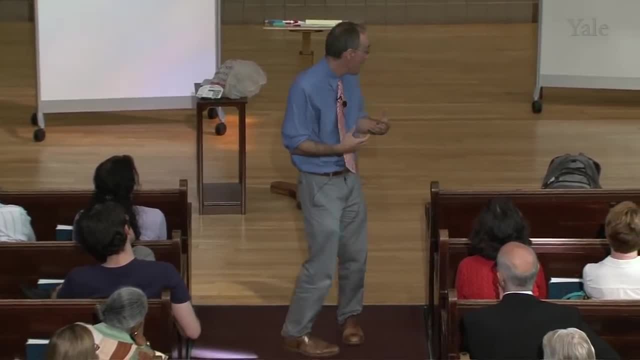 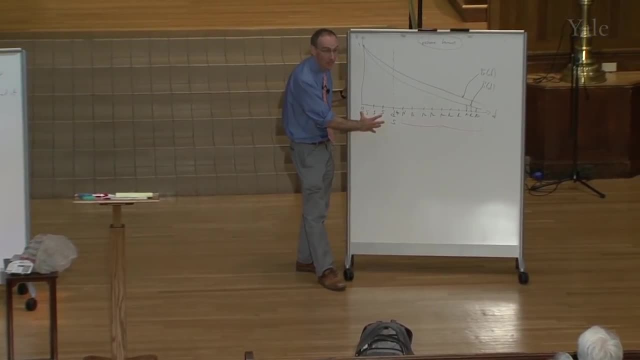 while they're putting themselves in my shoes and they know that I'm rational, and so on and so forth. So this backward induction argument is much more fragile to irrationality. So Laurie Santos gave a talk yesterday about irrationality, which is an incredibly important topic these days. 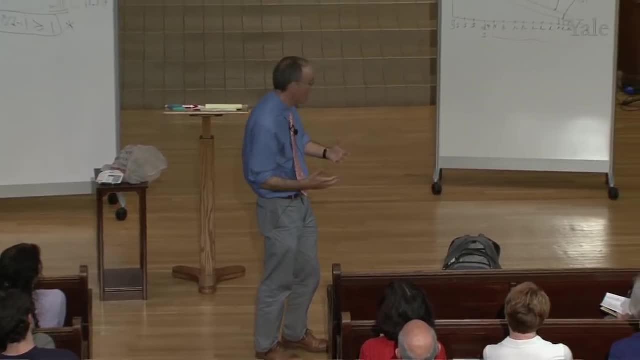 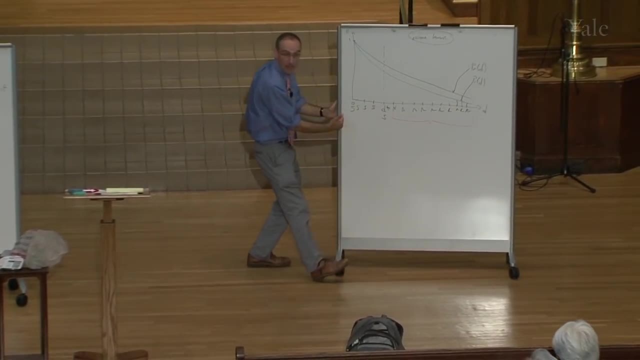 It's possible that on Monday they might give the Nobel Prize in Economics to Robert Shuller, who's worked on such topics in finance. Irrationality here doesn't affect this part of the argument. it does affect this part of the argument. 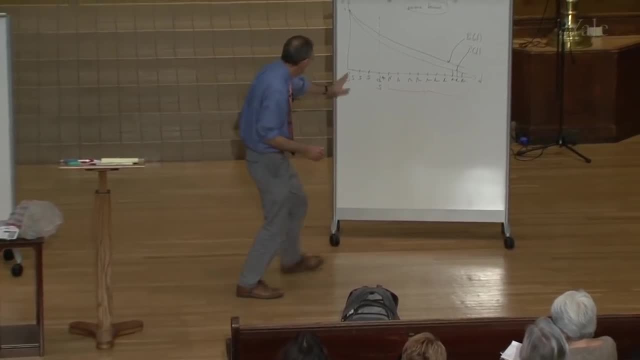 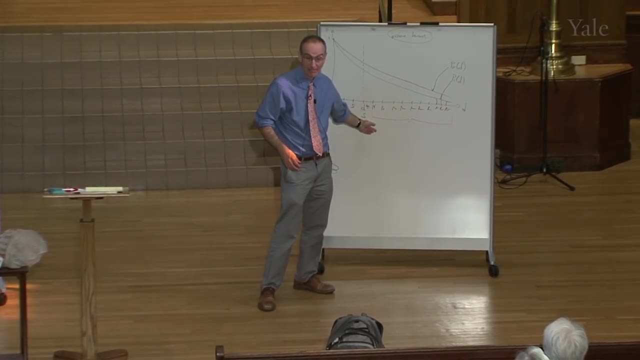 Now, nevertheless, the fact you should not shoot before here is a pretty strong argument because, frankly, by the time you've figured out the other guy's irrational, it's too late. You don't really care if he shoots early here. You're perfectly happy if he shoots early here. 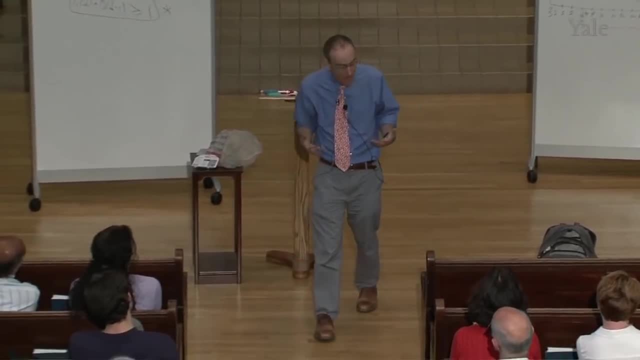 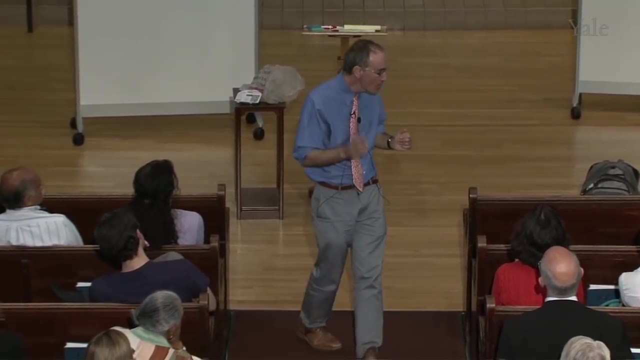 So this argument, this particular example, even if the other guy isn't rational, I shouldn't shoot before d star. Now let's push that idea further. I've played this game in class with undergraduates. I've played it in my business school class. 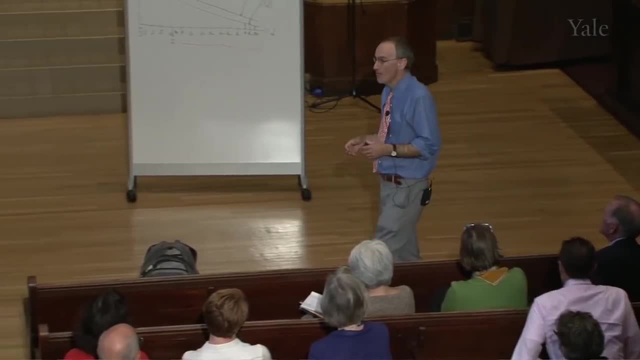 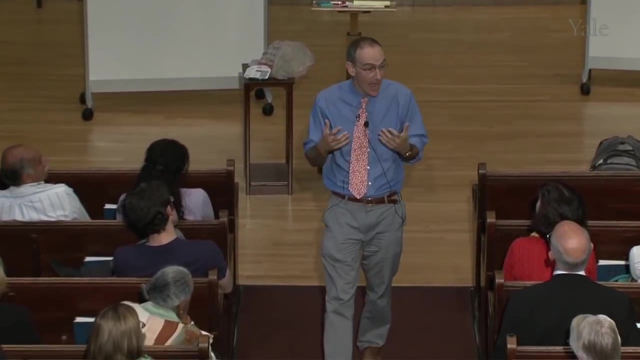 with business school students, I've played it with parents, I've played it with alumni, I've played it with deans, and so I have some idea about how people do on average in this game. Now, assuming that people are following the reasoning I just said. 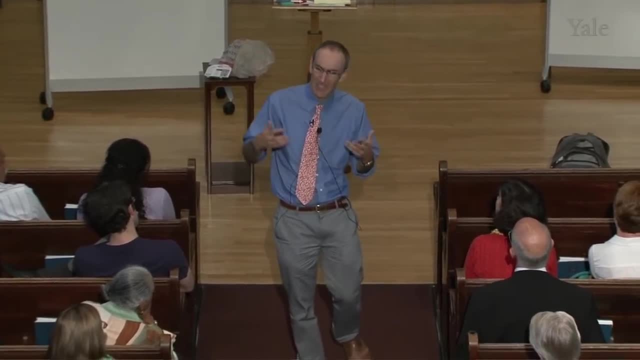 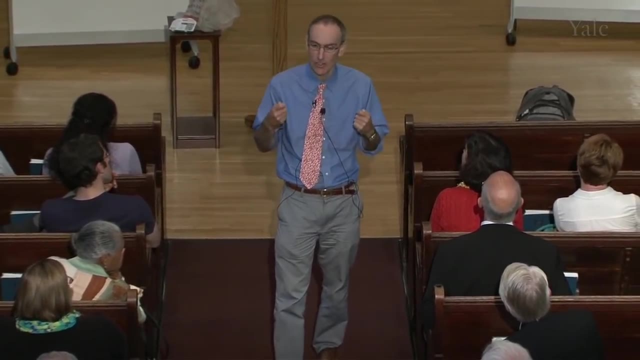 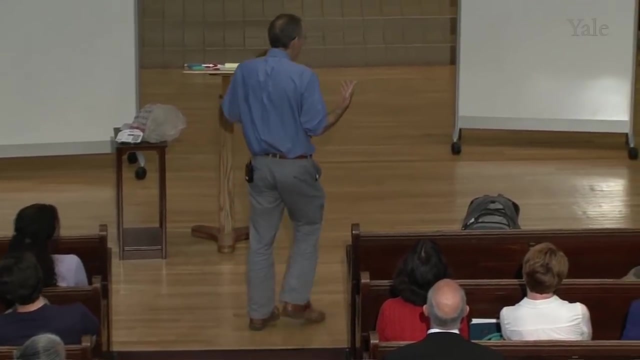 and assuming that ability is distributed roughly randomly, and also making this somewhat unreal assumption that people know each other's abilities. how often should I, how often do I expect to people? how often do I expect to see people hit on average? Well, d star could be the weaker. 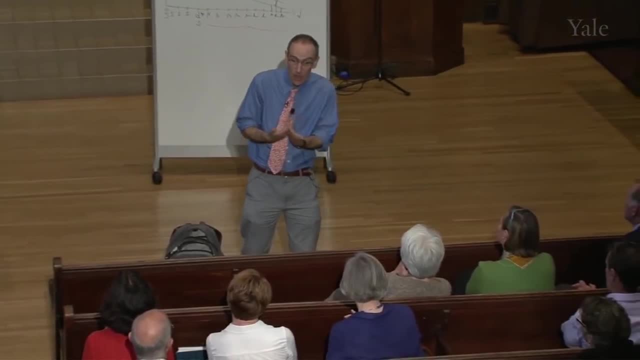 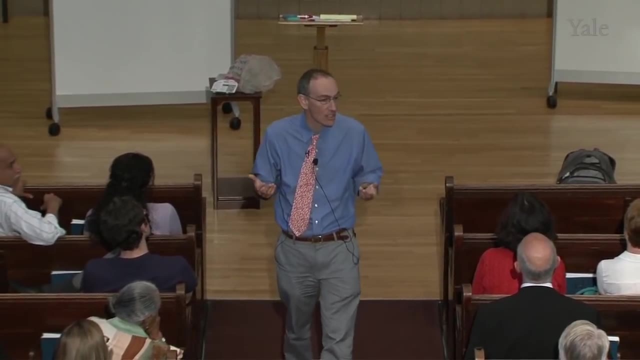 person shooting. it could be the stronger person shooting if it's happening at d star. one is the sum is one On average. how many hits should I see? Fifty percent. So if I get a large enough sample, there's a bit of hand waving in that argument. 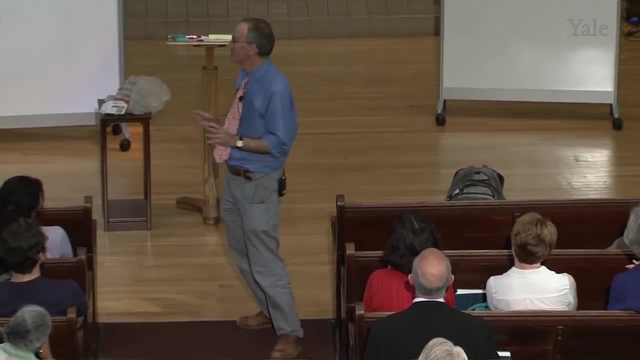 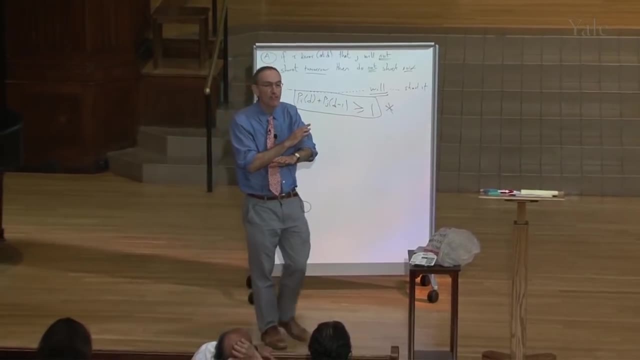 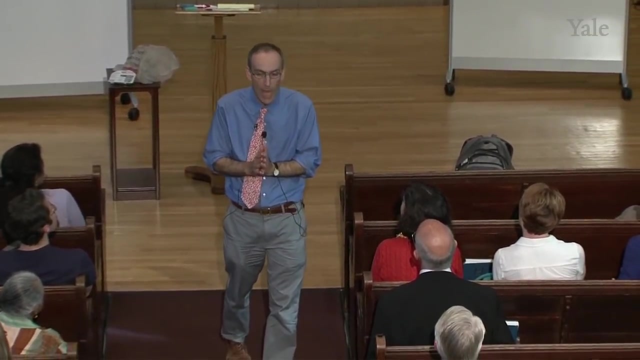 someone's going to point out. allowing me a little bit of hand waving: discrete versus continuous. roughly speaking, fifty percent should hit. I see far fewer than fifty percent, Massively fewer than fifty percent, I would say. I see ten percent hits Why. 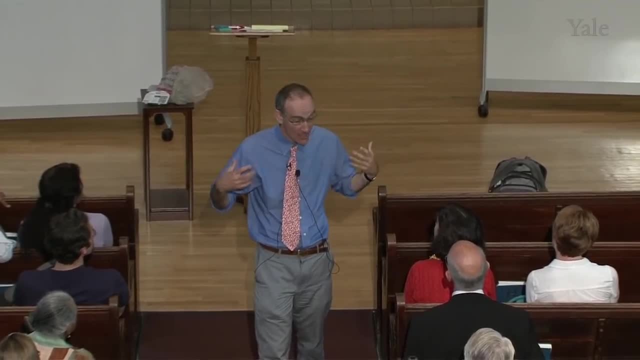 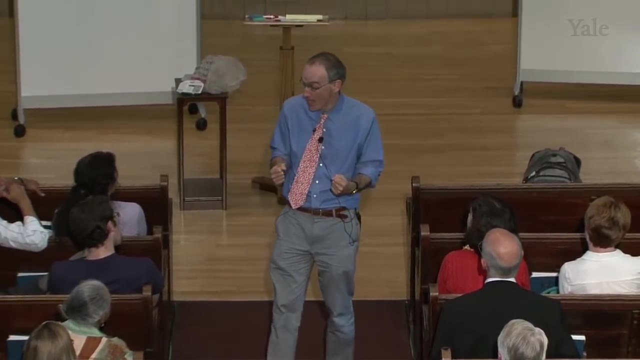 Why do I see ten percent hits, when we just agreed that, even if everyone's crazy and irrational, no one should shoot between them before d star and d star's telling us that half the shots should be hits? Why do I see such a low hit? 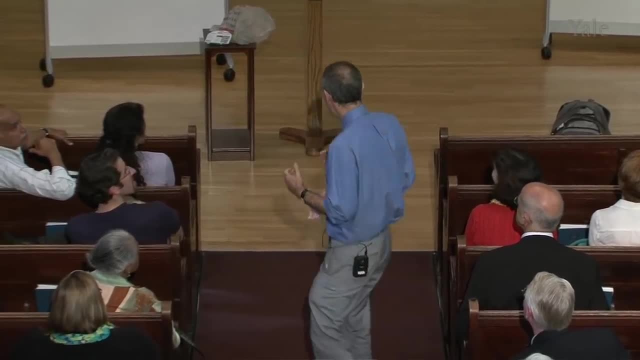 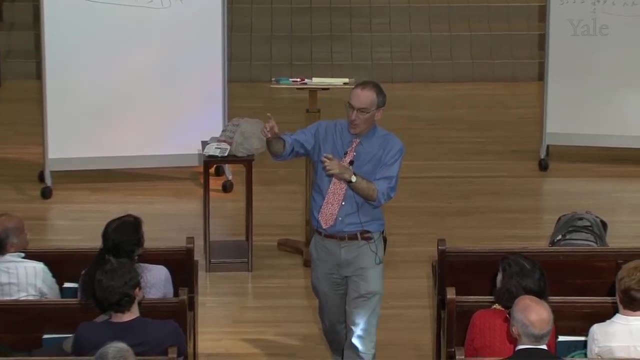 People are unexperienced and untouched punters, although that might make them shoot later. I mean, you know in some sense, Right? so I think there's two things going on. Let me take them in turn. So I think people do two things. 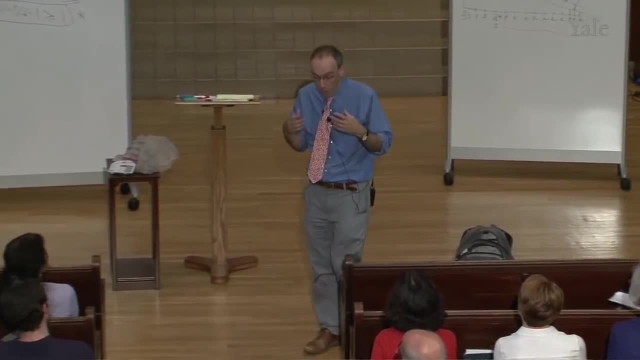 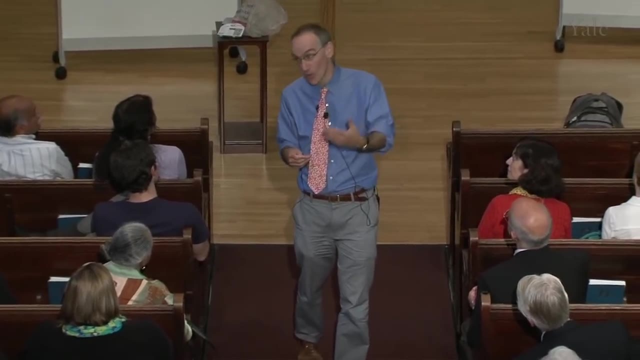 They overestimate their opponent, they also overestimate their own abilities. So there's a well-known psychological bias that people overestimate their own ability to do something. They probably also overestimate the other person, but they certainly overestimate their own ability to do things. 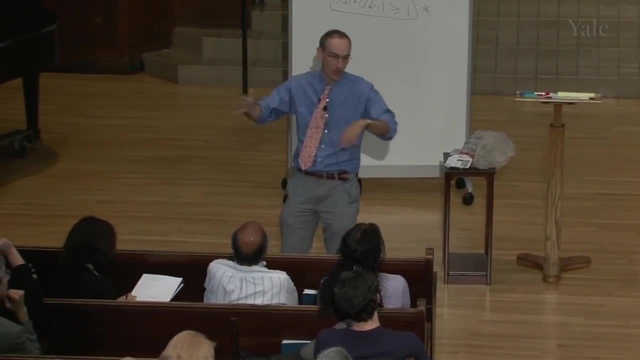 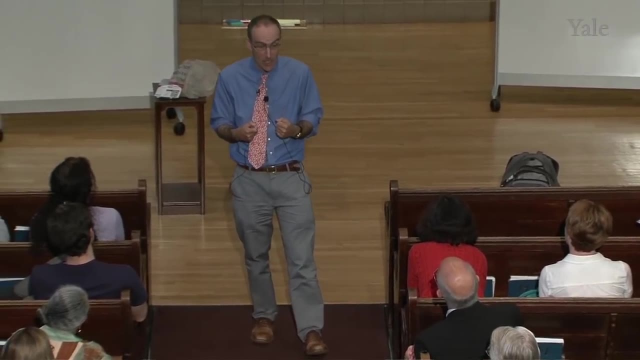 So there's an overconfidence bias and there's stacks of literature on the overconfidence bias. So if you Google overconfidence and start reading papers, you can be there a long time. So it's pretty well established that people are overconfident in their abilities. 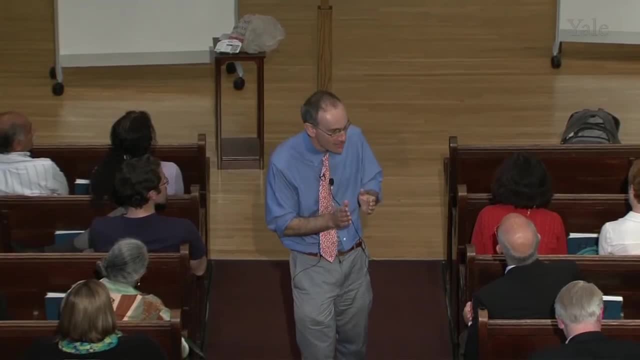 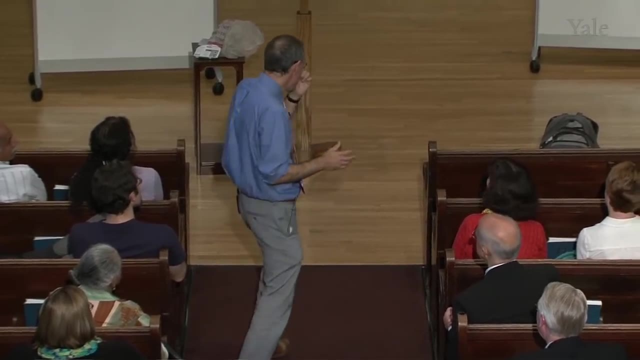 Amateur golfers will try that shot, which they've seen Tiger Woods do, where he slices it between the trees. I don't play golf, but I'm told amateur golfers are never going to hit that shot. Actually, I don't know the answer to that, Meg. 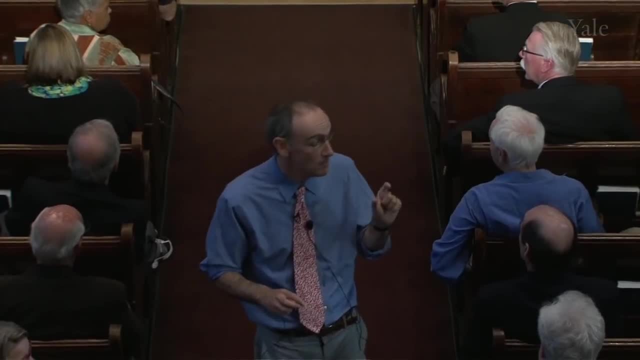 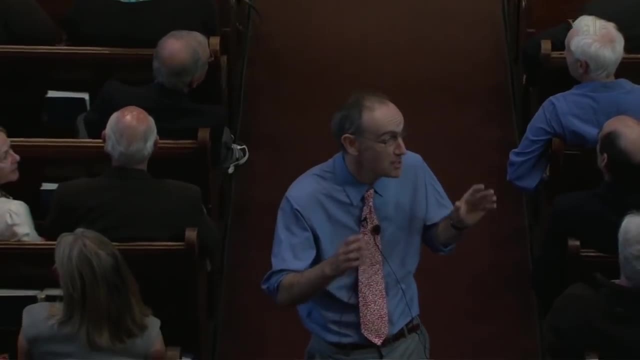 It's possible. There probably is literature on that, because almost all these things have been tried with gender in there. If I had to have a guess, I would say men are more overconfident, but I don't know the data. I have the same suspicion you have. 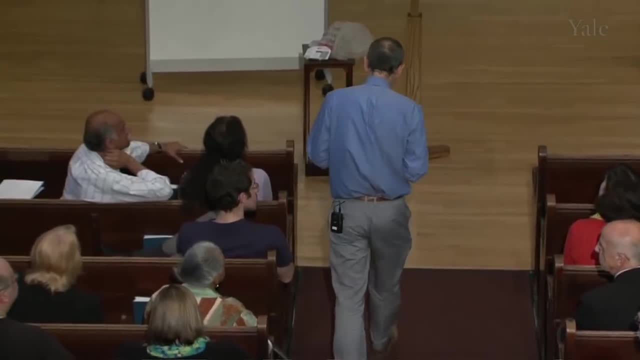 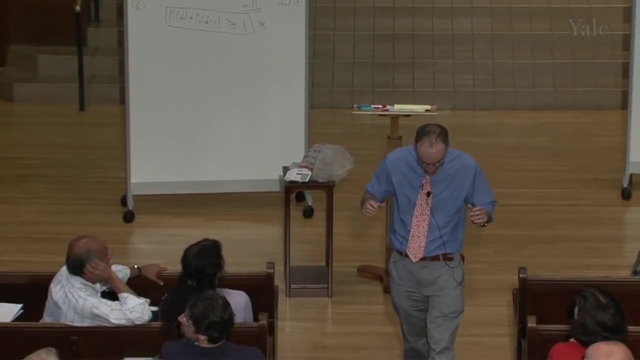 So one thing is overconfidence. That's a well-known bias. I think there's another thing going on here, and I think it's going on specifically in America, and I think Paul's saying there's another thing going on here. I think that at least in America, 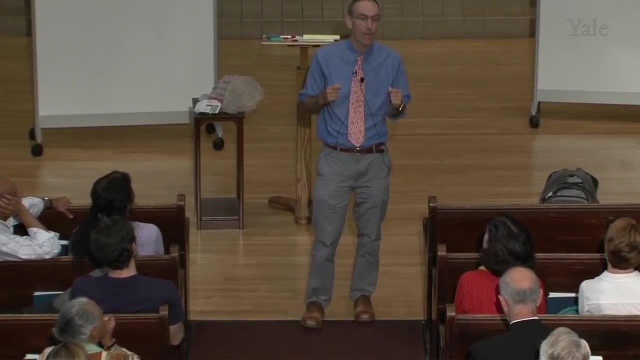 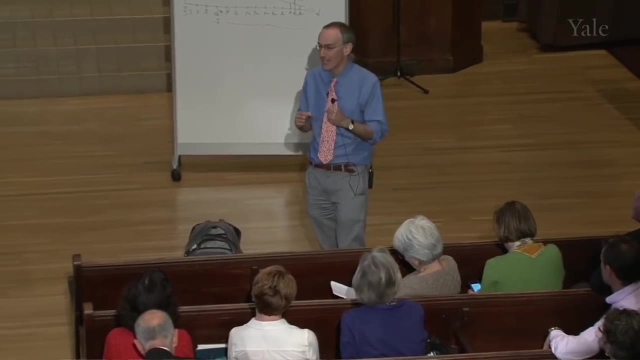 there is a thing I want to call the proactive bias. People like to be proactive. When you're kids in America, you are taught that being proactive is a good thing. I know this because I have kids. I have a 10-year-old and an 8-year-old. 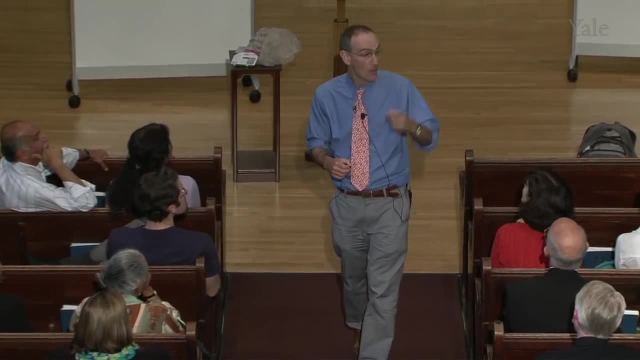 I have a 1-year-old too, but he hasn't gone to school yet. My 10-year-old and my 8-year-old- both who are girls- are being told being proactive is good. Seizing the bull by the horns is good. 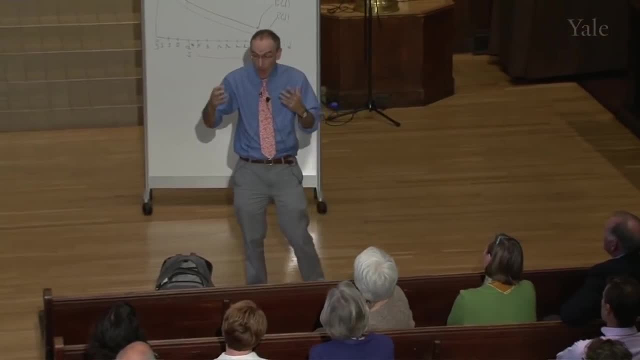 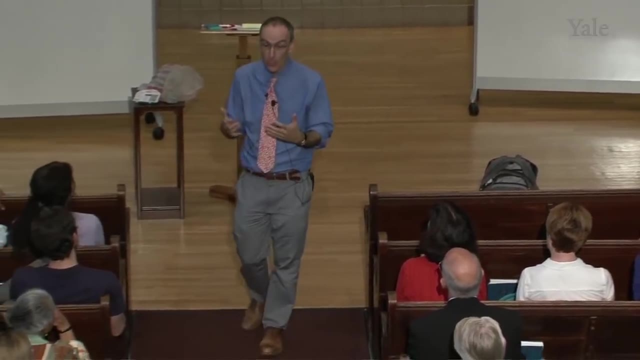 I also have more evidence about this. Just to make it clear: being proactive would be throwing the sponge. when things happen to you, People think being proactive is good. You see this on SportsCenter. You'll see these guys in the sweaty. Usually it's guys. 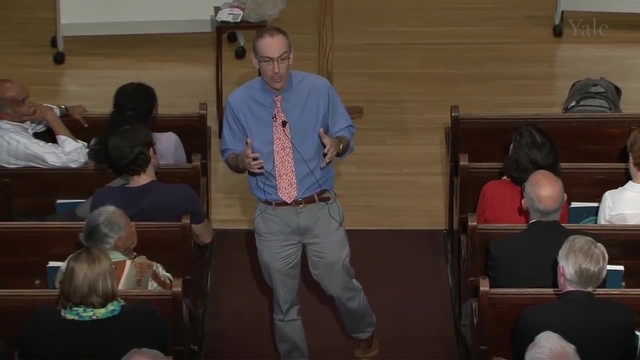 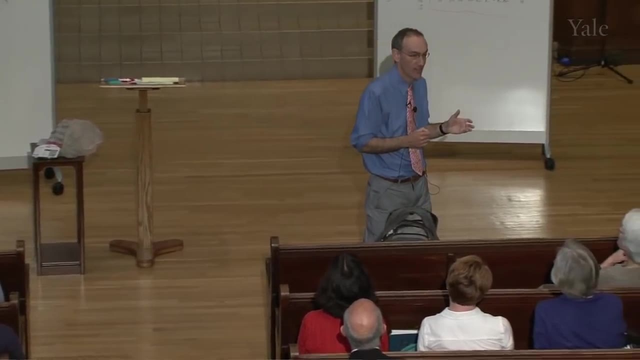 I don't want to be sexist about this. I think it's males or females. They make this statement and they say it's great because we control our own destiny. Coming from England, controlling my own destiny sounds kind of scary to me. 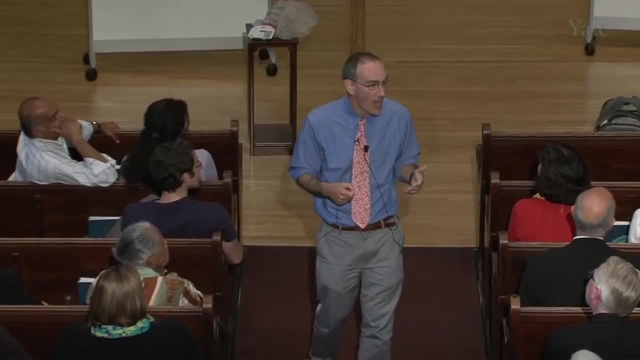 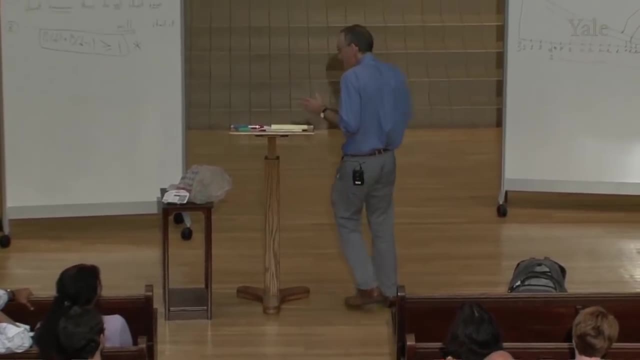 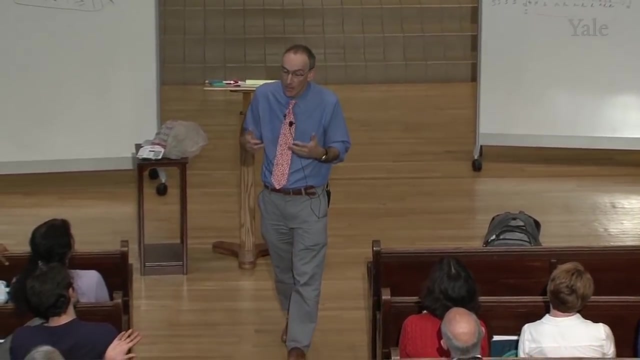 I have to say, if I could control my own destiny, I wouldn't have got married. I didn't say that I worry that this proactive bias causes people to throw the sponge too early. Taking the bull by the horns sounds like a good idea. 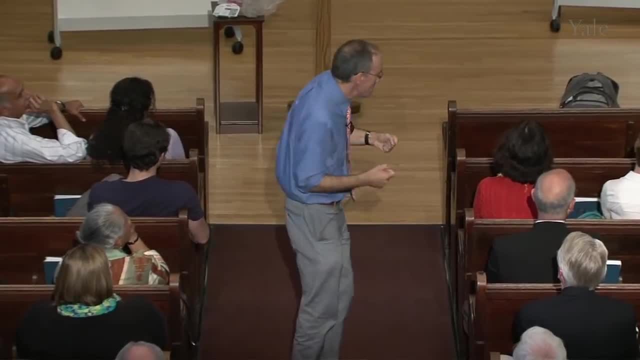 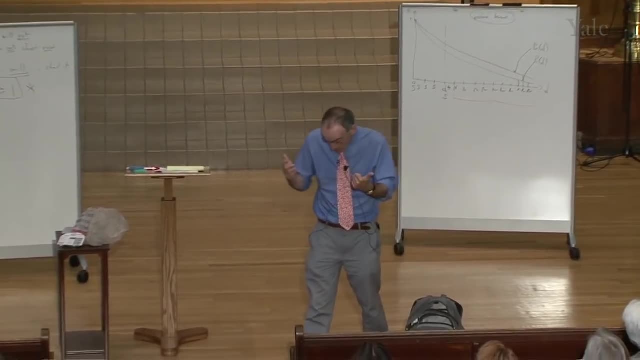 but when you think about it, running away is an awfully better idea. If I have one last lesson for you, what are the takeaway lessons from today's talk? Let's go through them. One is dominance arguments. I won't rehearse what they are. 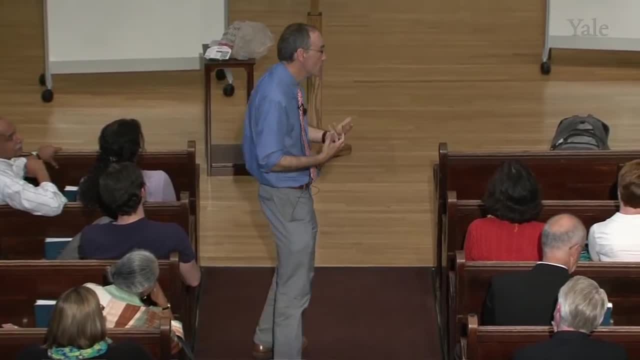 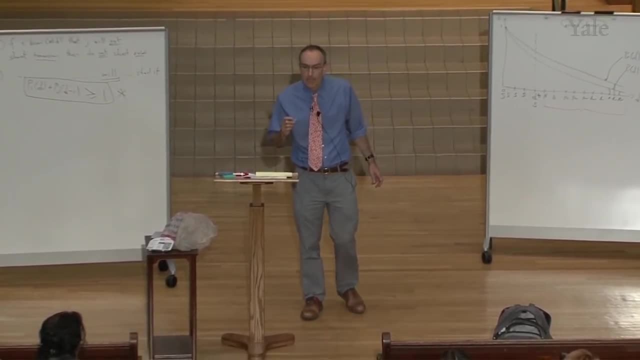 The second is backward induction. Sometimes it's worth going to the end of the game and working backwards. And the third is this- and it's really just for the Americans, because I think the Europeans in the room don't make this mistake: The point is not to go down swinging. 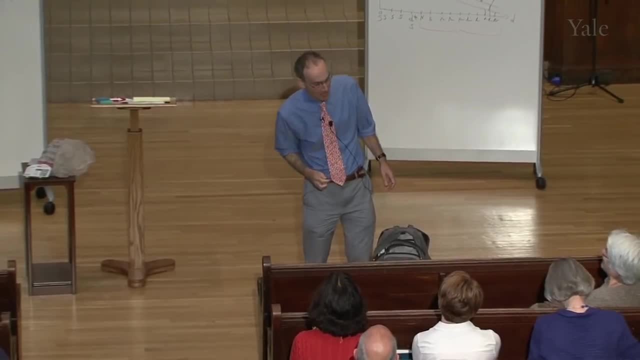 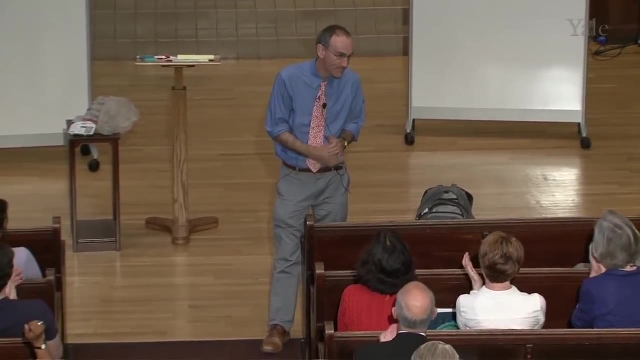 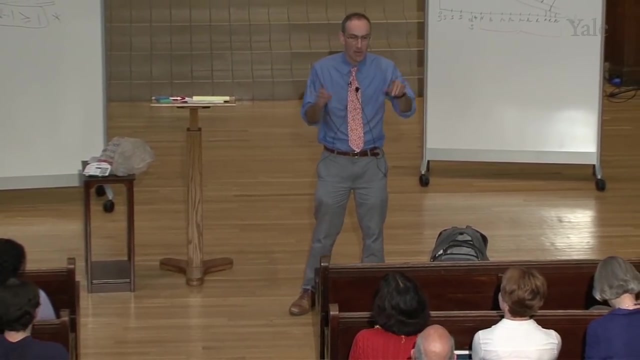 The point is not to go down. I'll leave it at that. I'm done, Thank you. I can take a few minutes questions, but I want to make sure you make it to the next talk. I have one game I have solved completely. 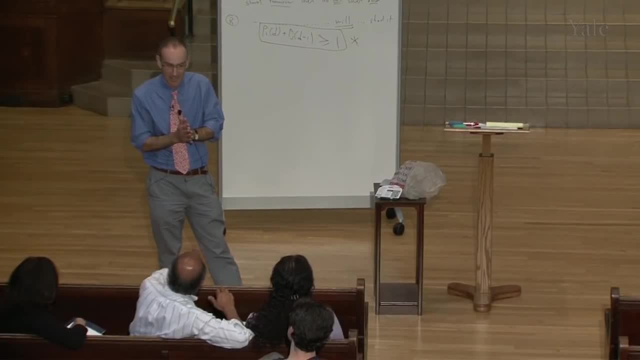 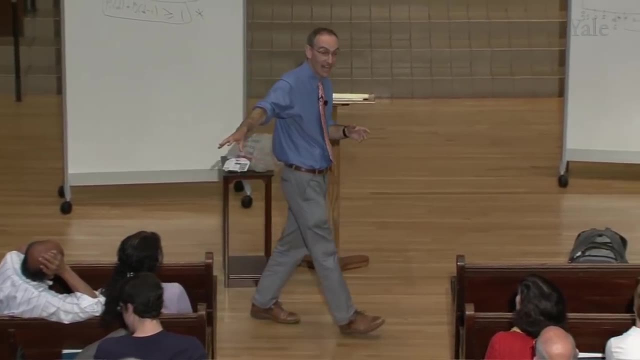 If the opponent is Gandhi, then I know he won't shoot. That's right. So if it's Gandhi, you just wait and plunk it on his head. So the question was: what if you're playing against Gandhi, So Gandhi's not going to shoot you? 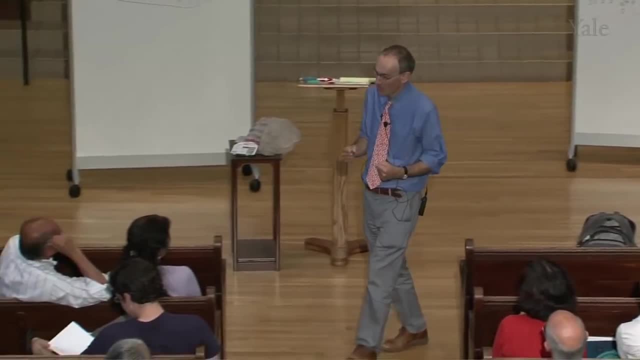 but if you were going to win the game and you are so inclined, Shankar's a cynical kind of guy- he'd just wait and plunk the sponge on Gandhi's head, An image I'm now going to have when I go to bed tonight. Do I like the casino? I never go to a casino. Yeah, I don't really like it Out of interest. I'm not a big casino player. I kind of like playing cards. I mean roulette wheels seem a little bit too. 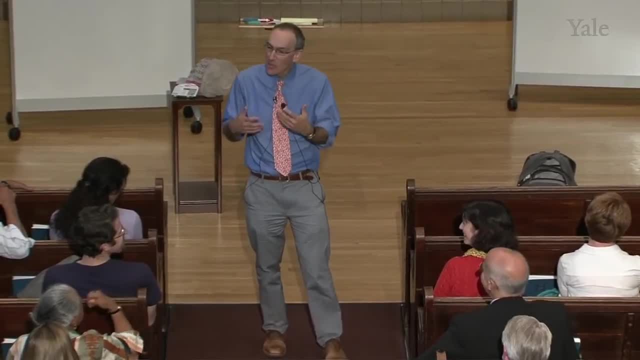 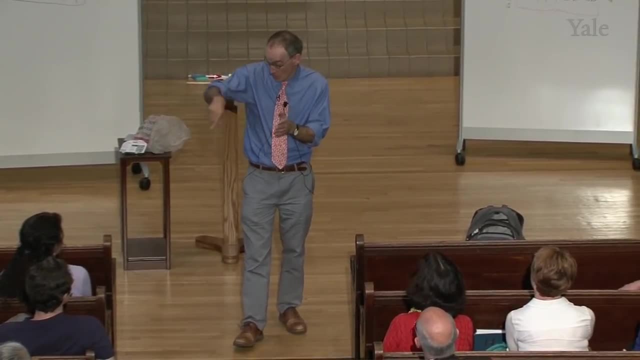 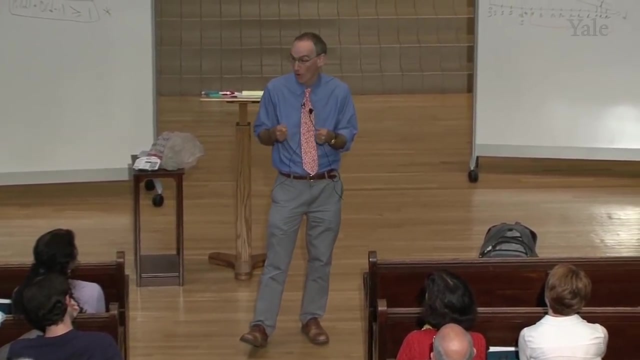 random to me. I worry a little bit about irrationality in the casino. So I had a student once who was studying behaviour in not roulette, but in 21. And it turns out that people do exactly the wrong thing there. They 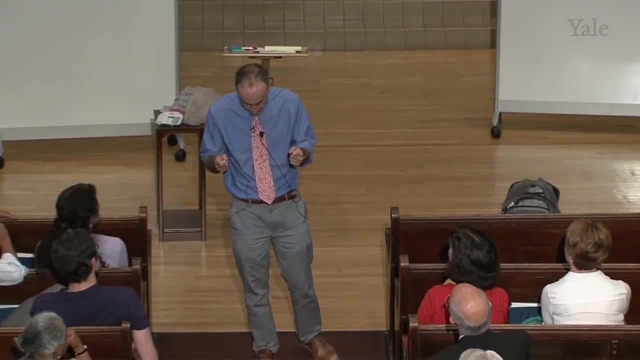 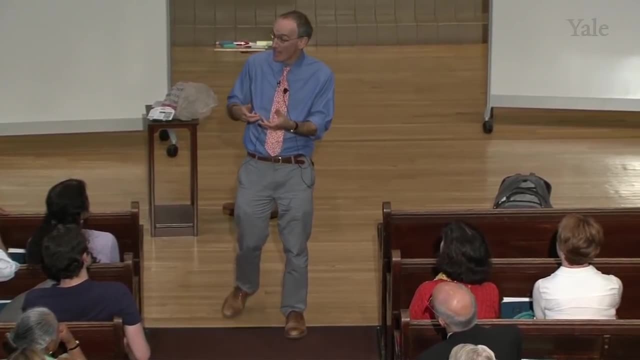 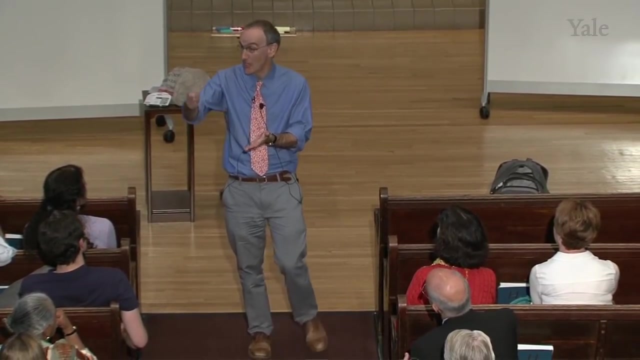 what do they do? They quit when they're behind rather than quitting when they're ahead. And it turns out, since you use five-packs- and it isn't a random sample- in doing well, any sensible updating will say you're going to do worse in the future. 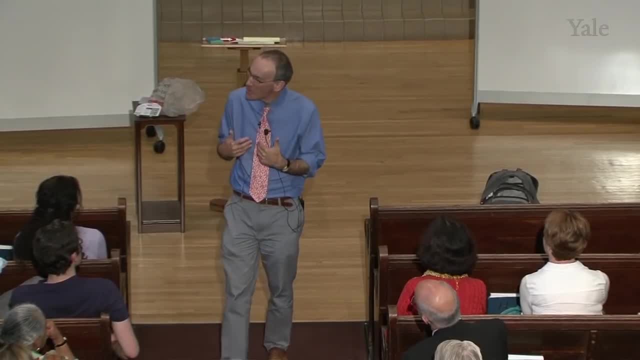 If you're doing badly, you're actually going to do better. There's actually a regression to the mean, So people do exactly the wrong thing And I'm scared I would do the wrong thing too, And my wife would not like it. 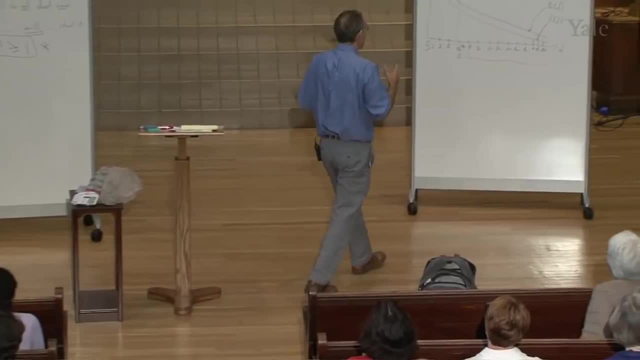 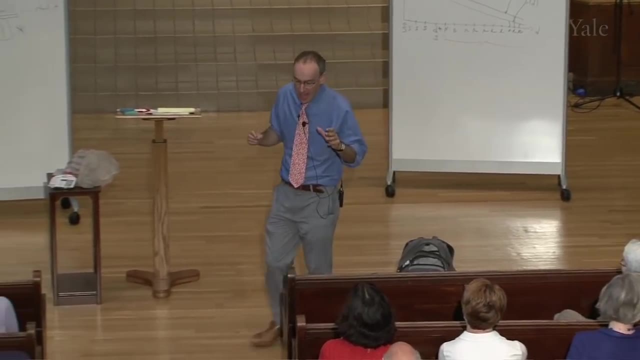 That's a good question. So the question is: can we see games like this in nature? So let me, as a politician, let me answer a slightly different question. So game theory is enormously used now in biology. In behavioural biology it's a major tool. 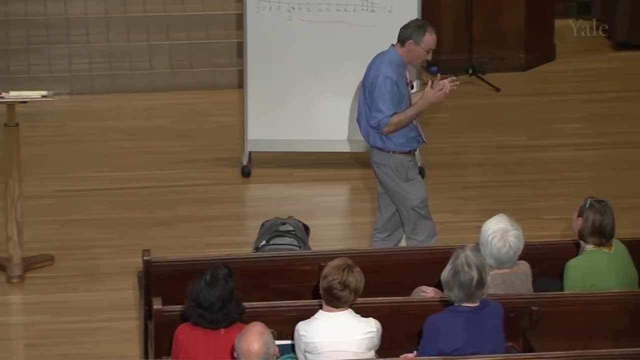 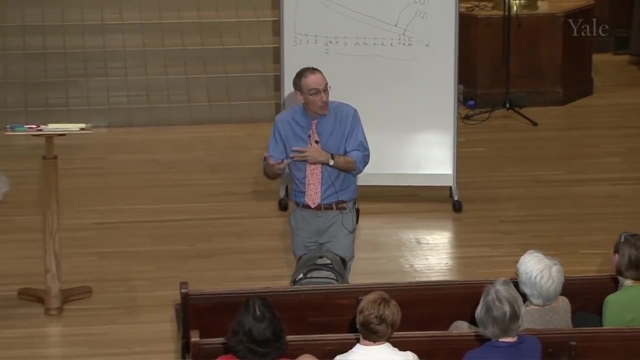 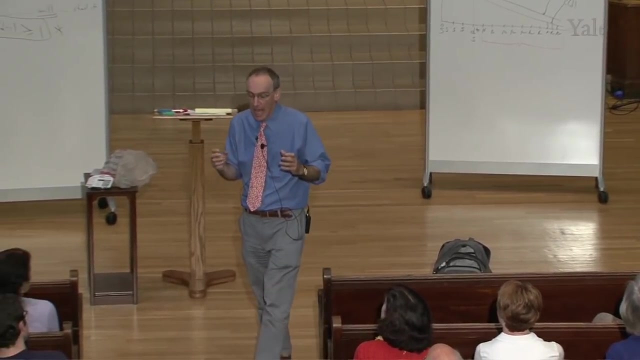 And it turns out that there are wonderful connections between the game theory we developed in economics and notions of equilibrium in economics and notions of evolutionary stability in biology, And they're not exactly the same idea, but one is kind of a subset of the other. 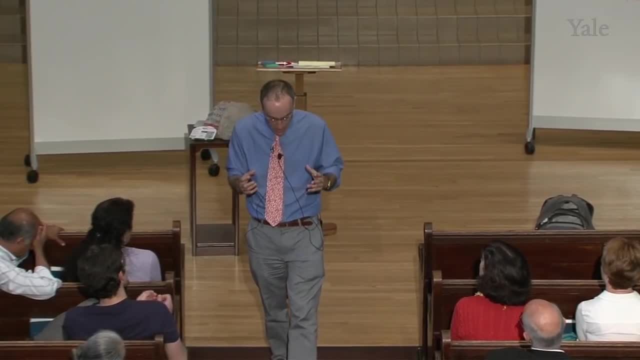 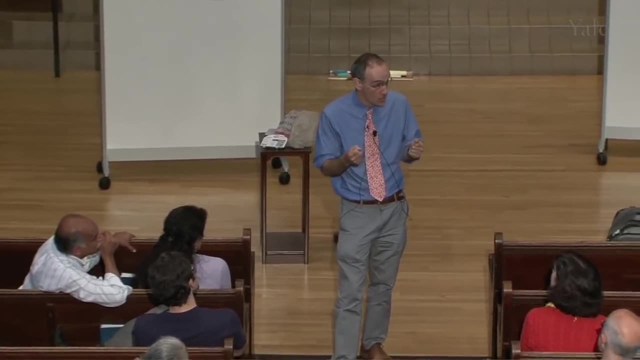 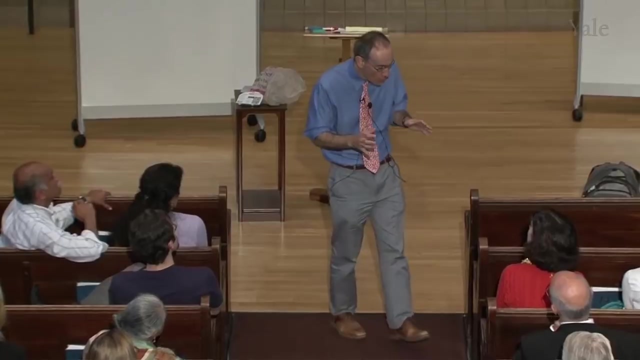 And what you can do in evolutionary biology, which is kind of cool, is if you know the basic form of a game that a particular species is playing- and be careful because the actors now aren't rational, it's gene selection- but still if you know the form of the game. 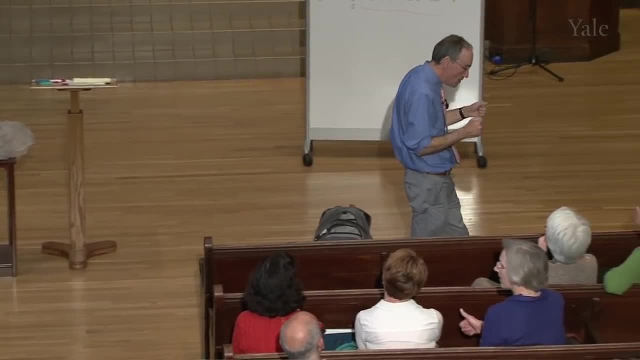 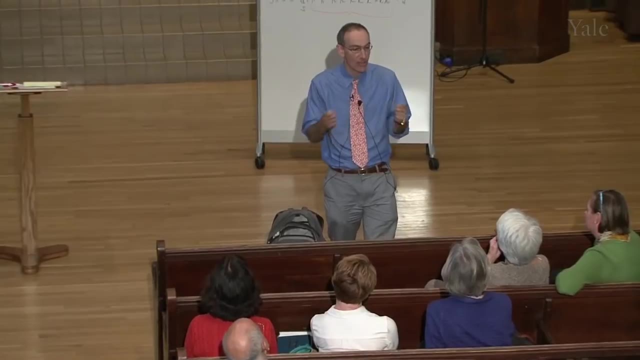 but you don't know the exact payoffs of the game. you can actually look at the behaviour. look at the behaviours you see in the population and back out what the exact payoffs must be, Which is a lovely example of what's called 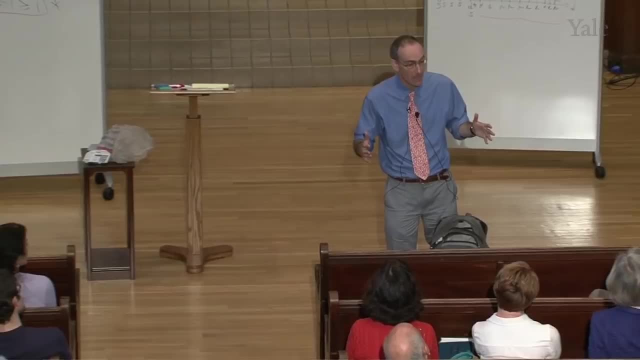 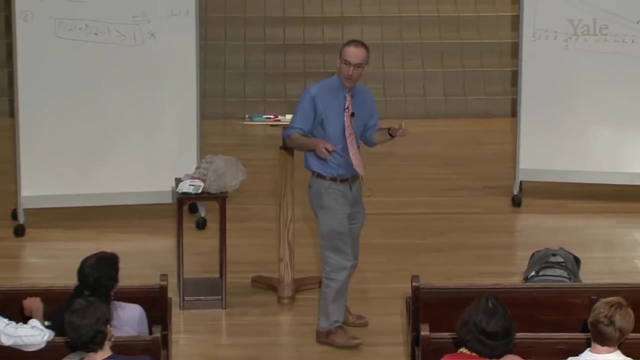 identification in economics. So biologists do incredibly cool things with game theory. Actually, at this point they do cooler things than economists do with game theory. it's really cool Now this particular game, I don't know. there's some biologists in the room. I'm looking at Tom. 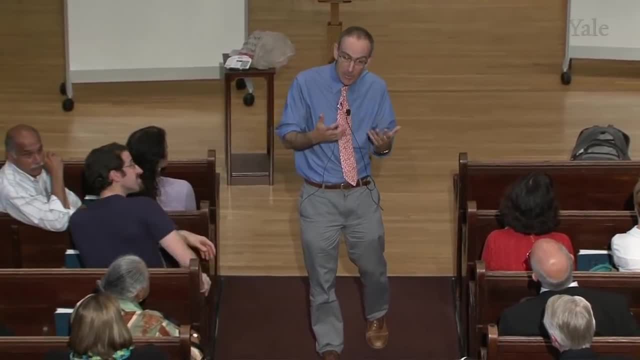 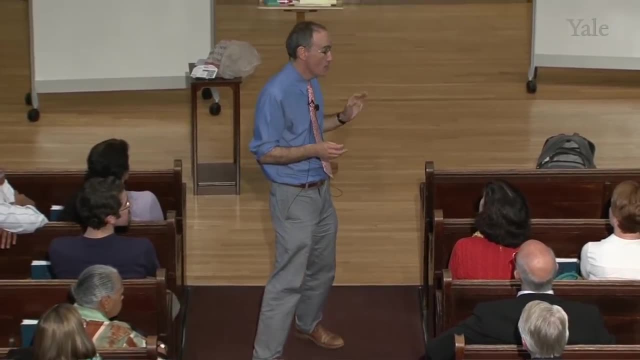 I don't know exactly what game this would correspond to in nature, but there are games that a better example for nature is the game rock-paper-scissors, Rock-paper-scissors, So rock-paper-scissors. everyone know the game. rock beats scissors and scissors beats paper. 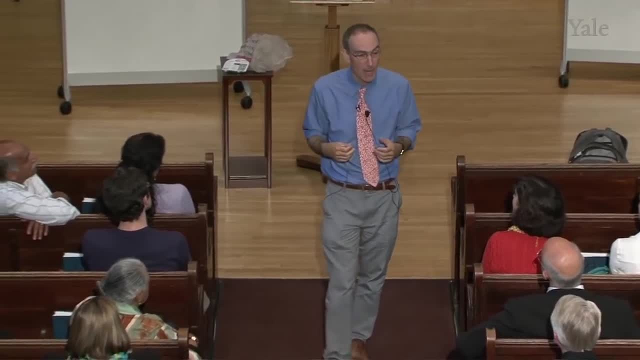 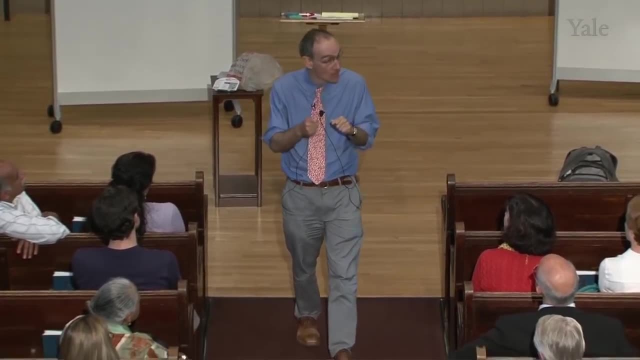 and paper beats rock that game. So rock-paper-scissors is a nice little zero-sum game that you can find examples of. it looks a lot like that in nature and you can twiddle them a little bit, so not exactly rock-paper-scissors. 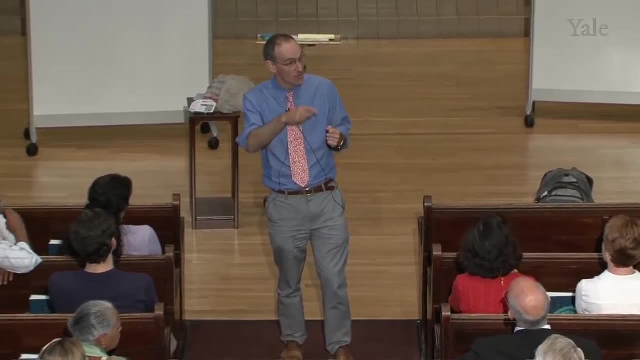 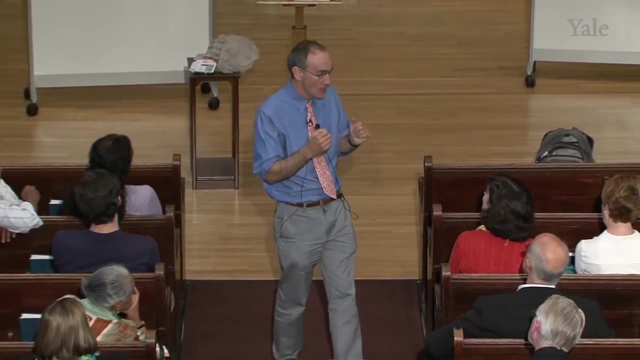 and they actually have no evolutionary stable point and you can show in examples of that, cycles occurring in populations of- actually the most famous example is tree lizards, mating behaviour of tree lizards- and you can show, you can predict out from those cycles what the exact payoffs. 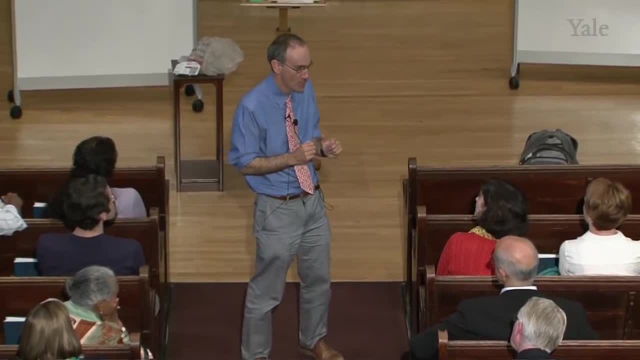 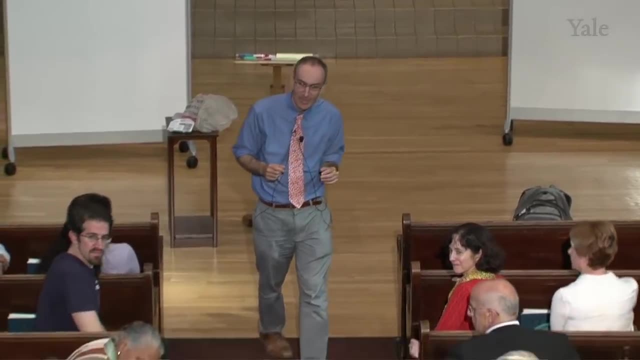 of the rock-paper-scissors game they were playing was. So there are really cool things in biology with this, But Tom knows more about that than I do, so I'm on dangerous territory. Tom, do you want to comment? How do you use game theory? 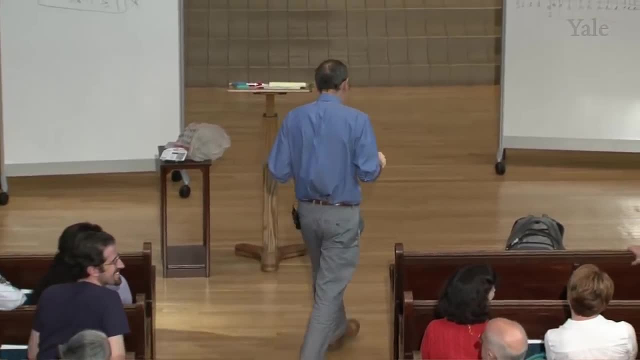 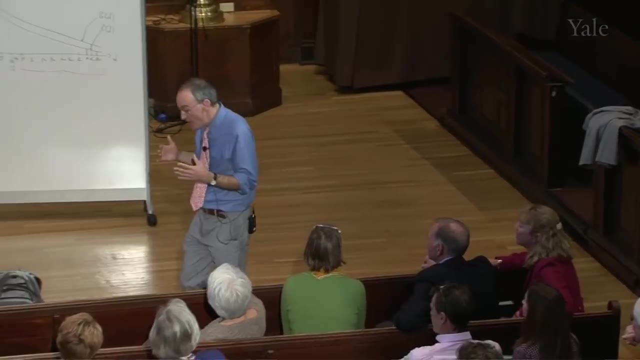 in your day-to-day work as a provost? Ah, How do I use game theory in my day-to-day work as a provost? Yeah, so it's a good question. So I do it a little bit. I think I've been doing this so long. 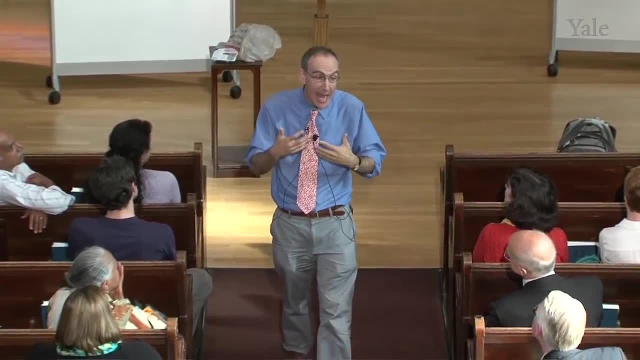 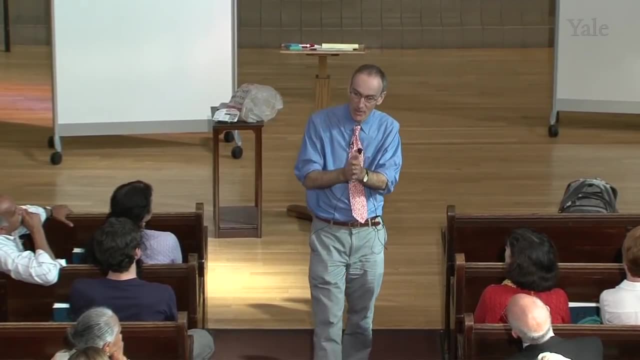 that it's kind of hard-wired for me to think this way. So I do tend to lay out things and I do tend to sort of try to go down one branch of the tree at a time and see if they're all the same. 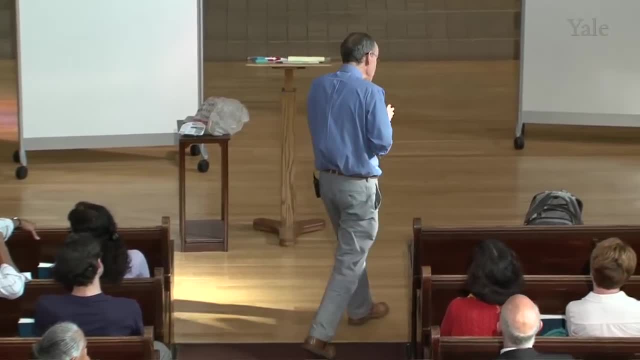 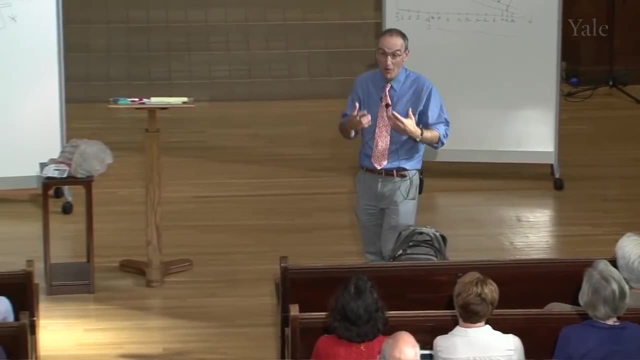 if there's a dominance argument there I can seize hold of. But also a large piece of game theory, as applied to economics or to organisational behaviour is the theory of incentives And, as you well know, Tom is the dean of the graduate school. 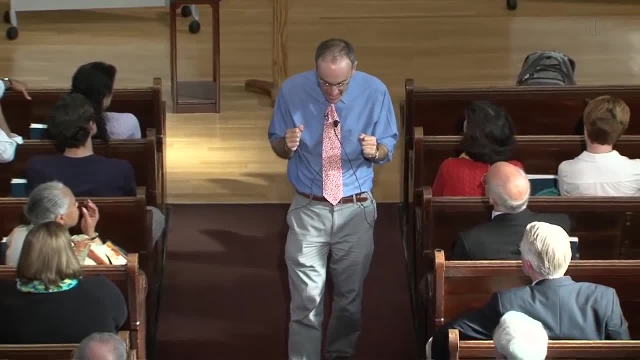 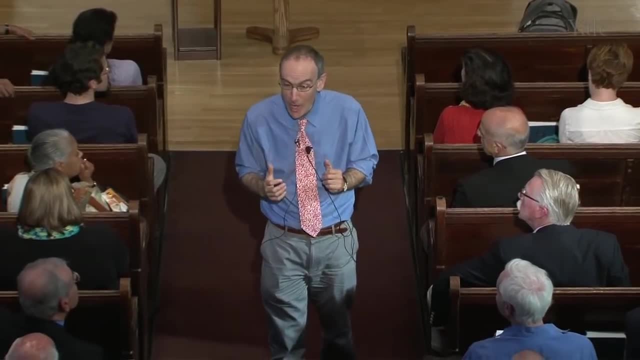 he's a wonderful dean of the graduate school and he steers the graduates in a wonderful way. Some of that is about incentives, that's the game theory part and your relationship with the graduate student, which is more the psychology part. So I'd say, Peter and I have the 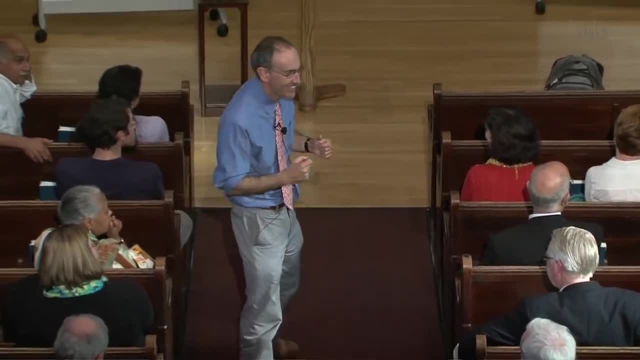 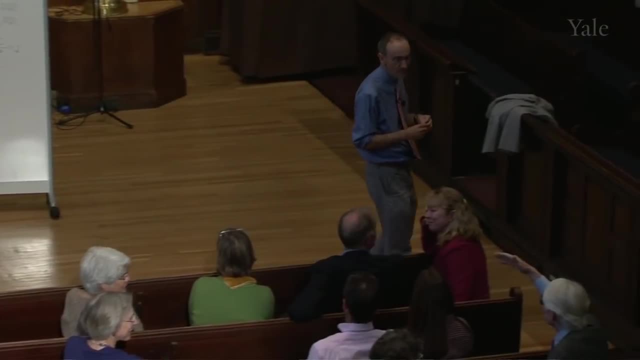 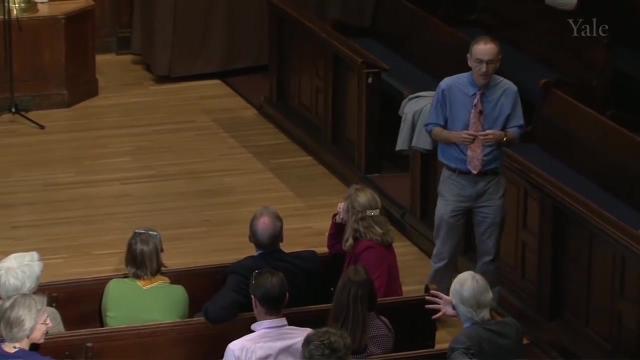 combined have the skills, but Peter has the more important skill, probably Ed. Well, in this example you know the shape of the skill curve that you play. But let's say I go in the game and I know my skill curve. 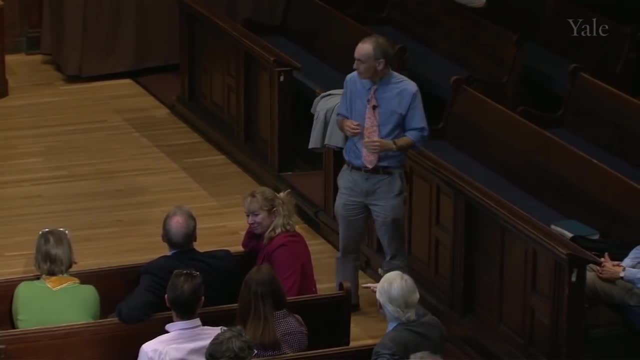 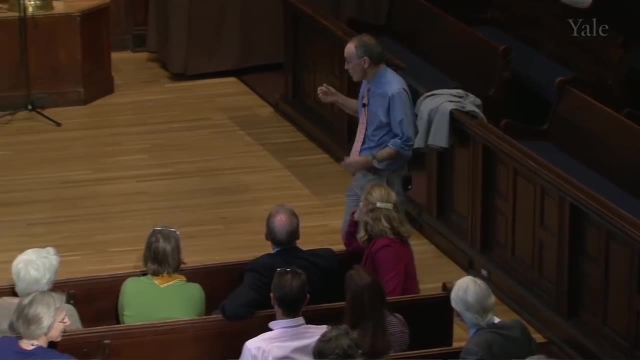 but I don't know my opponent's Now. my opponent may have a highly skilled curve, may have a poorly skilled curve. How do I develop the strategy? Good, good, So it's harder, but not impossible. So it's harder because now, 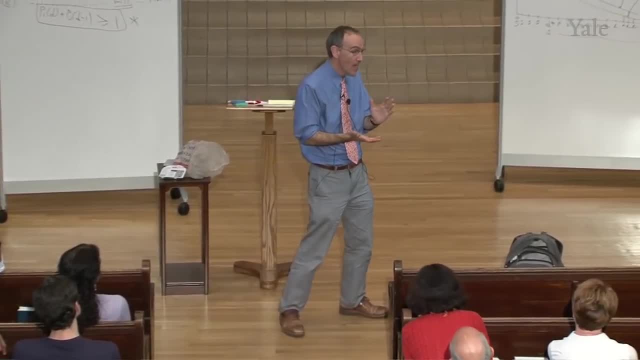 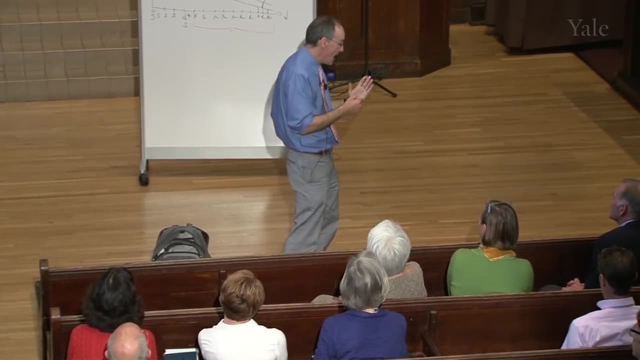 we'd have to think about the population of skill curves out there, And I want to be able to think of my opponent as being drawn, perhaps randomly drawn, from some population of skill curves, And so I'm going to have some. I'm going to 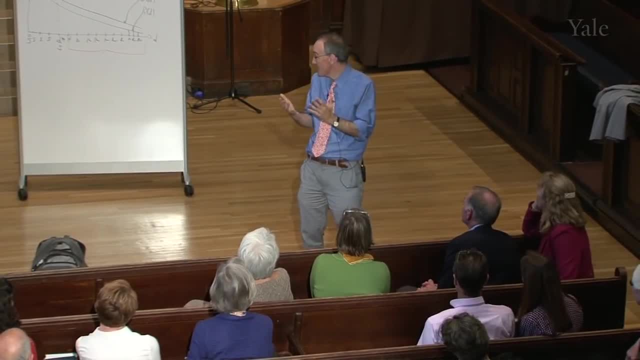 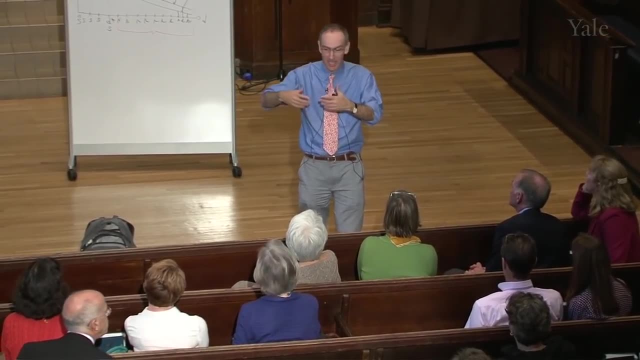 index each skill curve and I'm basically going to take expectations at every point in the game over those skill curves. So essentially the reason I didn't do it here is I need to carry a whole bunch of integrals And I'm taking distributions over. 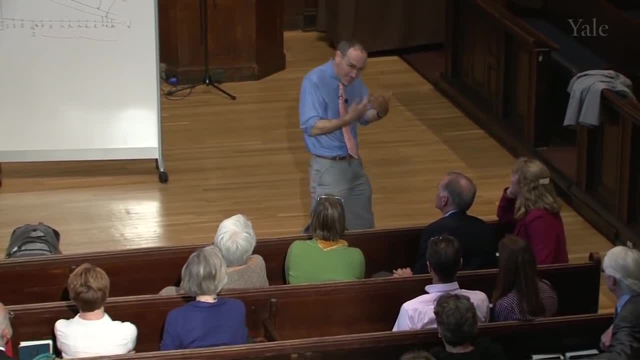 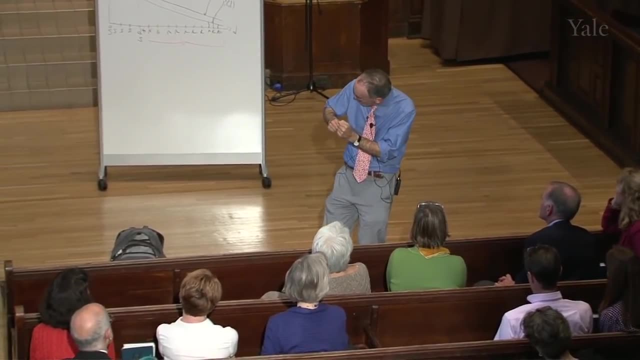 curves, which is a messy thing to try and do, But basically the basic idea is still the same. I'm going to carry some expectations around, because now I'm just now- it isn't that I know what the probability of this guy hitting tomorrow is. 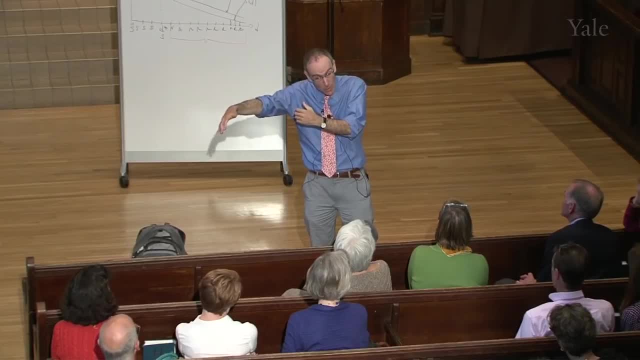 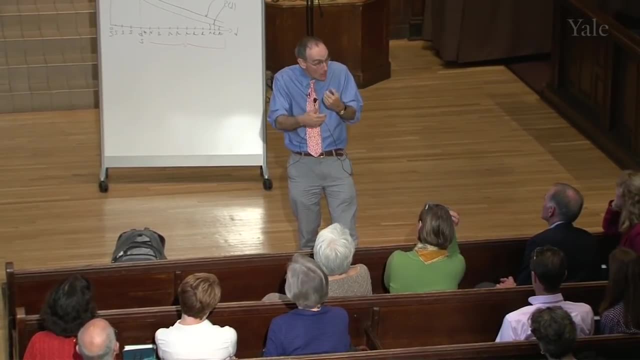 it's that I know only the expectation of that. I know with expectation what their probability of hitting is if they were to shoot tomorrow. So that means that the math is a little harder, but the basic idea of looking forward and working it out still runs through. 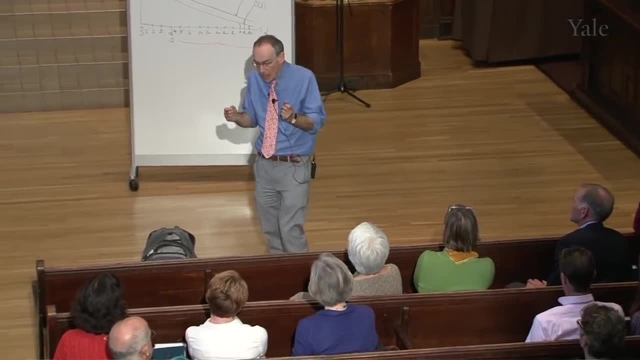 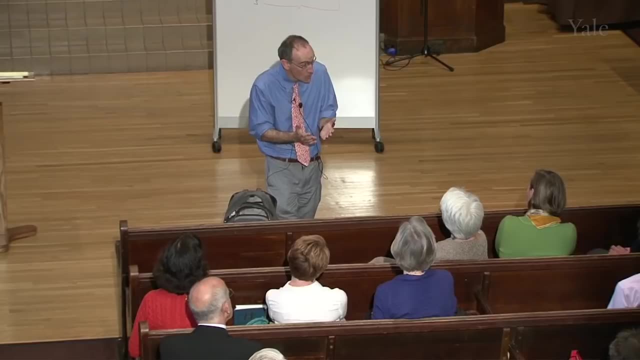 I'm underselling the math a little bit, because not only do I have to worry about the distribution of skills out there and worry about taking expectation over those skills, but that distribution is going to change as the game progresses. I'm going to be able to infer: 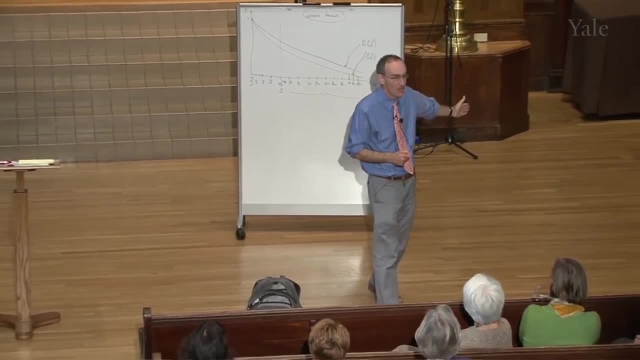 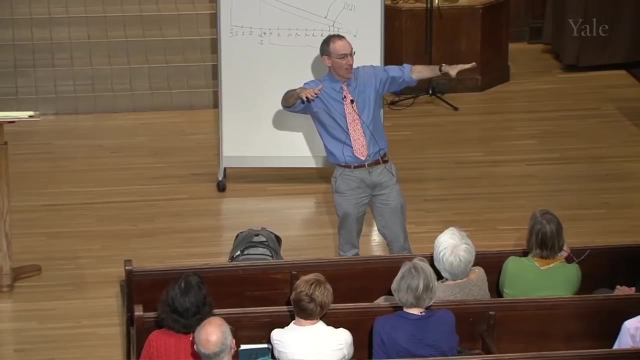 from the fact that the guy hasn't shot yet, that he's not as skilled as I thought he might be. So that distribution- you think about some bell shaped distribution of skills where these are the high skills and these are the low skills. 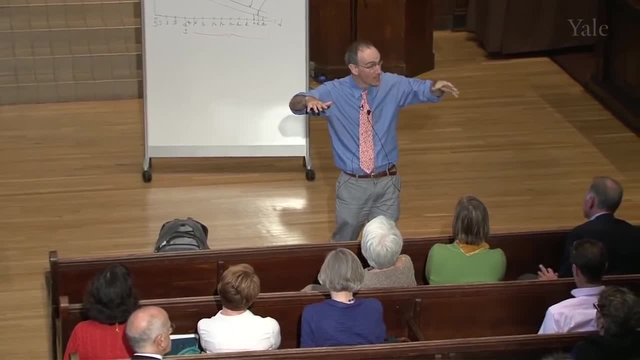 some of those high skills. I'm going to be able to conclude that they're not in the game as the game proceeds, when I see the guy not shoot. So I have to keep track of all that stuff. I have to do it based on updating on this distribution. 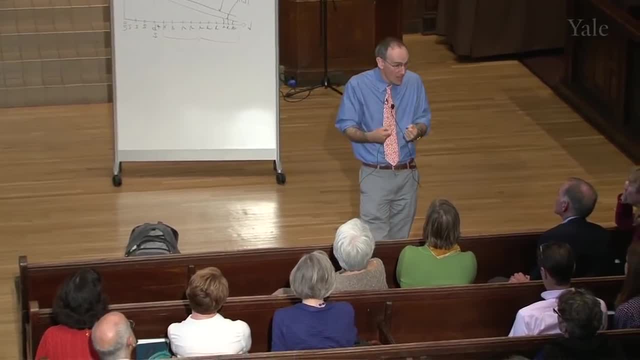 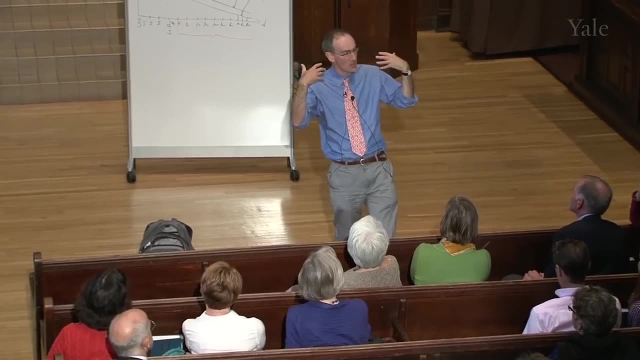 I have to get expectation and so on. but up to a lot of math, nice math, but up to a lot of math. the basic reasoning still goes through. The reason I didn't do it here is you can kind of hear there's a lot more math involved, but it's going to be okay. 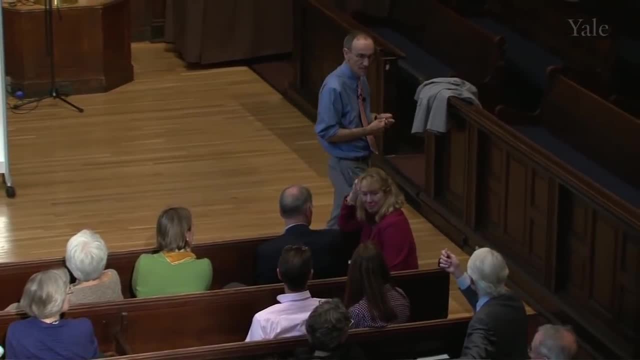 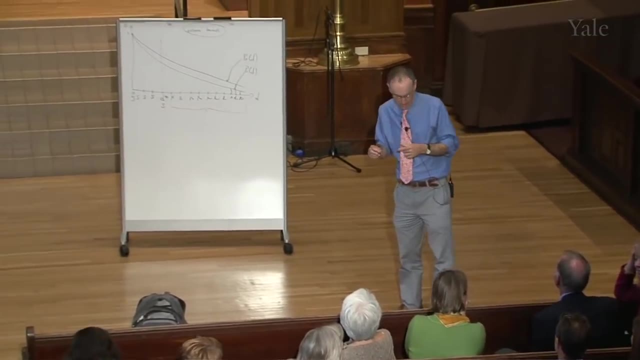 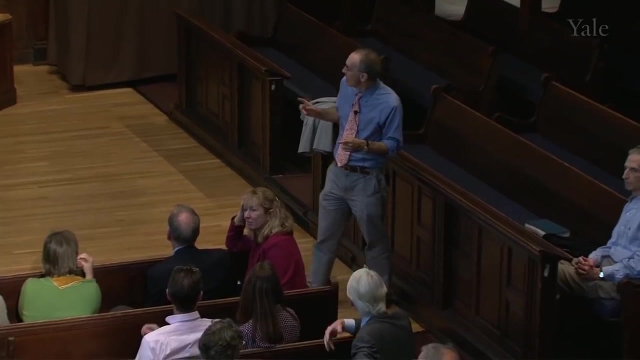 Well, doesn't it change if it's a life or death game? My objective is: don't lose, But let's say there's a greater monetary prize and if you win it's great. if you don't win it, eh, So doesn't that change my? 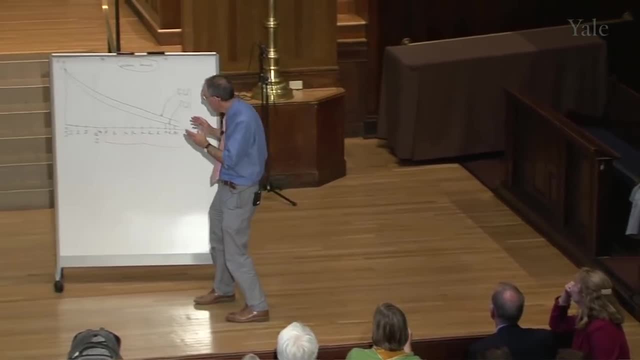 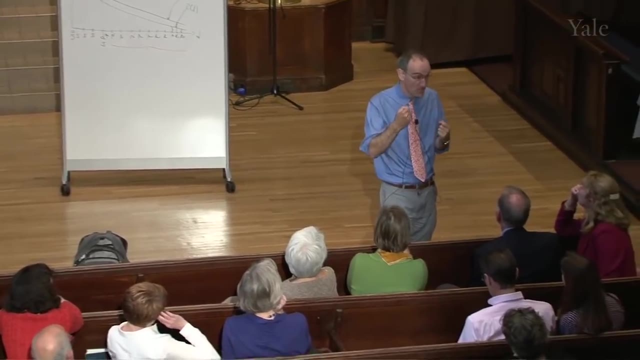 strategy. So that's an interesting point In this example: if there's just two monetary prizes, one for winning and one for losing, and the winning one is strictly better than the losing one, then it actually doesn't change the strategy In this simple game. But 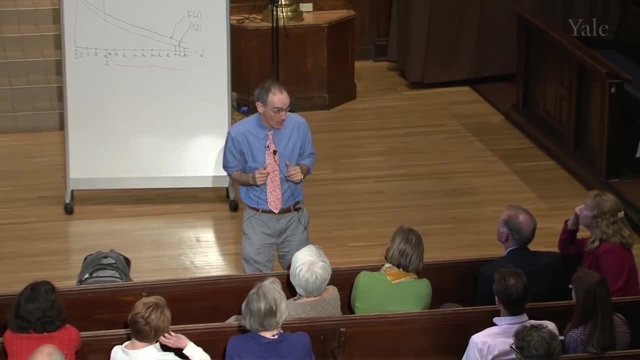 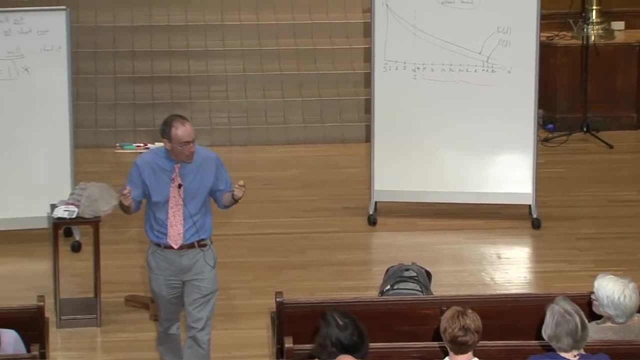 but that's too quick an answer. Imagine there's three outcomes. Imagine there's an outcome. so imagine the game is being played not exactly as we played it, with sequential moves, but with simultaneous moves. So in each period people simultaneously have to decide whether to throw or not. 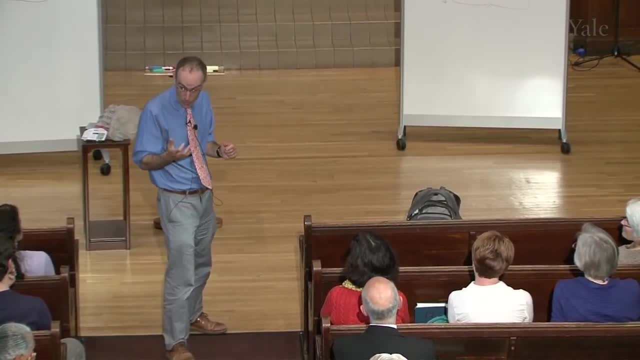 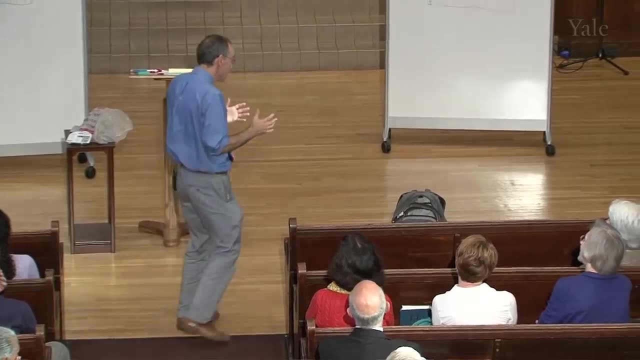 So now a third outcome is in the game. Now there's the outcome win, there's the outcome lose, and there's also the outcome both miss, Tie or draw. Now, now it's more complicated. Why is it more complicated? Because when there are three outcomes, 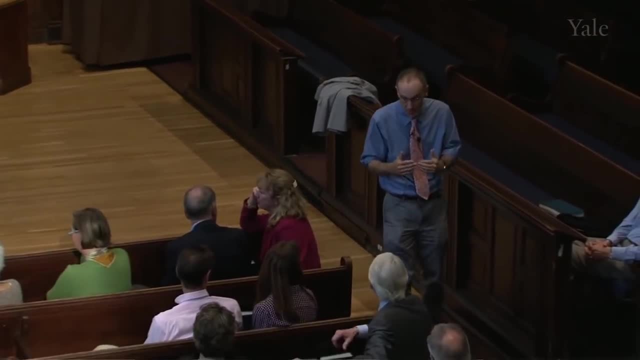 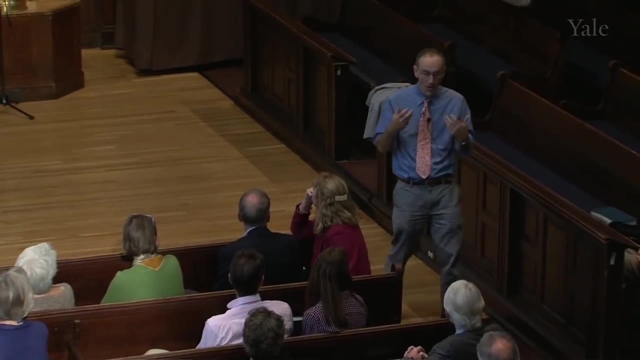 we have to take into account things like risk aversion, just as we would with many money outcomes. If there's only two monetary outcomes or two outcomes, this analysis is fine, But as soon as we go from two to three, we have to start worrying about risk aversion. 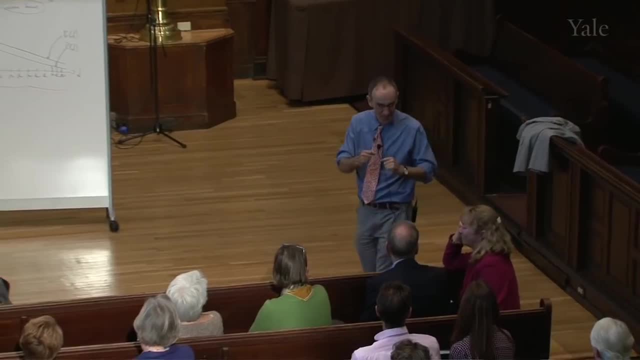 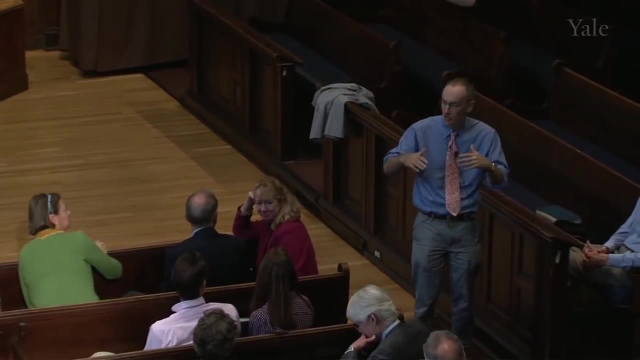 and things like it. Again kind of in David's territory, We have to do a little bit of what David does for a living to solve those things. But it's a great question. I should probably make this the last question because you will have other talks to go to. 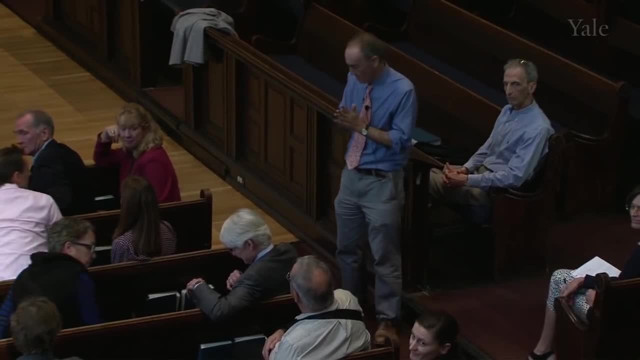 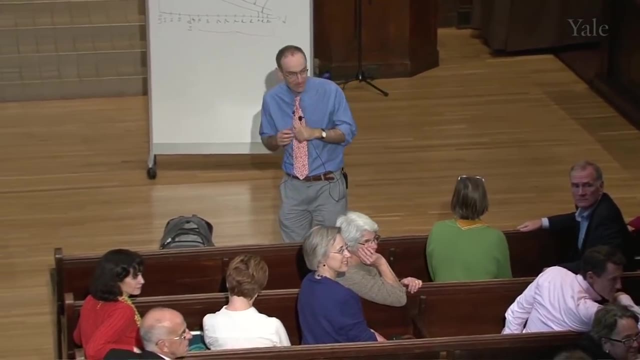 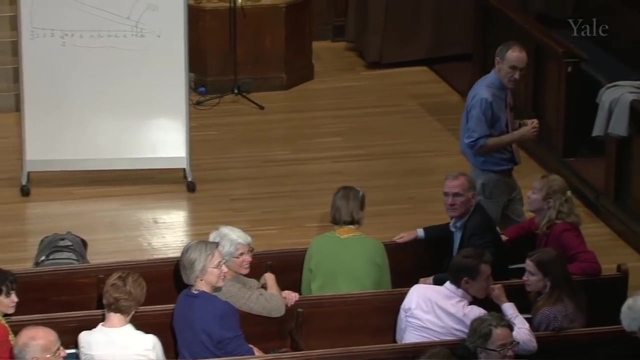 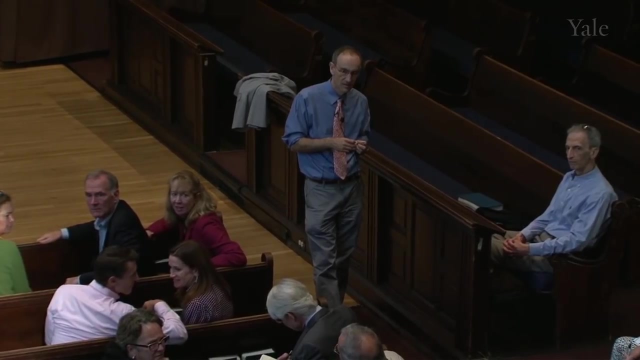 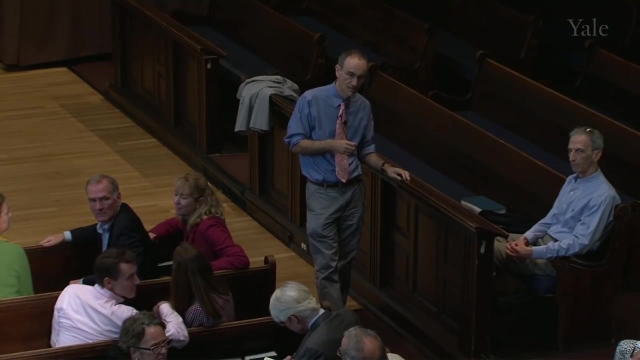 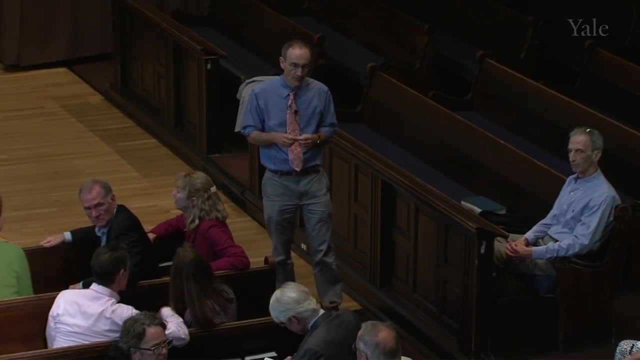 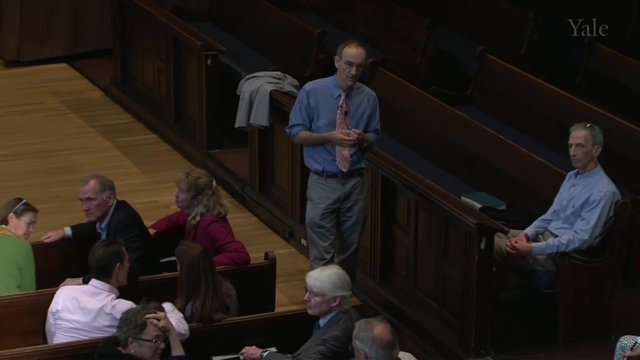 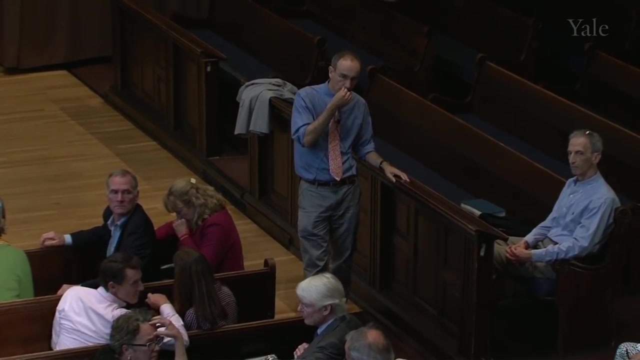 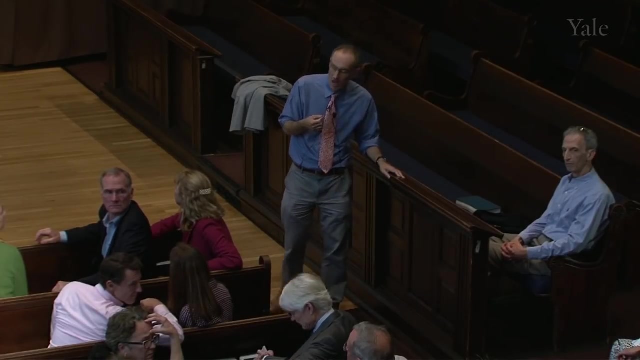 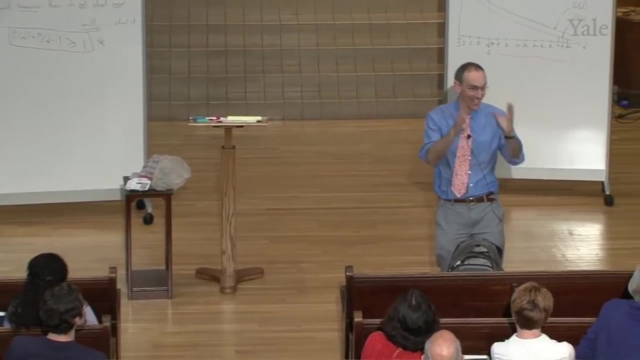 Yes, Yes, Yes, I agree with that. Of course, this is applied to biology. We're talking to a sociologist now, as you can hear, So I agree with that. So, by the way, today was high church because 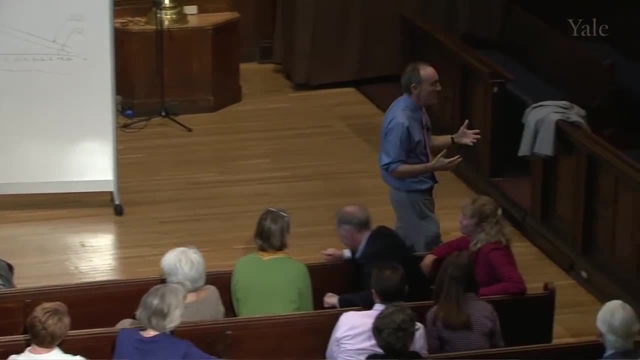 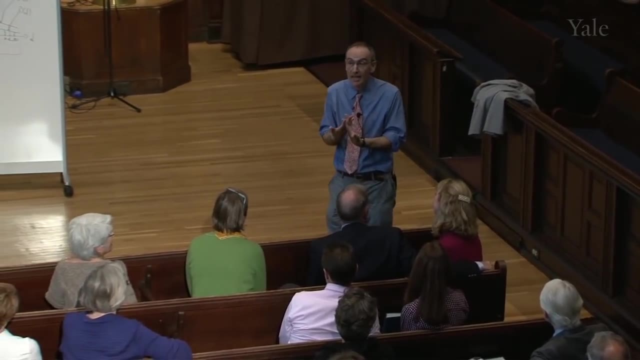 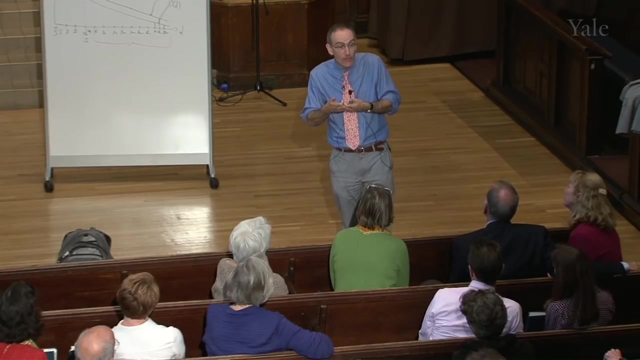 well, look around you. So what are we thinking? So what we're doing in mathematical economics, or the more mathy end of the social sciences, is trying to tease out our intuitions and trying to tease out how different assumptions lead to different conclusions. We are not. 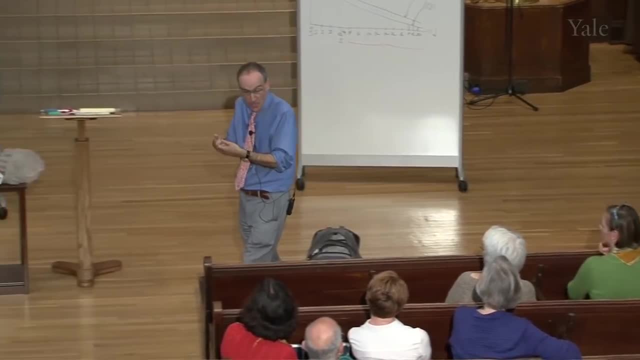 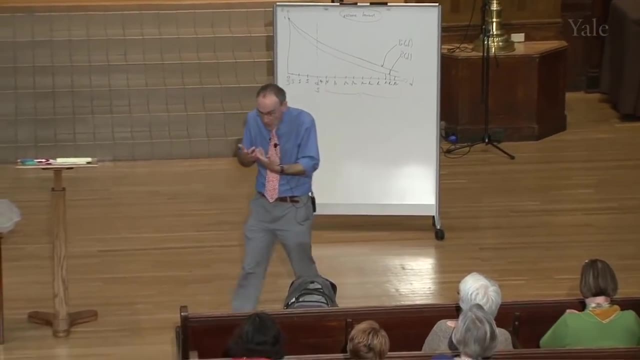 and you're absolutely right. we are not trying to say this is a tight prediction of what's going to happen. Some things will be pretty robust. This argument about dominance is pretty robust, But most arguments are not that robust, And one of the things we have to do in most 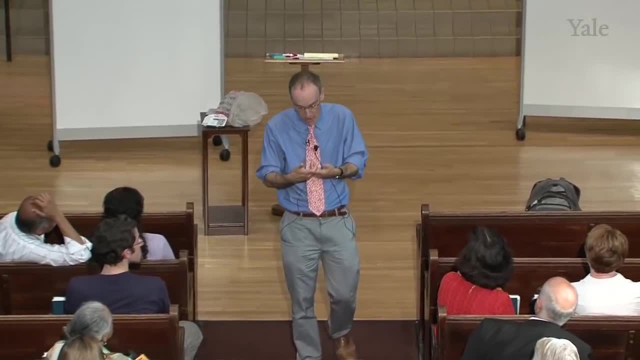 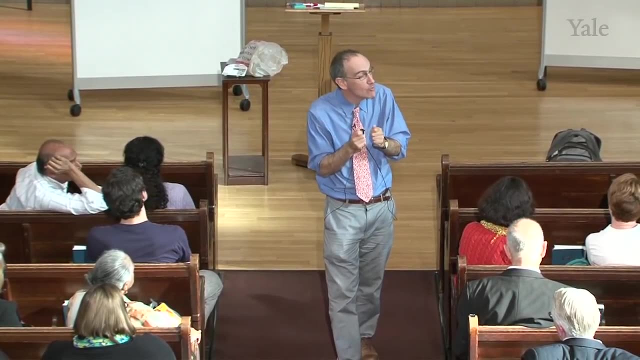 areas of theoretical economics, but the same is true in theoretical areas of sociology, is we need to tease out exactly what are the assumptions we're making. and what are the assumptions we're making? Would these results be robust to changing them? So the great thing. 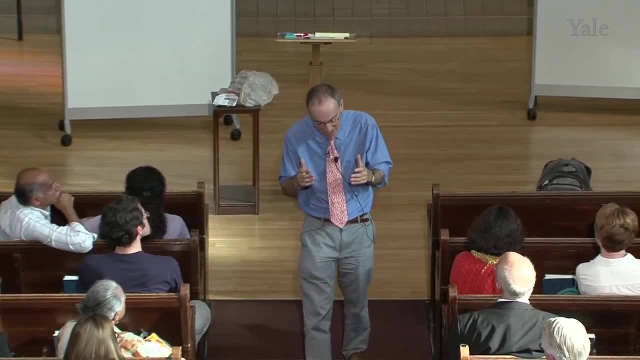 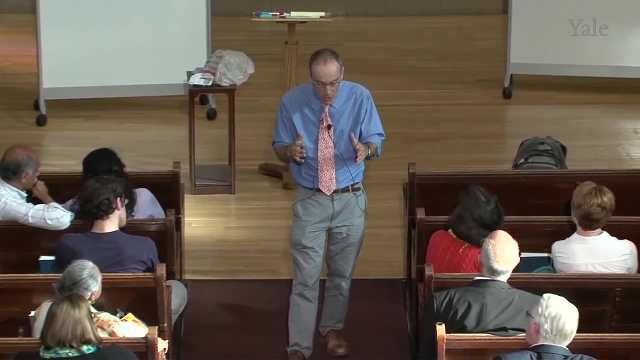 that, and this is not the most inspiring thing to end on, but I'll end on it despite that. the great thing about doing mathematical social sciences- which I guess is what I've done in my career- is it allows you to think through a kind of thought experiment, rather than an 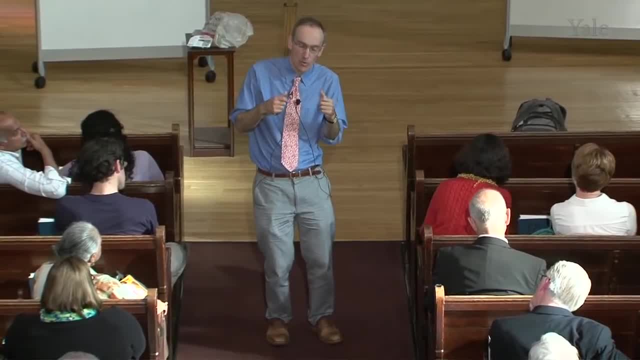 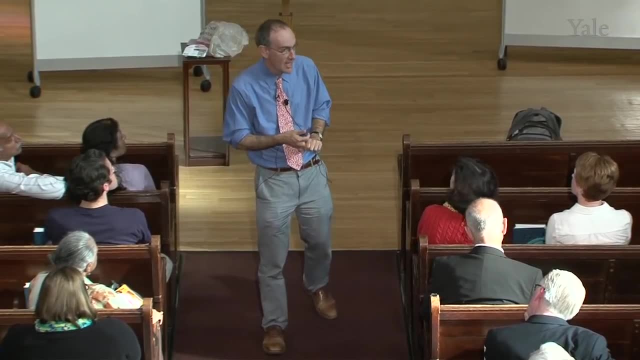 experiment. It says: I can't really. so I'll be having some discussion, let's say, with my wife, who's an English professor, and she'll say: yes, but you've assumed this, this and this, And it allows me to say: okay, you're right.